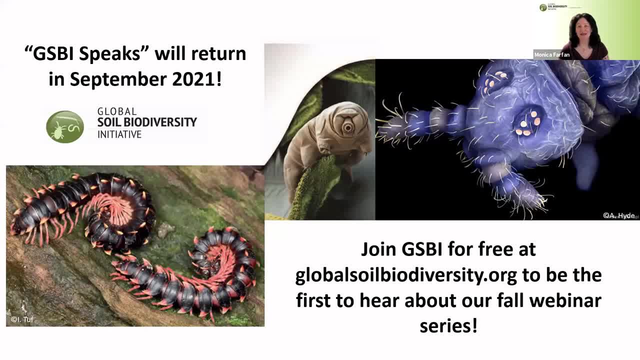 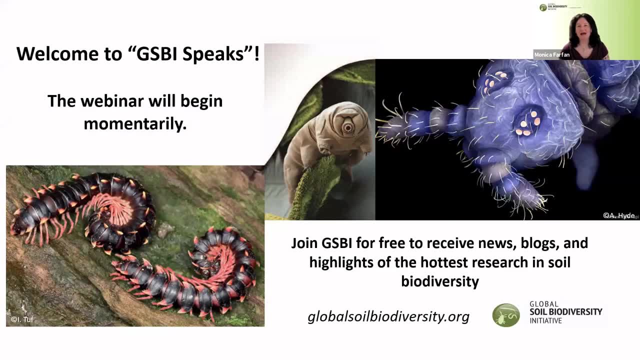 Good day and good evening. My name is Monica Farfan. I am the Executive Director of the Global Soil Biodiversity Initiative and welcome to GSBI Speaks. We have a wonderful program for you today, but first I wanted to go through a few housekeeping details. First of all, the GSBI. 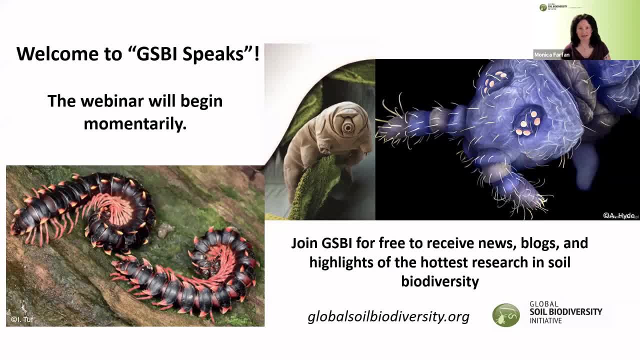 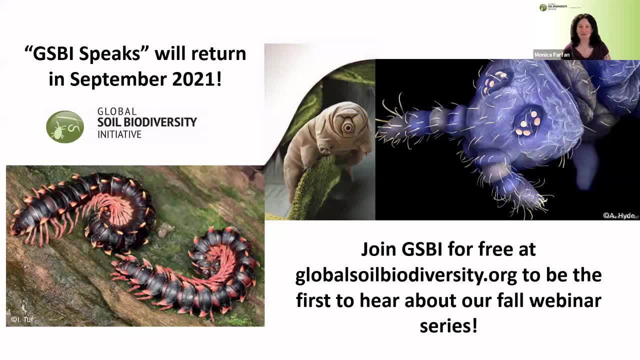 Speaks webinar series is going to be on hiatus for July and August. Please check our website for registration information for our September 2021 webinar. Today I would like to also share with you that this is being recorded and the recording will be available either later today. 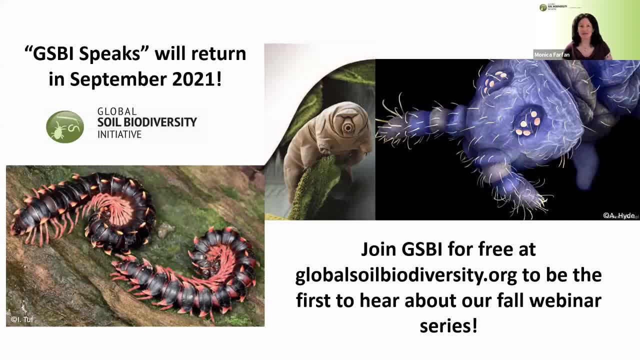 or tomorrow. If you registered for this webinar, you will receive an email regarding that. Next, I would like to let you know that we will be taking questions throughout the webinar. However, only in the discussion portion of this webinar, so the last hour- will those be addressed. 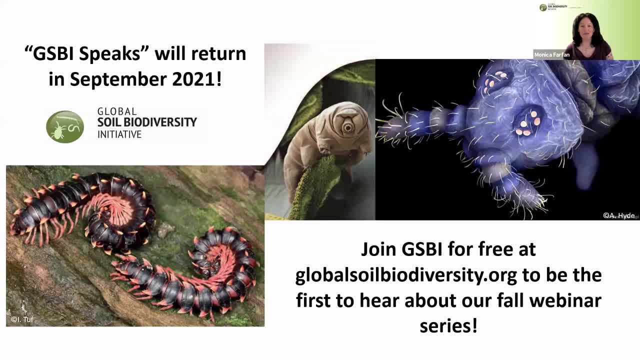 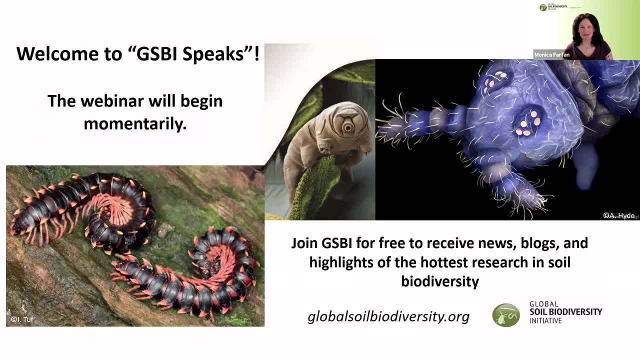 For those of you who would like to add a question to the queue, please use the Q&A box at the bottom of your screen. And now I would like to introduce our moderator today, Katie Suttig, from the University of Colorado. Katie is known for her work in ecological restoration. And please, Katie, now the floor is yours. 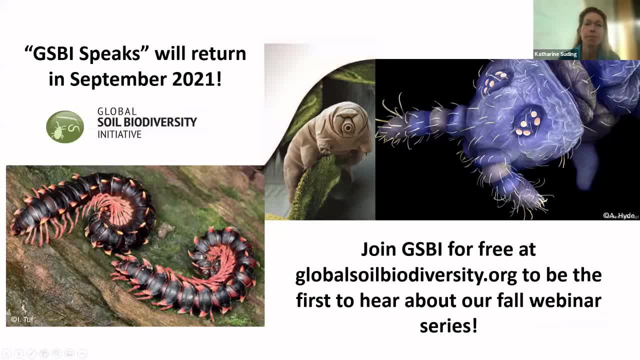 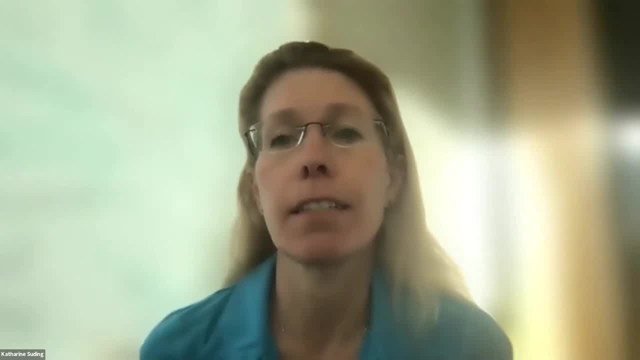 Great Thank you, Monica, and welcome everyone to our panel today on soil, biodiversity and ecosystem restoration. Great Thank you, Monica, and welcome everyone to our panel today on soil, biodiversity and ecosystem restoration. So, as Monica said, my name is Katie Suttig. 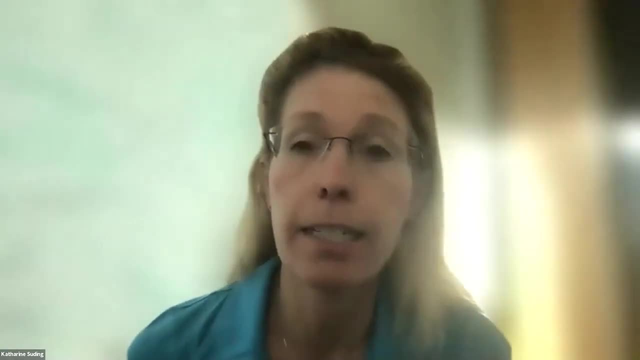 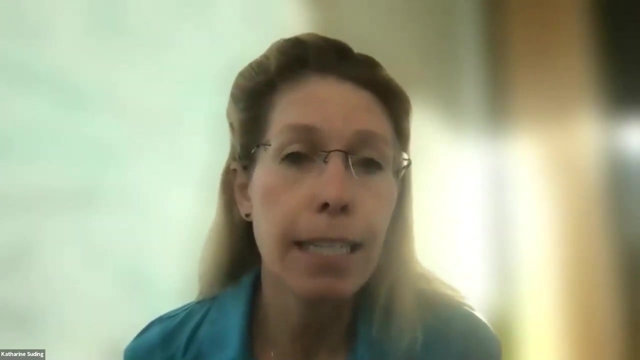 I'm a professor at University of Colorado and I will be moderating this next hour and a half And I want to start out just by pointing out some really exciting news, and I hope everyone was aware of it. But this Saturday the UN Chief, Antonio Guterres, kicked off the UN Decade of Ecosystem Restoration. 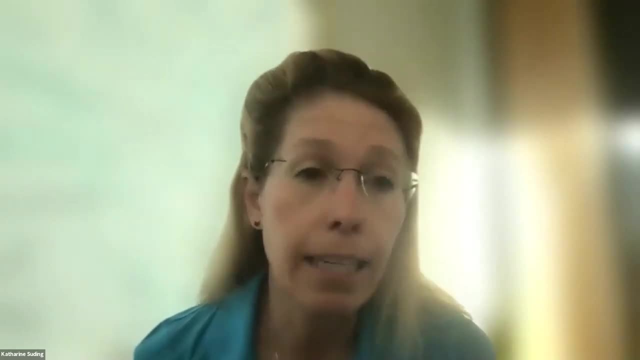 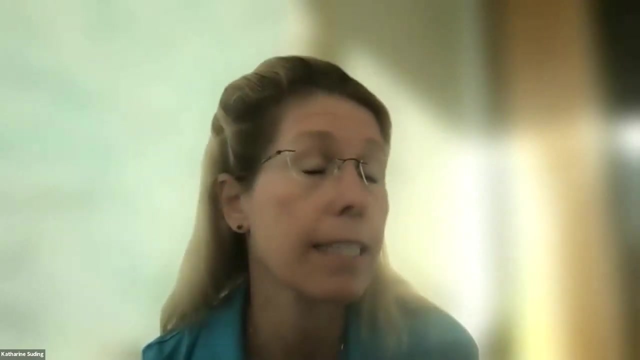 But this Saturday the UN Chief, Antonio Guterres, kicked off the UN Decade of Ecosystem Restoration And in his speech he pointed out that it's the next 10 years that are our final chance to avert climate catastrophe, turn back a deadly tide of pollution and end species loss. 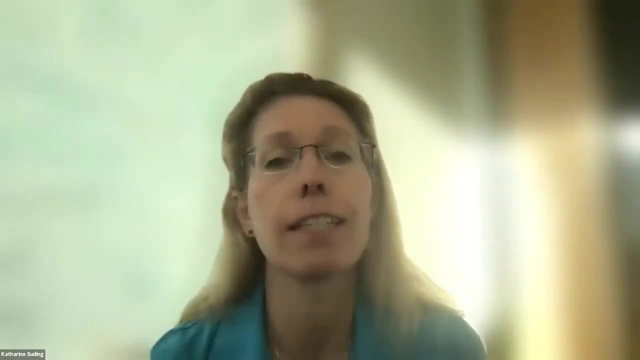 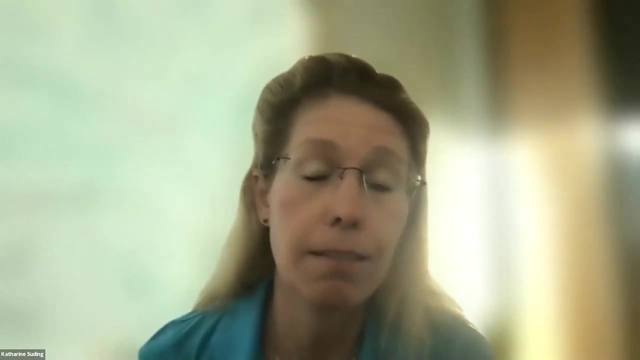 So they are putting a huge, huge emphasis on the next 10 years and on ecosystem restoration. So we are right right now starting the decade of ecosystem restoration, So this panel is super timely And, alongside forests and oceans and deserts, soils are really taking a center stage. For instance, the UN Convention on Combating Desertification has set the ambitious target to restore 100 million hectares of degraded land Soil capture around 250 million tons of atmospheric carbon in the next 10 years. So yeah, this is big. 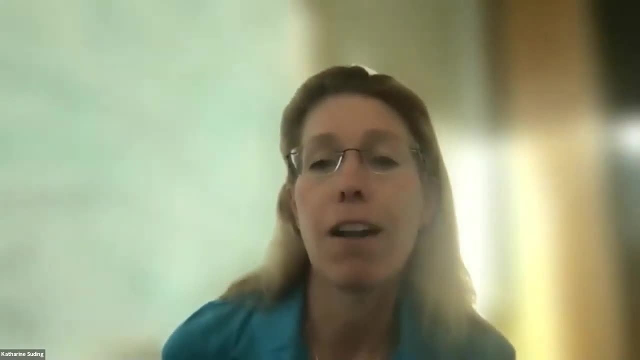 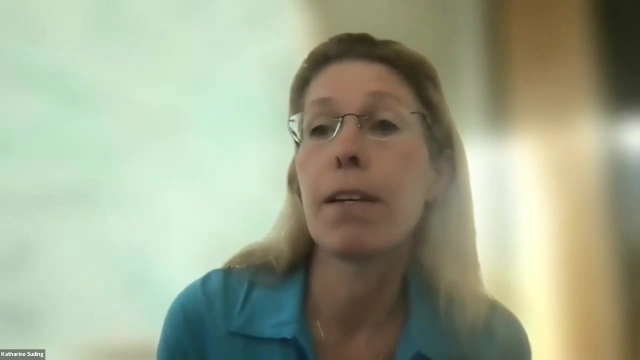 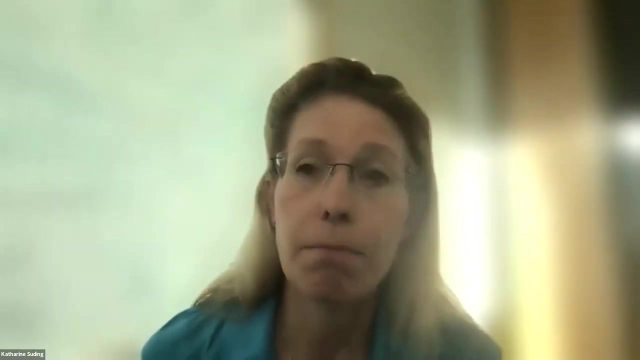 And it all, at least in my opinion, revolves around soil And by why I think everyone is really super excited about this ambition. you know, it's a little nerve wracking as well, And I just want to start with a little antidote. 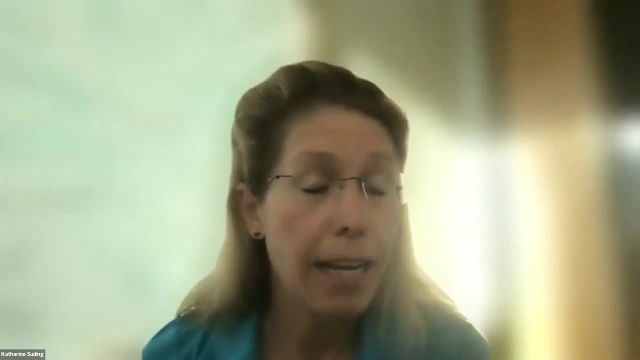 About my personal work. So when I have looked into issues of restoration time and time again, I found that when a system is stuck, when it's really really seems difficult to guide recovery and the way we're pulling our hair out about what to do, you know, the key component almost always- at least in my case- is the soil community. 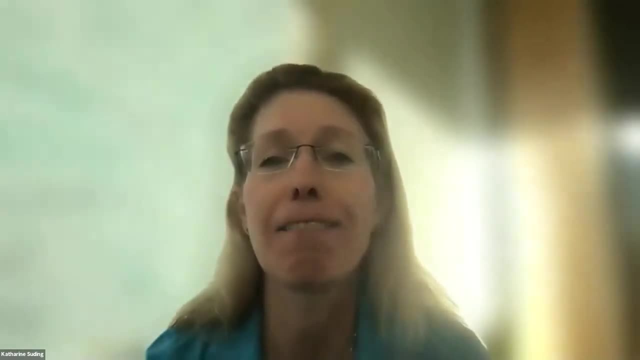 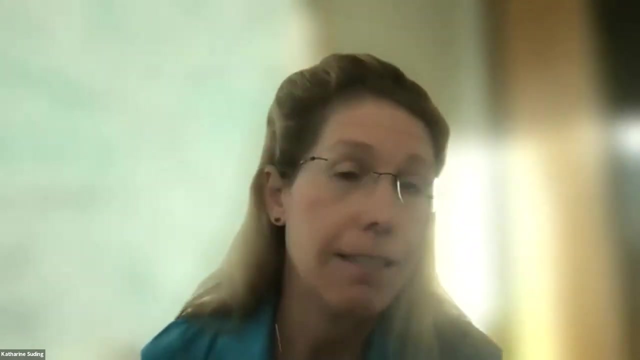 And it rules many, if not all, of the plant recovery And ecosystem dynamics in these semi-arid grasslands and prairie systems that I work with. So it really is key And so I think it is very much a key consideration in these next 10 years if we are going to meet these ambitious goals. 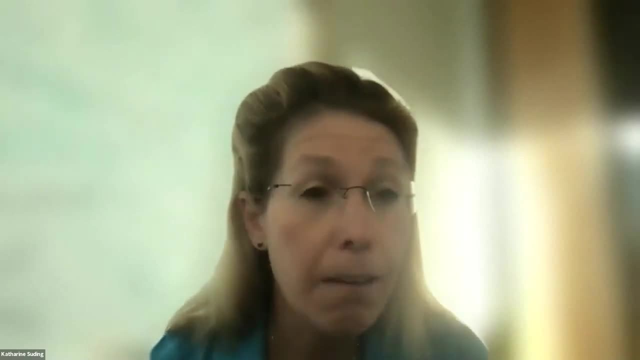 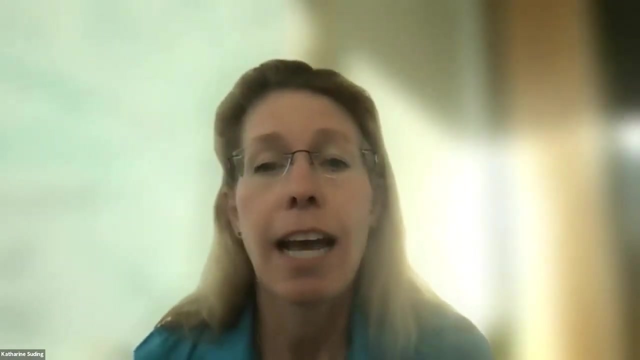 But we also often hit the wall once we pinpoint that it's the soil communities that are key to recovery and ecosystem dynamics. But how are we going to? what are we going to do? what are we going to do to address this limitation and restore soil biodiversity, get the importance and balance back into the system? 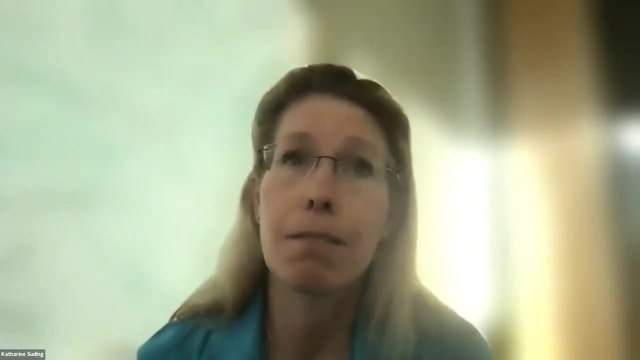 And this isn't really as simple as, for instance, just planting a tree. It is a super complex problem And in many cases I've walked away scratching my head and not being able to provide great solutions to the managers and policymakers that I'm working with. For instance- just one example of this- the native grasses in California can persist and resist invasion really well with a lot of environmental threats and pollution, drought, so on. But when they're removed and we try to get them back- so try to restore them in a system- we really have very little luck because the symbionts, the microbial symbionts in the soil are not there. 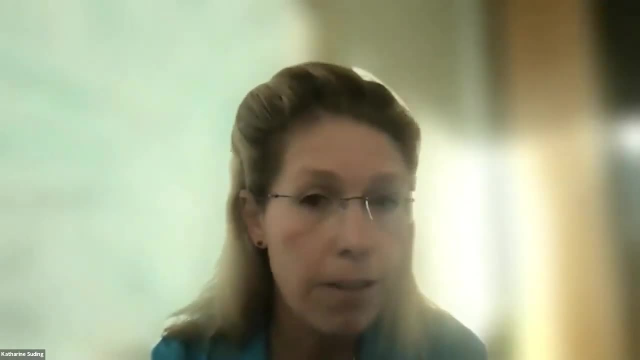 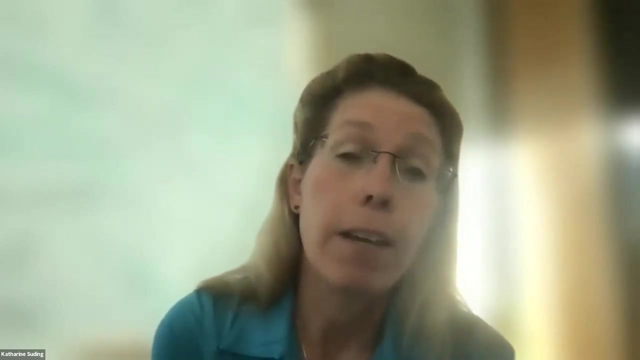 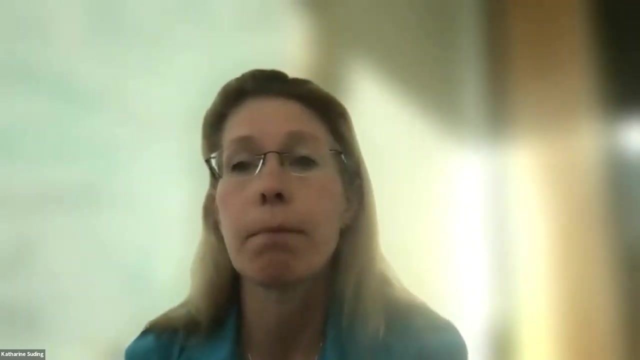 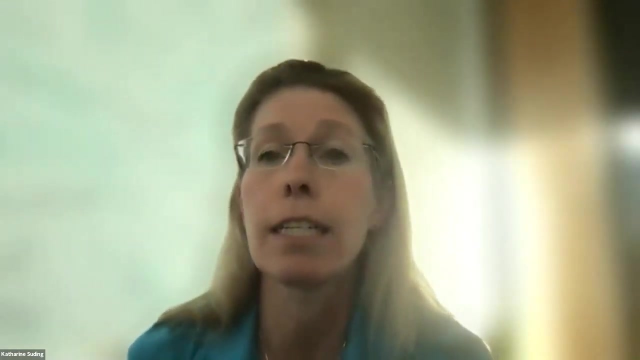 And we try time and time again. we try different things, try all these ways of trying to restore the soil community, And it is very, very difficult to get them back in the system. So the fabulous thing about where we are at in this research about soil biodiversity and restoration is that we're learning so much about these linkages between the soil community and recovery and restoration, as well as we're breaking down these walls about how to restore soil biodiversity. 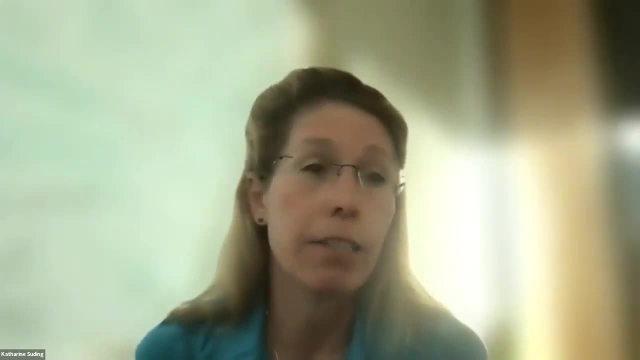 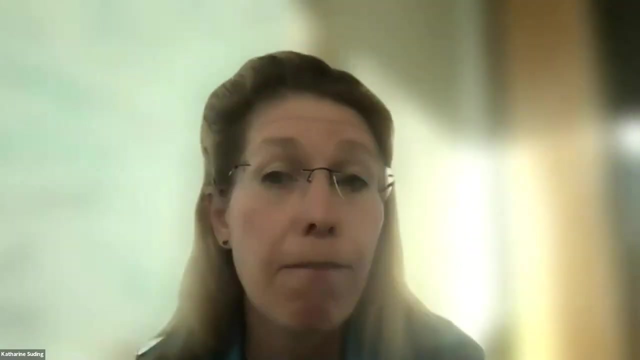 And we're also learning how to use that knowledge and really apply it to restoration actions. So there's a lot, a lot of exciting breakthroughs right now. So right now, I'm super excited to hear from four of my favorite soil restoration scientists. 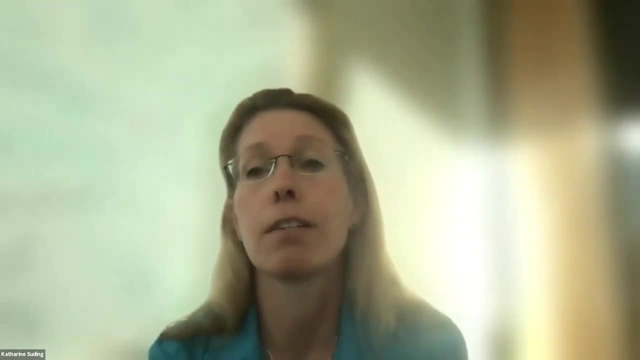 And together talk about soil, restoring the soil, the role of millions of microbial and animal species that live in soils, and restoring an entire ecosystem. So we are so fortunate to have these four scientists. They're making a change in our soil And we're working really hard to get them back in the system. 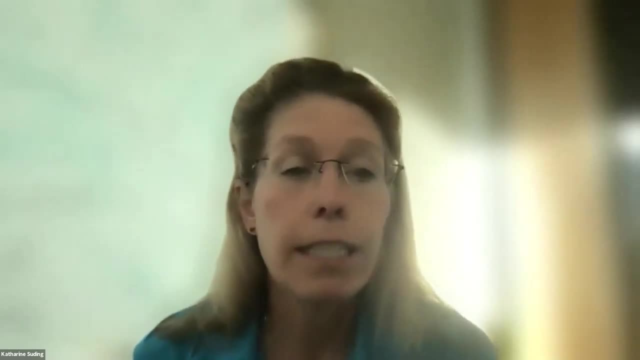 So they're working really hard to get them back in the system with us today, And so I'm going to briefly introduce each one, And then I'm going to ask them to give a short introduction for the first bit of our session today. 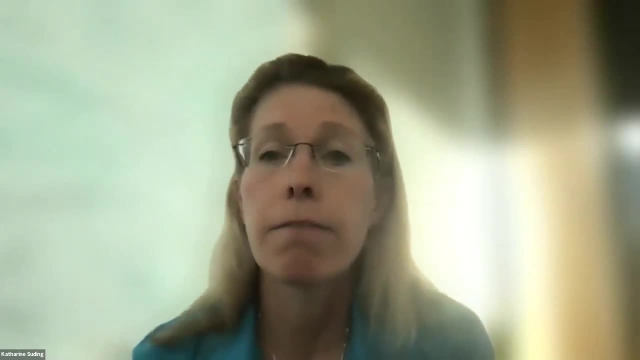 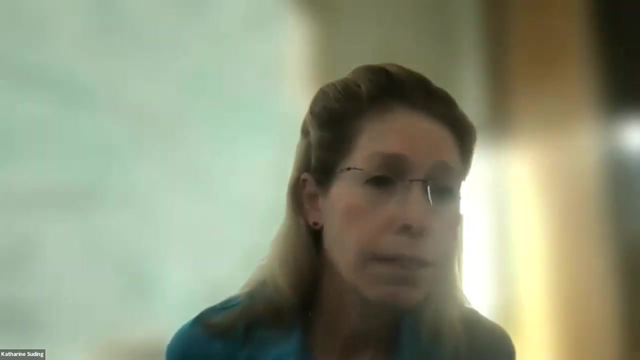 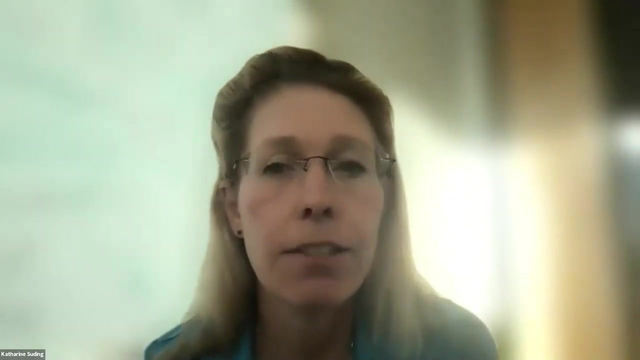 So we are fortunate to have Sarah Baer from the University of Kansas. So, Sarah, Susana Rodriguez Echeverria from University Comba, Portugal, Susana, Hello. We have Jasper Wubbs from ETH Zurich- Hi everyone. And lastly, we have Raul Ochoa from University of Cadiz, in Spain. Raul, 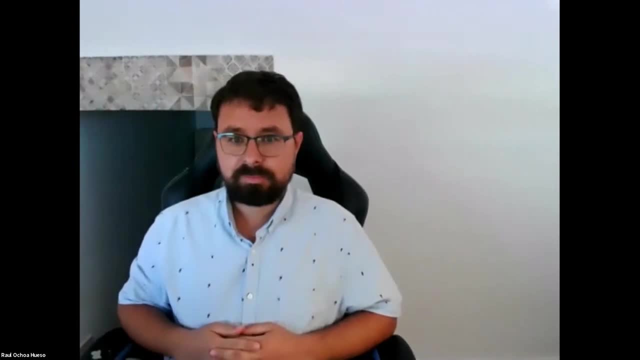 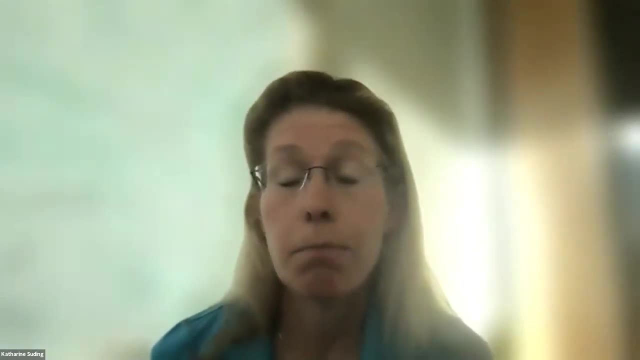 We have asked all panelists to talk about their amazing work on the subject. They bring a huge diversity of perspectives and expertise, As well as looking forward about our major gaps and understanding what can be done and how we can move forward, particularly in these next 10 years. We will hear from each and we are not going to stop for questions in 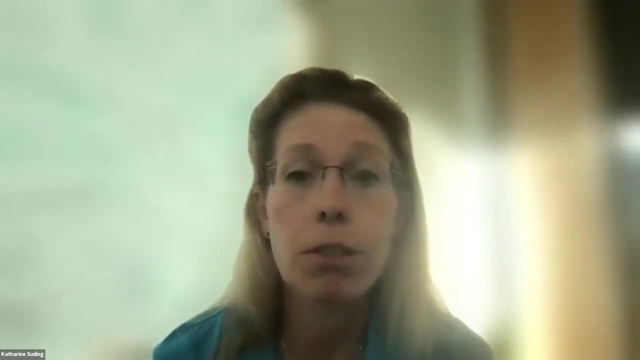 between. We will hear from each and we are not going to stop for questions in between. We will hear from each and we are not going to stop for questions in between, And then we will open it up for questions as a group. So please type them in the question and answer section of the. 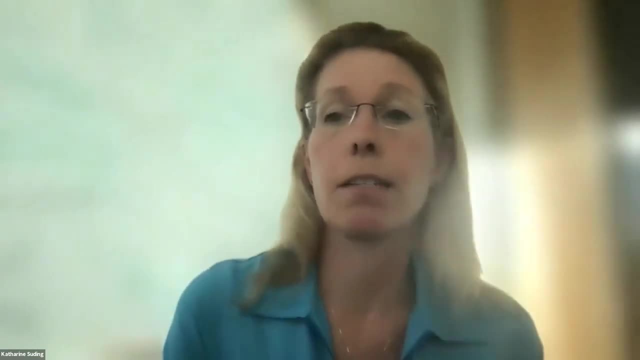 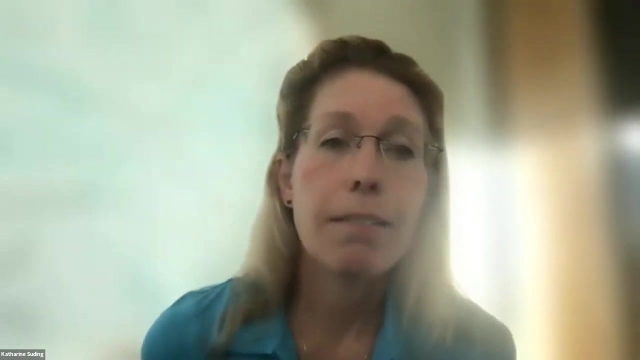 Zoom And I will try to get to as many as possible. So I'm pleased to turn this over to Sarah for her to talk about her research. Thank you, Sarah. Sarah Baer, University of Kansas. University of Kansas, College of Agricultural and Environmental. 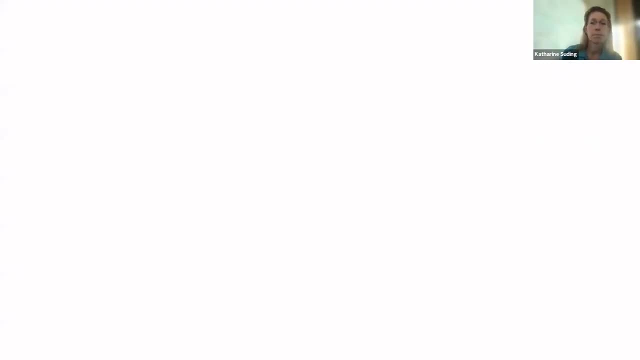 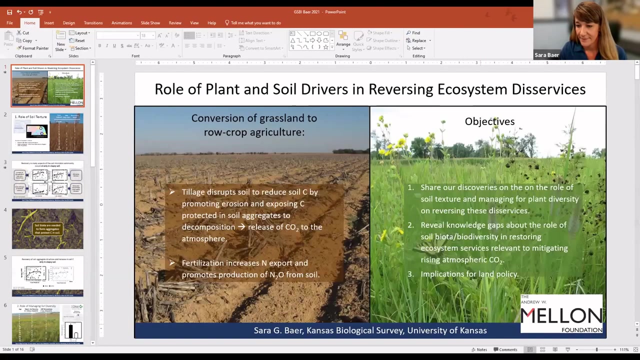 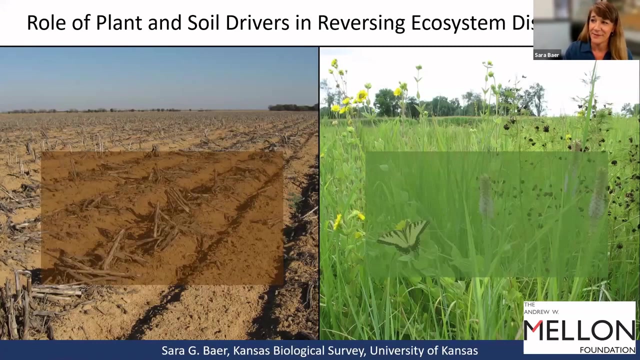 Science and Technology Services, MA. How can I learn more? Sarah Baer, University of Kansas. University of Kansas. University of Kansas, College of Agricultural and Environmental Science and Technology Services. So it should start soon. Well, thanks for inviting me to present at this very timely Forum The Soil, Biodiversity and. 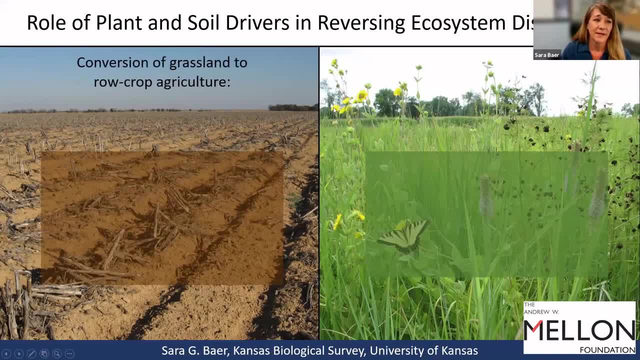 Ecological Restoration. We are very curious to hear yourومani nuts. when I was in LA I met all restoration. Much of my research has focused on the role of plant communities and soil properties as drivers in reversing ecosystem disservices caused by agriculture. So when grassland is 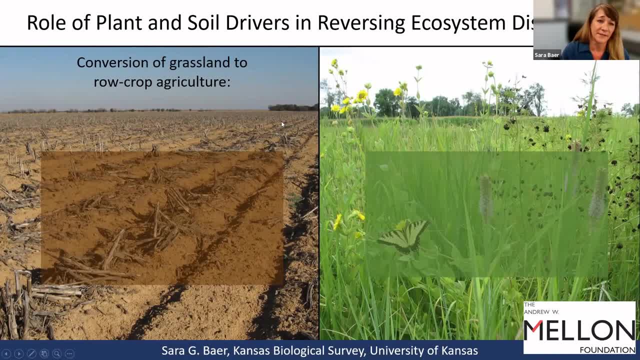 converted to row crop agriculture. numerous disservices result When the soil is tilled. it disrupts the soil and reduces soil carbon by promoting erosion and exposing carbon that was protected in soil aggregates to decomposition, And this results in a release of that carbon. 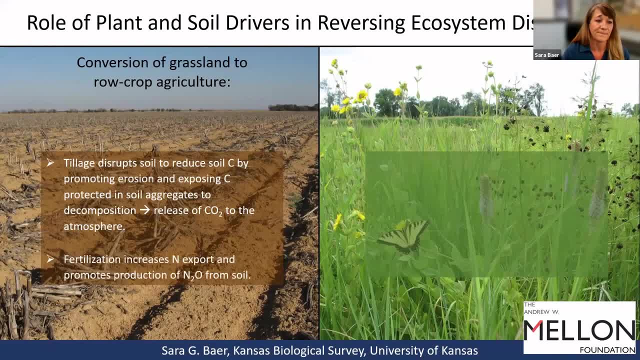 as carbon dioxide to the atmosphere. Furthermore, when we fertilize these soils, there's an increase in nitrogen export from the system, and fertilization also promotes the production of nitrogen. So when we fertilize these soils, there's an increase in nitrogen. 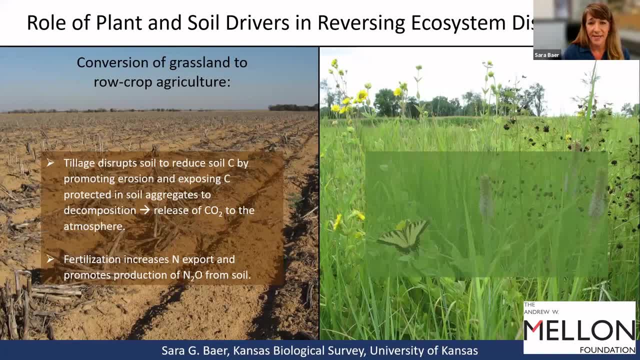 from soil, which is a more potent greenhouse gas than carbon dioxide. So today I'm excited to share with you some of our discoveries on the role of soil texture and managing for plant diversity, on reversing these ecosystem disservices, And I'll talk about knowledge gaps that we've learned. 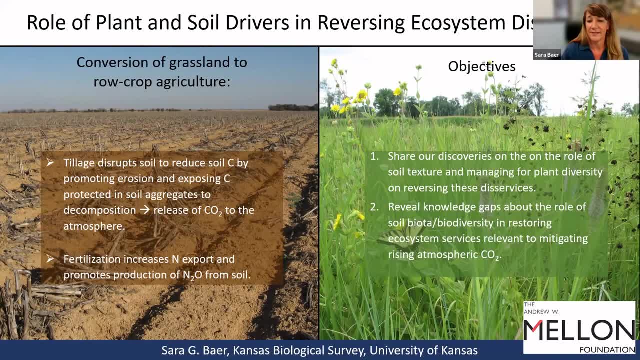 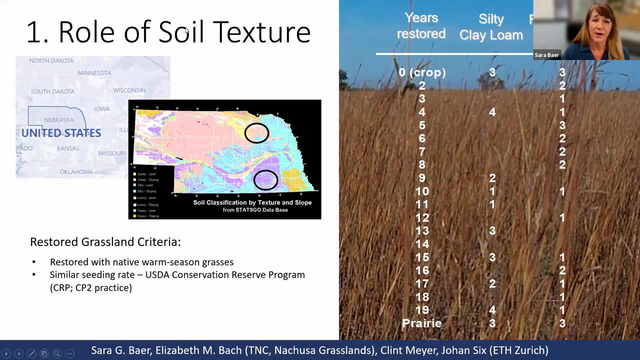 about the role of soil biota and restoring ecosystem services that are relevant to mitigating climate change And some implications for land policy. So my colleagues and I have studied the role of soil texture on soil recovery in Nebraska. Here we used many grasslands that were restored with native warm season grasses but existed on two. 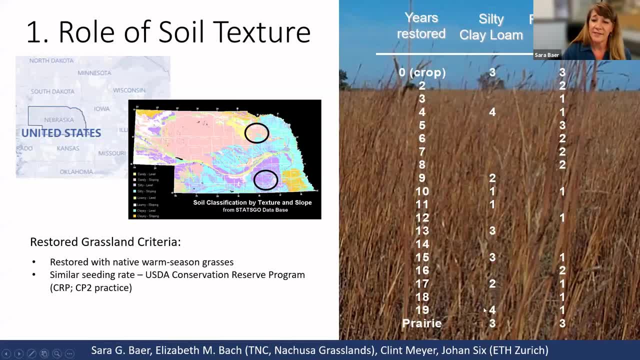 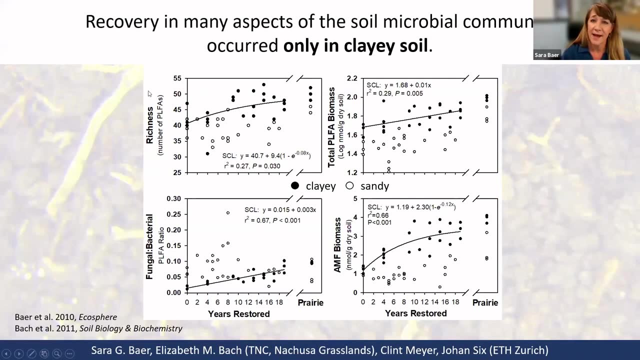 very different soil types, So within each soil type we sampled many fields that were restored for different periods of time in order to model below ground recovery, And what we found was recovery in many aspects of the soil microbial community, Recovery in the number of phospholipid. 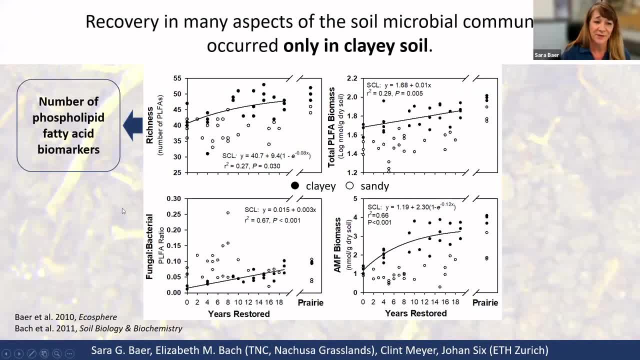 fatty acid biomarkers that are extremely coarse measure of microbial diversity, recovery of microbial biomass in the soil, the ratio of fungal to bacterial biomass in the soil and the recovery of our muscular mycorrhizae fungi biomass in the soil. But all of these patterns only. 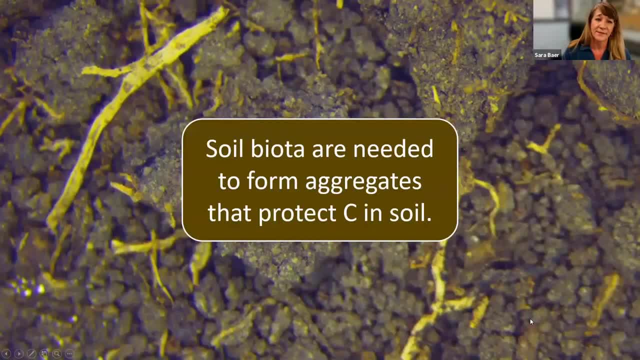 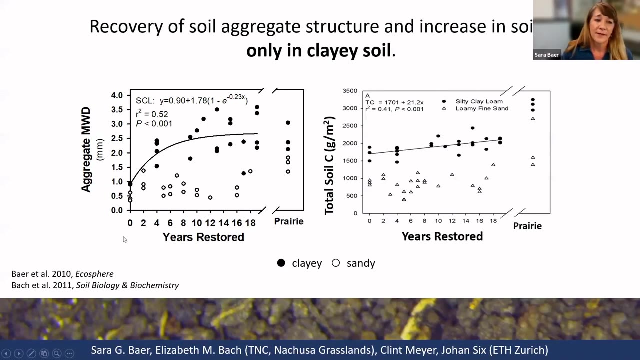 occurring in the clay soil and not in the sandy soil, And so those soil biota are required in the soil And their recovery to form these aggregates that ultimately protect carbon in the soil, And so what we saw was only an increase in recovery, is the growth of macroeconomic biomass by foliar 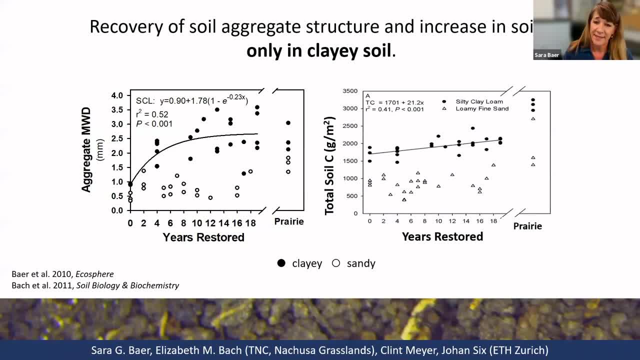 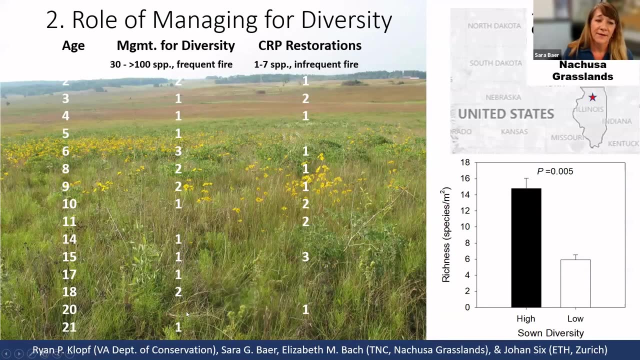 in this aggregate structure happening in the clay soil and consequently, we only observed an accrual of carbon occurring in these clay soils. We used a different pair of restored grassland chronosequences to look at the role of managing for plant diversity on soil recovery, as 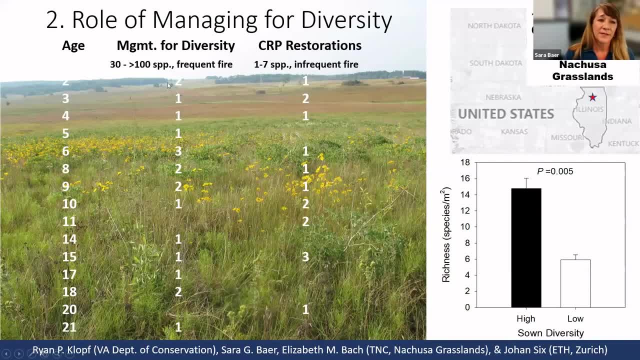 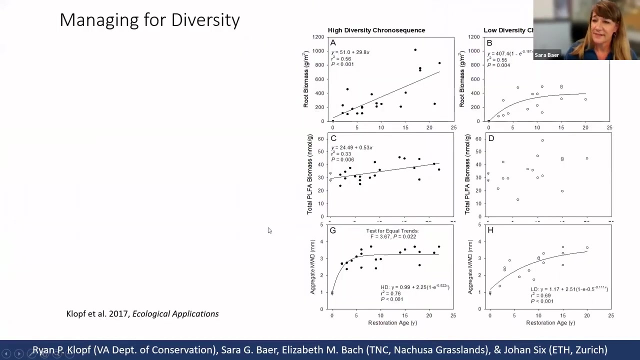 well, And here we did this in Illinois, where we used again a sequence of fields restored for different ages that were restored with many species and managed frequently with fire, and compared that sequence to fields that were restored with far fewer species and managed with infrequent fire. And so results from this study showed that managing for diversity results in a 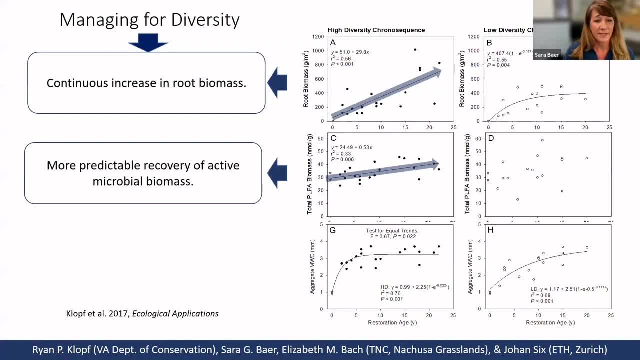 continuous increase in plant diversity, And so we used a different pair of droughts over the course of this study, which shows that the unfair age of the soil by over 80% in the two or three years, And that's when the soil was disturbingly damaged. So we were able. 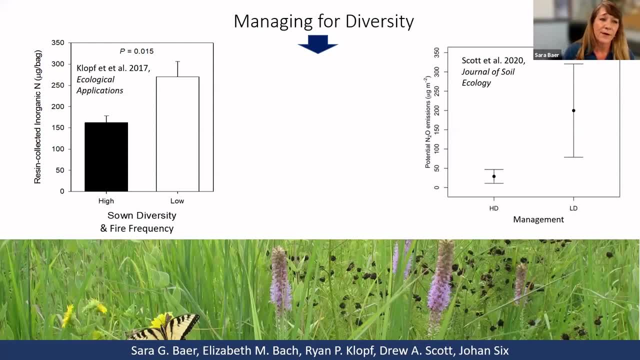 to see a decrease in root biomass, a more predictable recovery of the active microbial biomass and a faster recovery of that soil aggregate structure. Managing for diversity also reduced the amount of inorganic nitrogen available to be lost from the ecosystem through leaching and less potential nitrous oxide flux from soil when managed for high diversity. 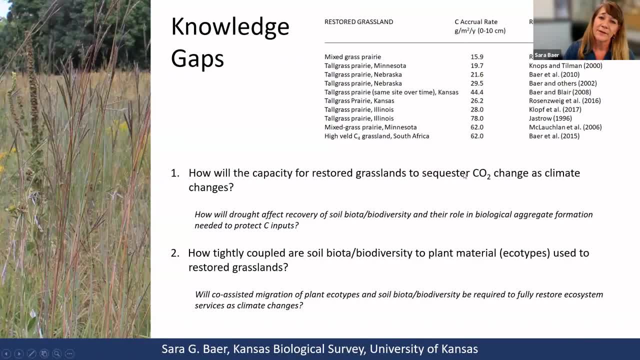 So when we look across numerous studies that have quantified carbon accrual rates in cropland restored with warm season grasses, we see large variation in the recovery rates of carbon, And so this indicates that we don't know all of the factors that are contributing to. 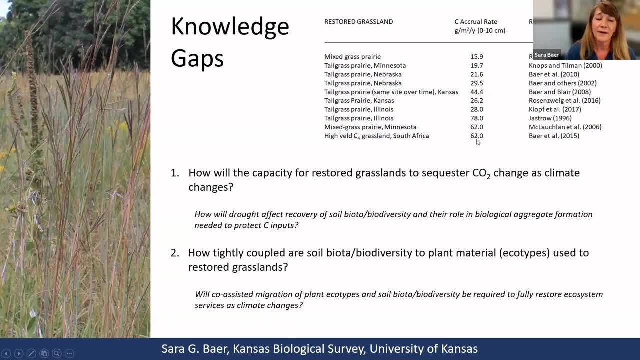 the capacity for which they can accrue carbon. Then other questions emerge, like: how will the capacity for restored grasslands to sequester carbon change as climate changes? For example, how will drought affect the recovery of soil biota and their critical role in forming? 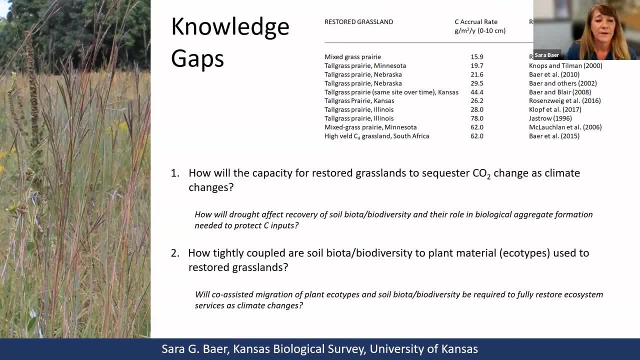 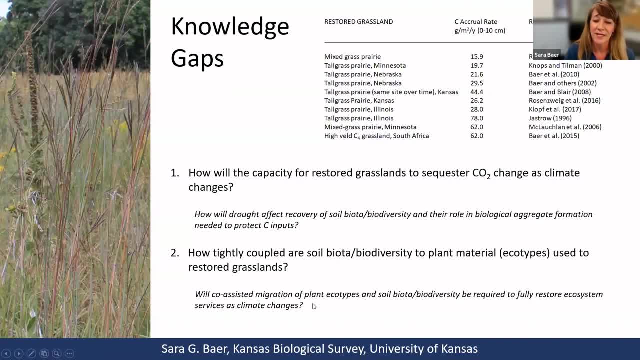 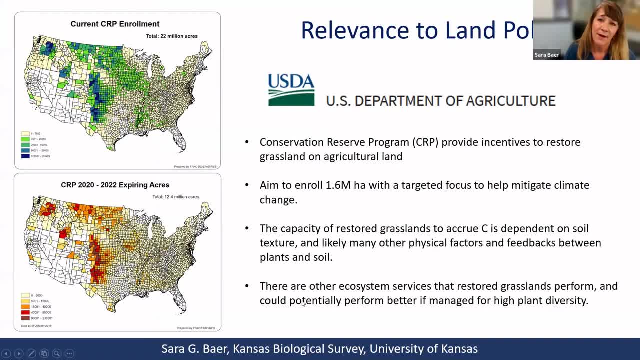 So these knowledge gaps are relevant to land policy. So the United States Department of Agriculture's Conservation Reserve Program is the largest incentive and opportunity to restore grassland on former agriculture. The USDA plans to enroll over a million hectares with a targeted focus to help mitigate climate change. 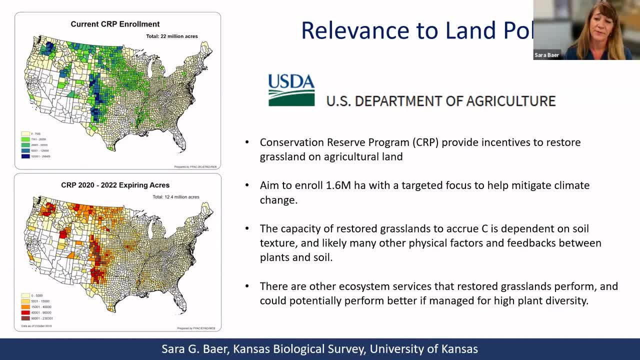 Our research shows that the capacity of restored grasslands to accrue carbon depends on soil texture and likely many other physical factors and feedbacks between plants and soil. Moreover, there are other ecosystem services that restored grasslands perform and could potentially perform better if met carbon-rich soil. 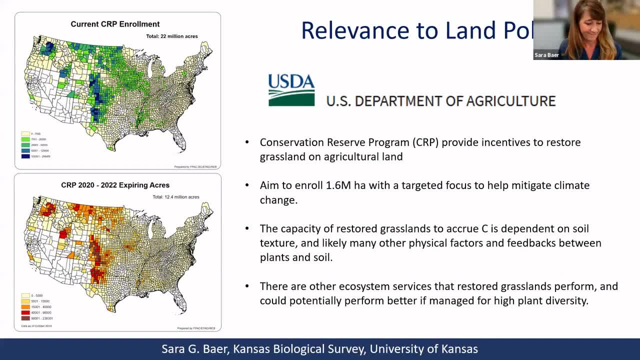 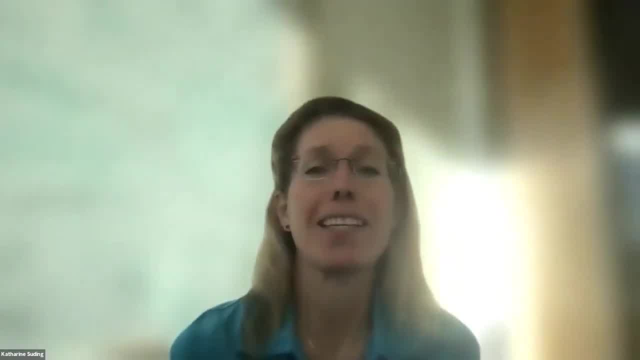 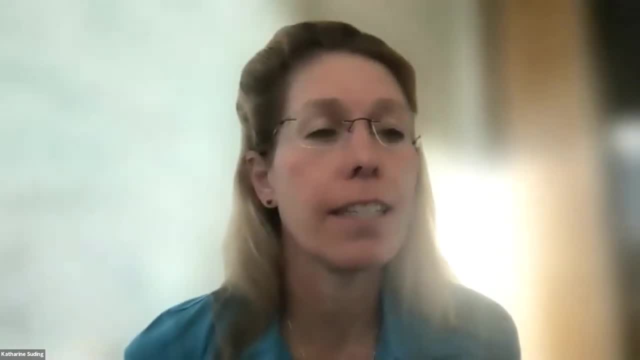 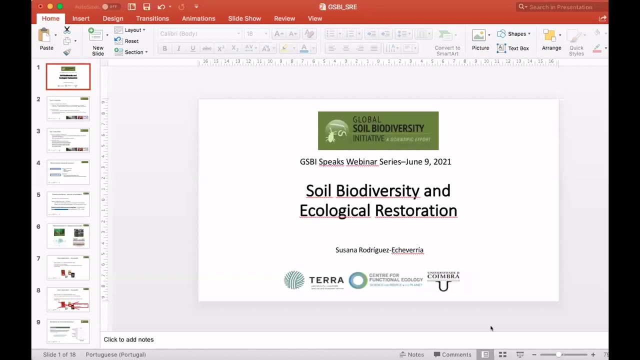 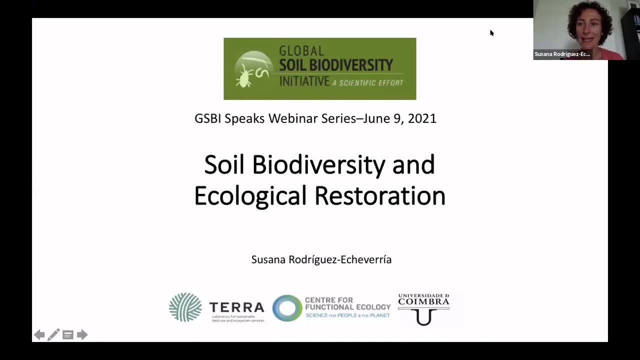 managed for high plant diversity. Thank you, Sarah, Amazing. Um, now I'd like to invite Susanna to share her screen and talk about her work. Hello everyone. Hi Katie, Thank you. Thank you for the invitation. I'm going to talk a little bit. 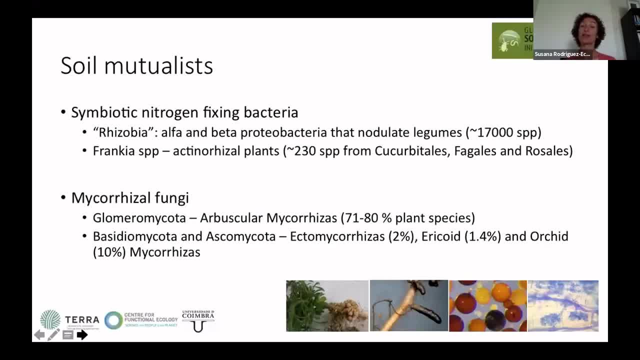 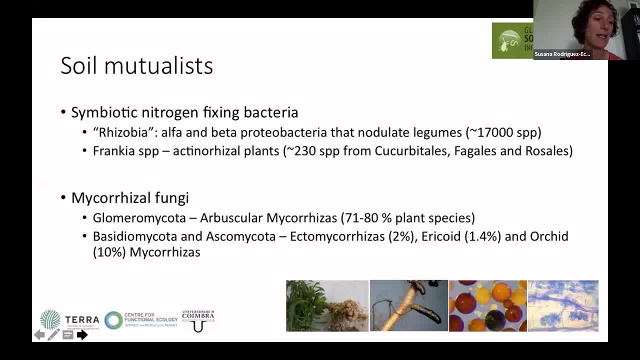 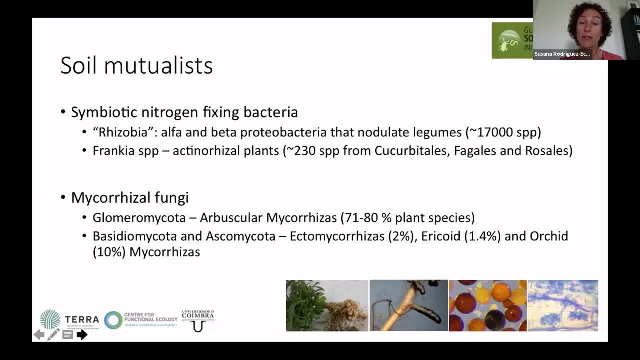 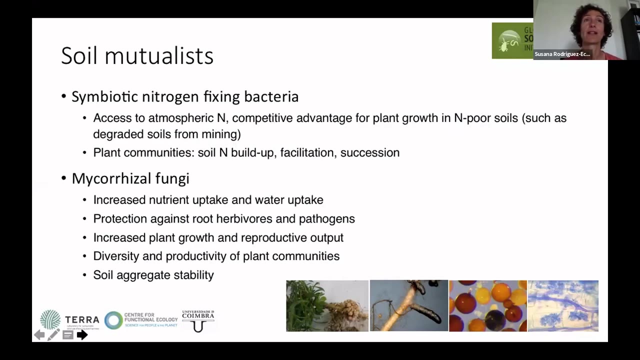 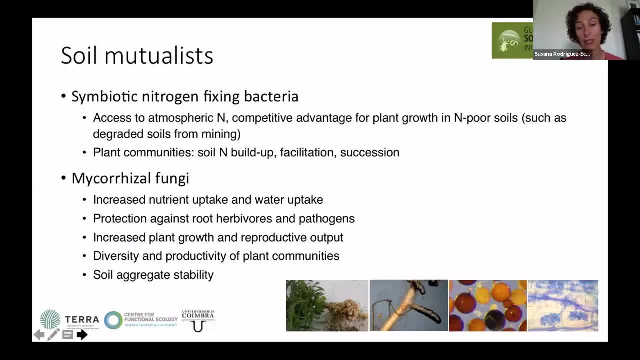 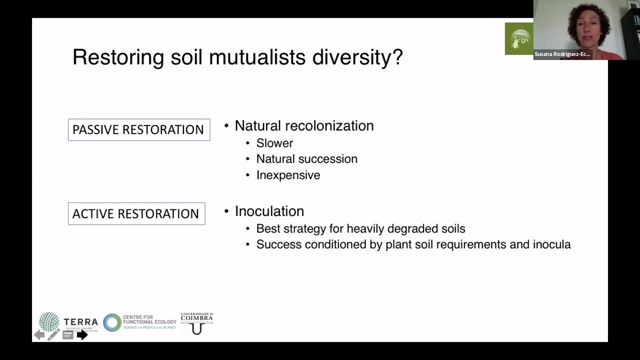 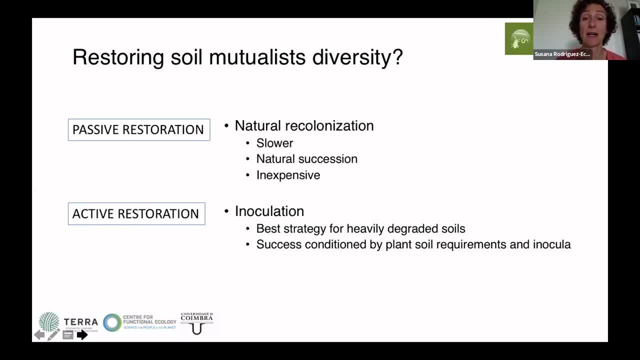 that we can do is just stop the disturbance and wait for natural processes to happen, for natural recolonization of these soils by these mutualists from nearby conserved areas for ecosystem. It's a slower process but it's also very cheap and since it's the natural succession, 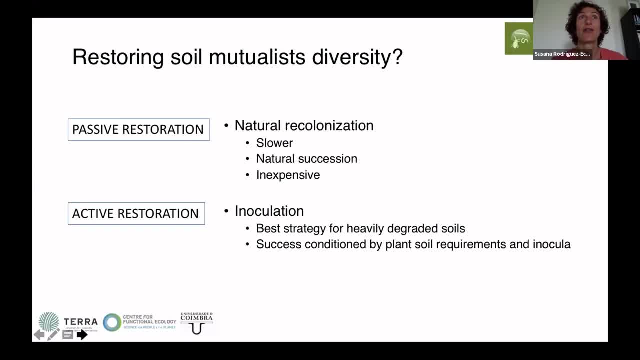 the success of this approach is guaranteed because it will happen what it has to happen in the ecosystem. That it doesn't mean that it's going to recover to pristine conditions, but it's what it can be done Now. in many cases, we don't want that. we want something. 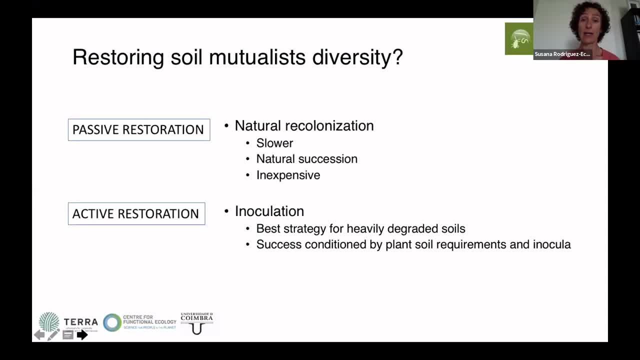 quicker or a stronger action, and then many types of inoculations have been tested for the use of microasulfanil or nitrogen fixing bacteria in revegetation projects or restoration projects. It is the best strategy for heavily degraded soils and there are many studies done. 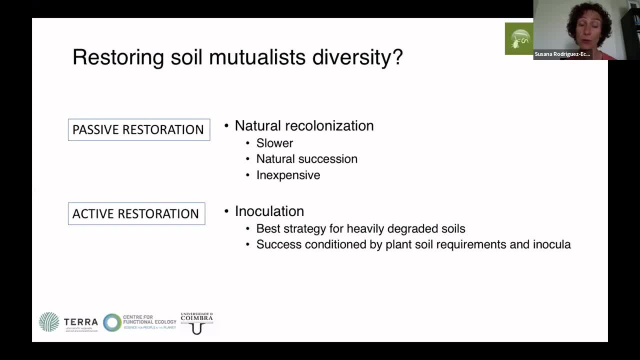 especially for soils contaminated with heavy metals or oil residuals. but the success of these projects, of these active restoration inoculation projects, has been very good. It's a very good approach. The next slide, please. It depends on the identity of the plants and the mutualists, but also on the requirements of plants. 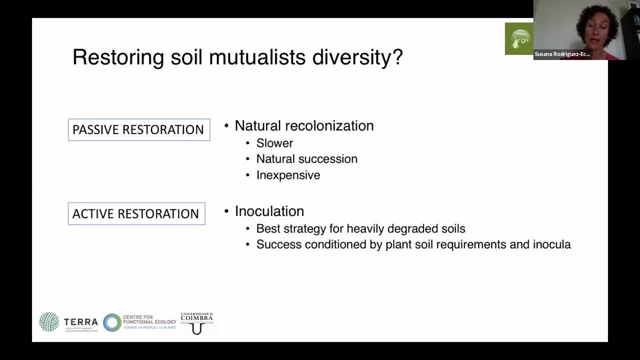 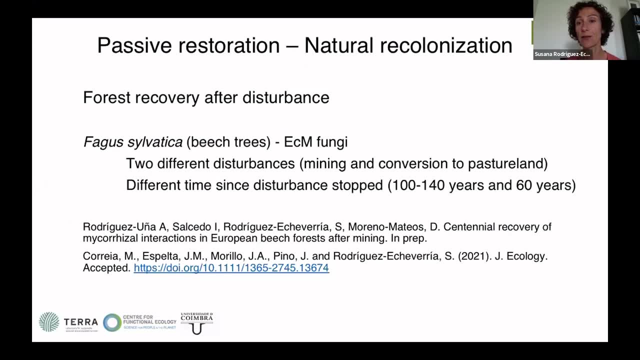 and the conditions of soil, as Sarah was saying before, and also of the inocula, as we will see later. As an example of passive restoration or natural recolonization, there are many studies that assess the diversity of a kind of mycorrhizal fungi that are associated. 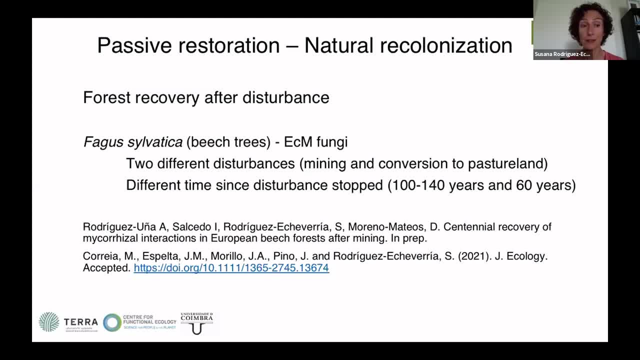 with temperate forest trees. We have been doing some research on this in the last years, specifically with beech trees, with phagus sylvatica and with the associated to mycorrhizal fungi which are essential for the growth and physiology of these trees in natural. 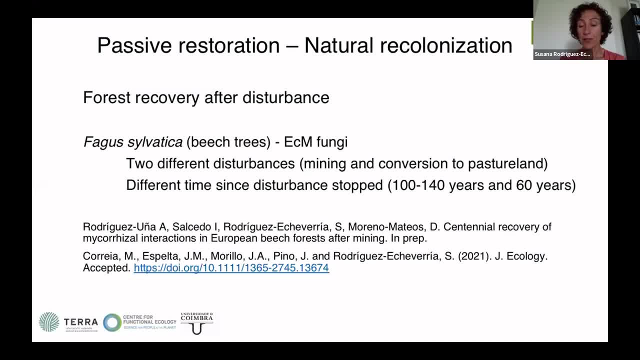 forests. We have studied forests affected by two different types of disturbances. One case was mine mining that destroyed the forest, and in the other case it was in the conversion of forest to pasture land during the 19th century. In both cases, these disturbances stopped a while ago. 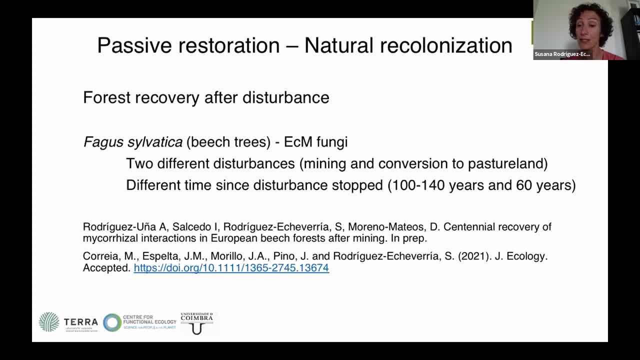 In the case of mining it was between 100 and 140 years ago and in the case of pasture land they were abandoned about 60 years ago and in both cases these are different sites in the north of the Bering peninsula. In both cases, the forest. 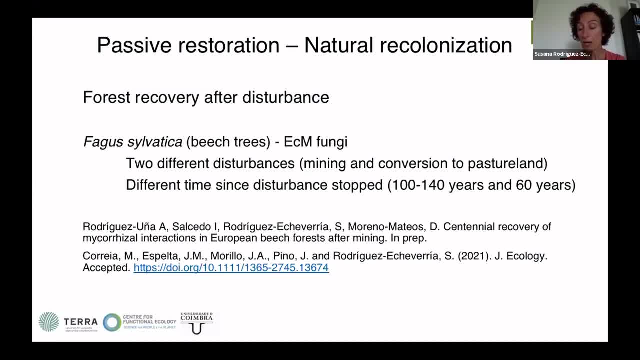 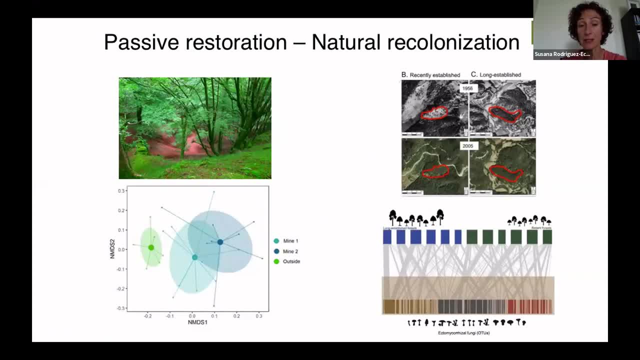 regenerate naturally. We studied what happened with the communities of mycorrhizal fungi associated to these species. As you can see in this image, you have here a mine which has been recolonized by the beech trees, the associated soil organisms. 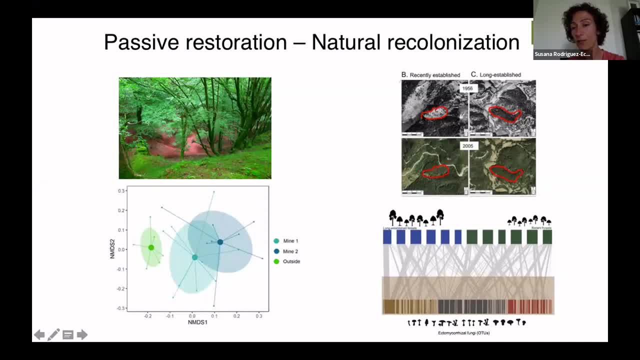 And here you have a photograph- aerial photographs of the forest that were cleared for pasture land and how they have regrown in the last 50-60 years. In both cases we have diverse and abundant community of ectomycorrhizal fungi associated to the roots of these trees. 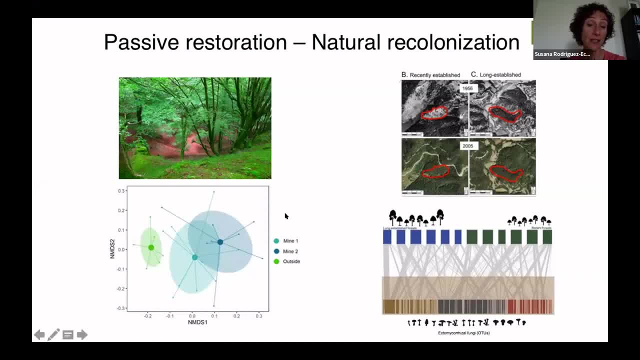 But, as you can see, in both cases, after 100 years or 60 years of recovery, the communities associated with these new forests are different from the communities associated with the forest that did not suffer the perturbation. So the recovery of the mutualism happens. 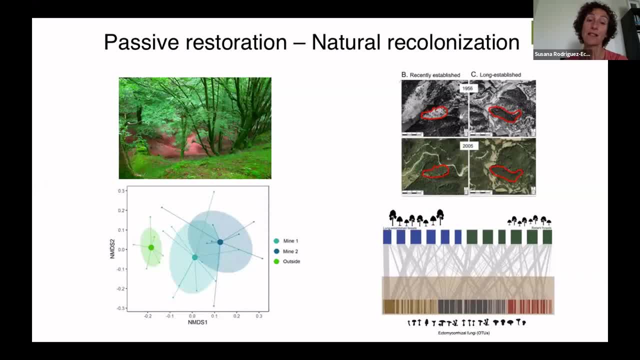 in a natural way, but we don't know if these differences in community composition are having any effect on the functioning of the forest, And this is one of the things that is starting to be addressed now. Also, the colonization will depend on the conditions of the 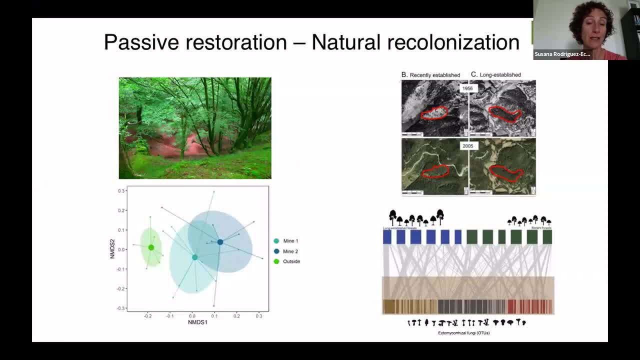 soil that sometimes, in most cases after disturbance, the concentration of nutrients and the pH of the soils is different, And that is not going to allow the establishment of all of the same species that were there before, But also it will depend on the capacity of these. 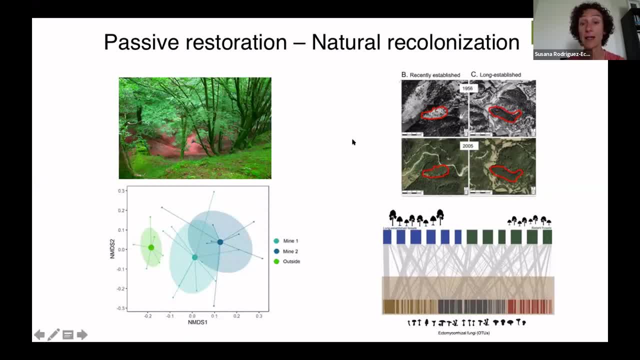 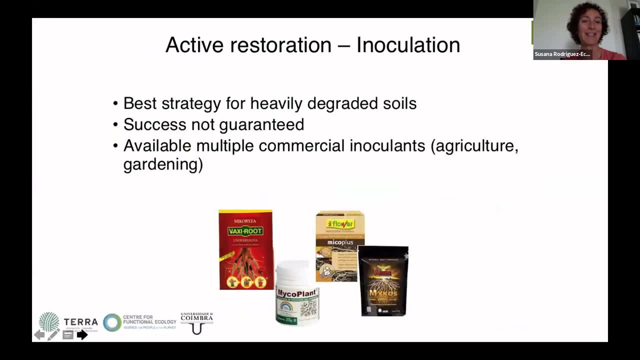 of dispersal of this fungi from nearby forest. The other option, inoculation, is management option that is very well established and they has been using a lot. Also because inoculation with nitrogen fixing bacteria or mycorrhiza, is something that is has been very well established and studied in agronomy. 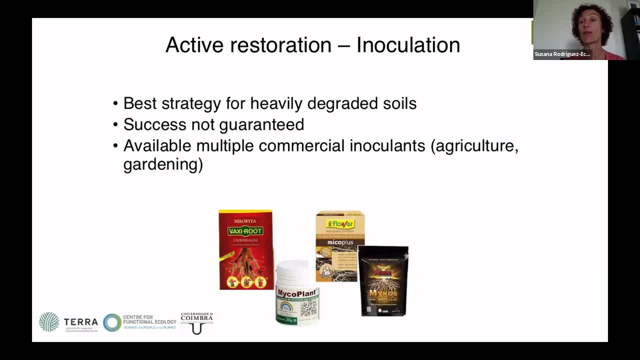 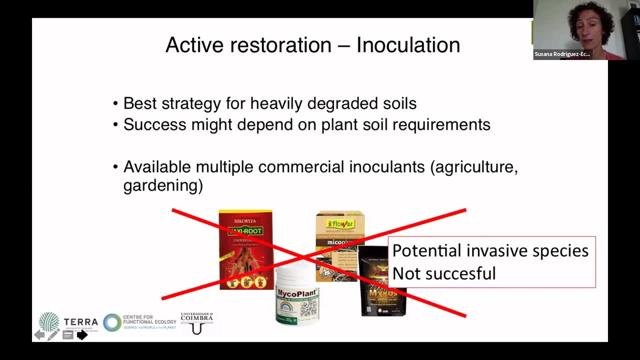 and also in the gardening industry. You can. if you look up in the net, you can find lots of different inoculants to apply for your plants or your crops. But what the studies, what different studies have shown, is that you shouldn't use these commercial inoculants. 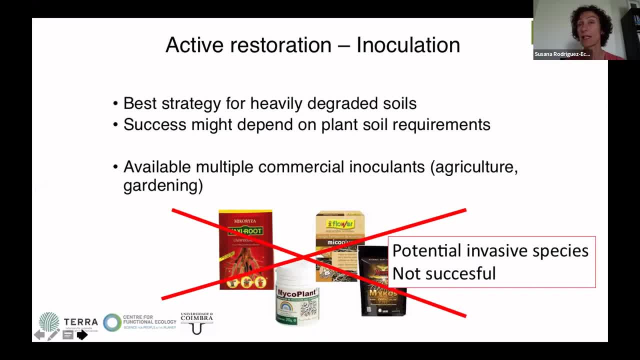 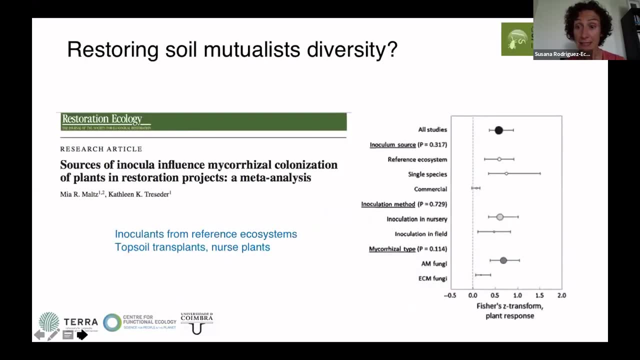 in revegetation projects, in restoration, because they contain a full amount of nitrogen and they are a very important species that can be potentially invasive, And also, in many cases, they are not successful in natural terrestrial ecosystem. This meta-analysis shows precisely this. 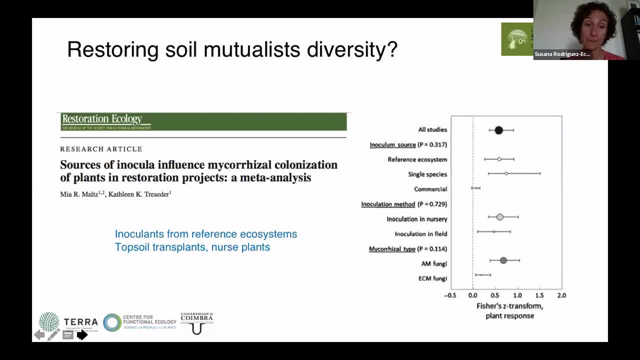 You can see that the success of the restoration project improves with the application of mycorrhizal fungi, But this improvement does not happen for commercial inoculants, So the best option is always to obtain an inoculant from reference ecosystems that are nearby the disturbed site. 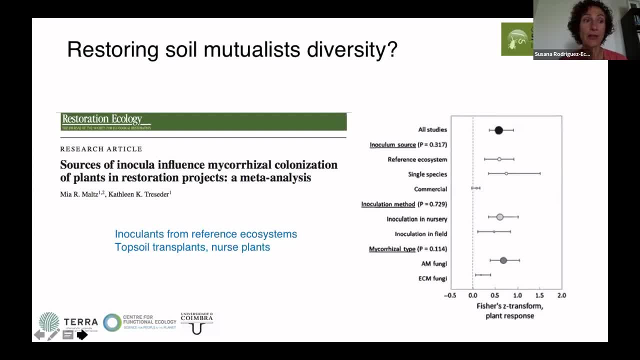 And you can use a mix of isolates from these reference ecosystems or single species isolated from these ecosystems. You can use the whole soil as topsoil transplants or cultivate these mutualists in appropriate systems, create nurse plants and put this to help restoring the system. 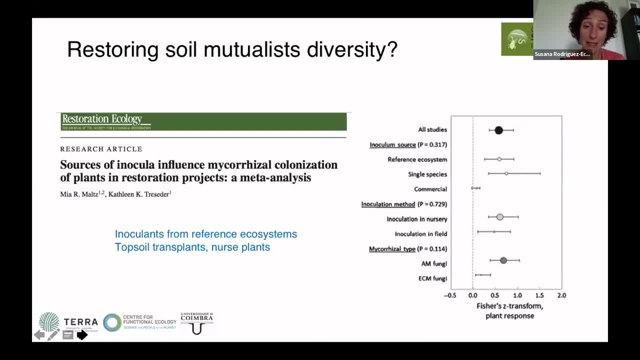 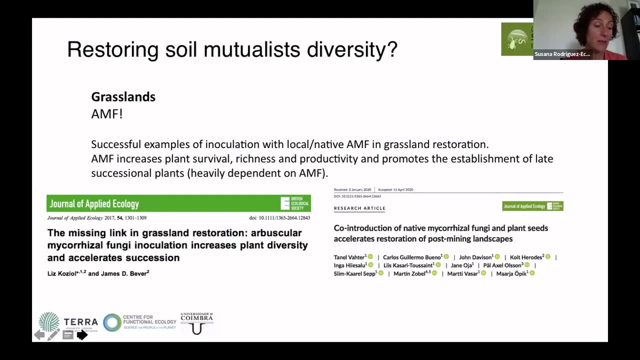 There are many different options. In many cases they have to be tested because there is no one only solution for all cases. One interesting case is the restoration of food islands, especially in North America. There has been many studies done in the restoration of food islands. 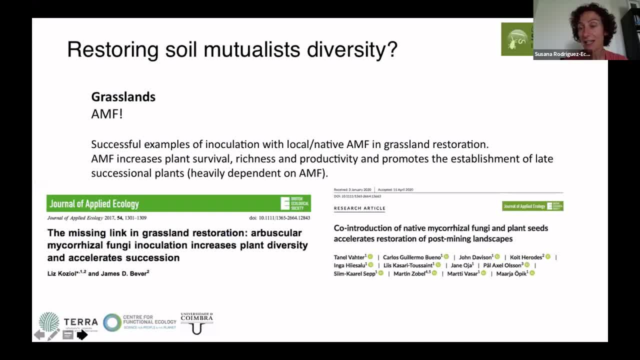 The application of mycorrhizal fungi in this restoration. The inoculation with local and native fungi increases plant survival richness and productivity in these projects and promotes the establishment of late successional plant species which are more dependent on mycorrhizal fungi. 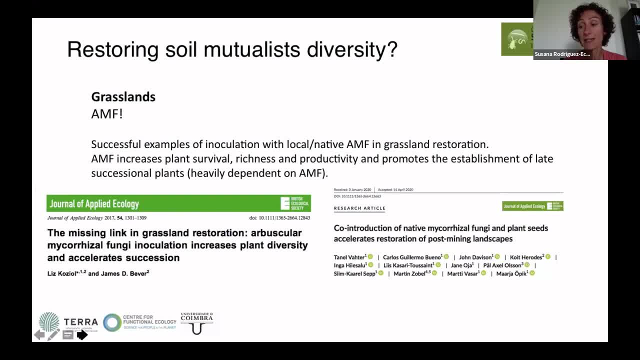 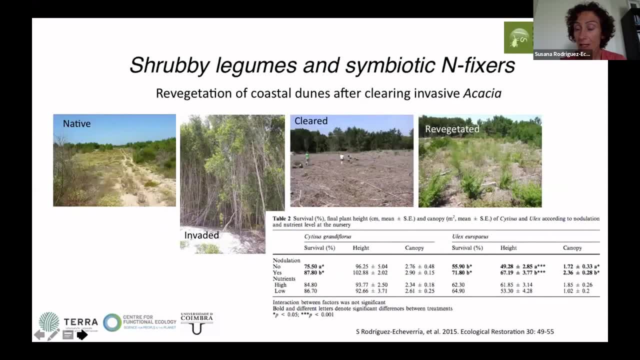 So they are essential components of the ecosystem and essential components for the recuperation of this ecosystem. Here I just saw very quickly a piece of study that we did in the recovery of coastal sand dunes that were invaded by an Australian acacia, which 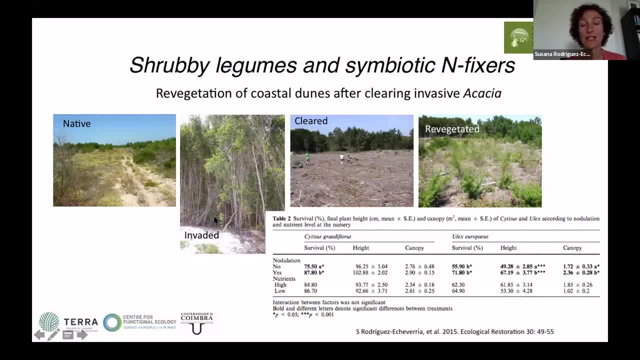 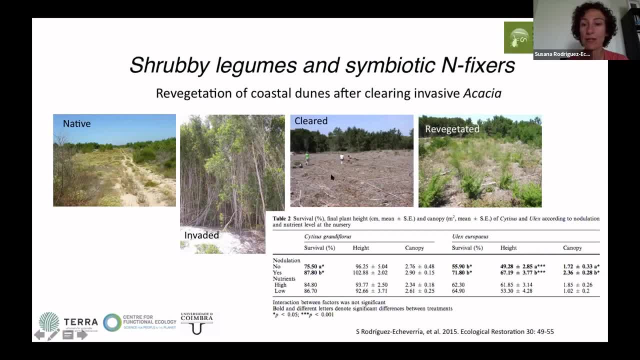 We did a pilot study using native shrubs. We did a pilot study using native legume shrubs to recover these vegetated areas And we also saw that in the nodulation. so the symbiosis with the nitrogen-fixing bacteria will increase the probability of survival. 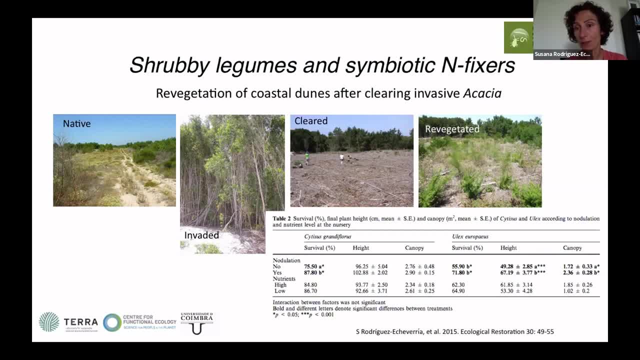 and the growth of these plants. So again, as for annuals of perennial annual species, you can also use this kind of inoculation techniques with native mutualists to improve the success of restoration projects using woody species. So there are many if you go to the literature. 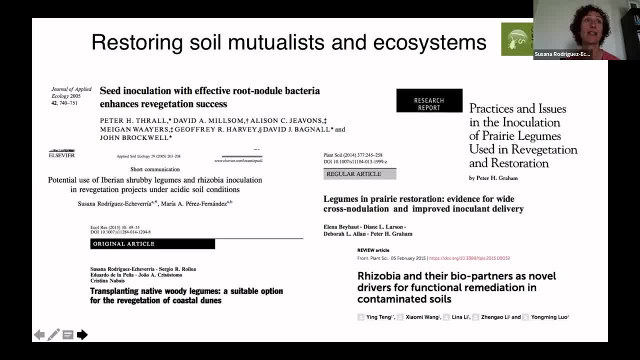 to do a search. there are many, many studies trying to do this, Talking about the major gaps in this area. although there are lots of research, there are still many gaps in our understanding of how this works in different ecosystems, because most of the studies are done in temperate ecosystems. 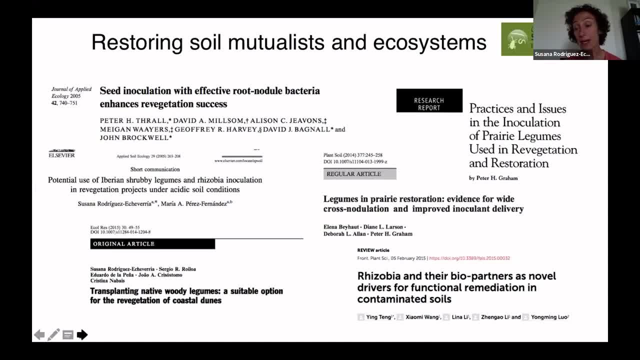 And also many of these studies are done only with one kind of mutualism, And it was very interesting to use both nitrogen-fixing bacteria and mycorrhizae when legumes are present. Also, many of these research reports are focusing on individual plant growth. 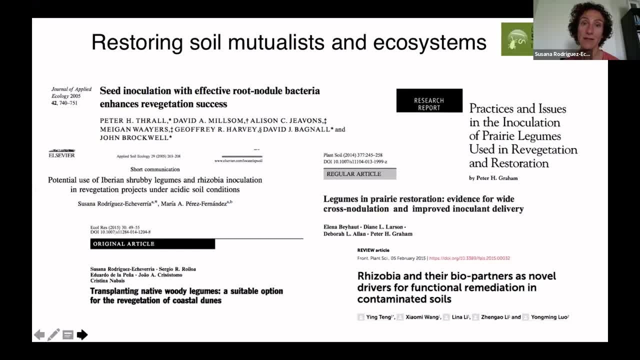 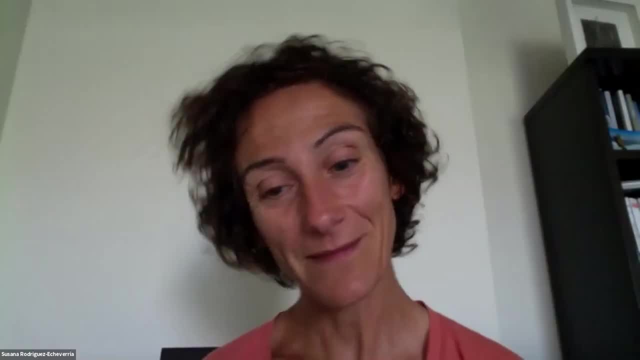 We need to expand our knowledge on different ecosystem services and different processes to see if the inoculation or the natural colonization are better options for the recovery of this ecosystem. Thank you very much. Thank you, Susana. Yeah, that's very close to my heart. 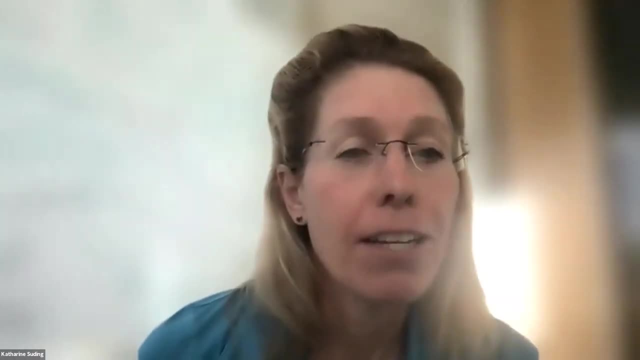 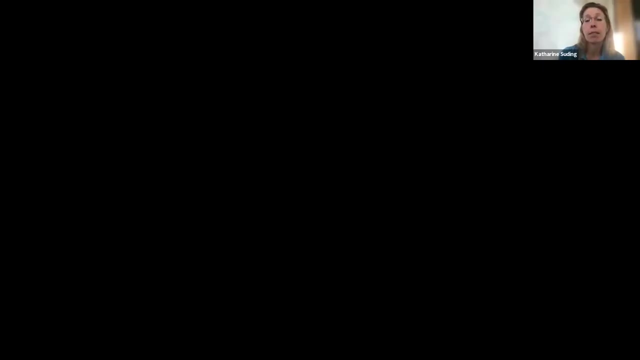 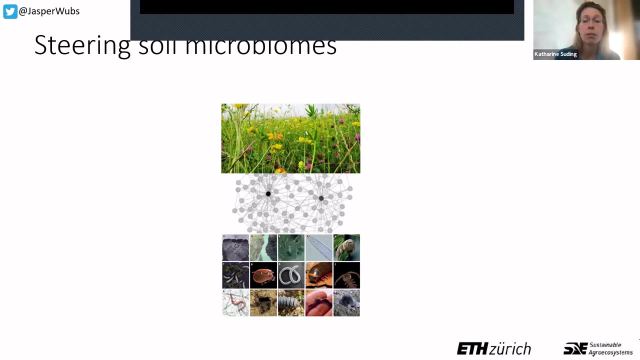 That's just a question. Incredible work. So now I'd like to invite Jasper to talk about his work And I'd like to just remind the audience, please, if any questions occur to you, just please use the question and answer tab to ask them whenever you have any. 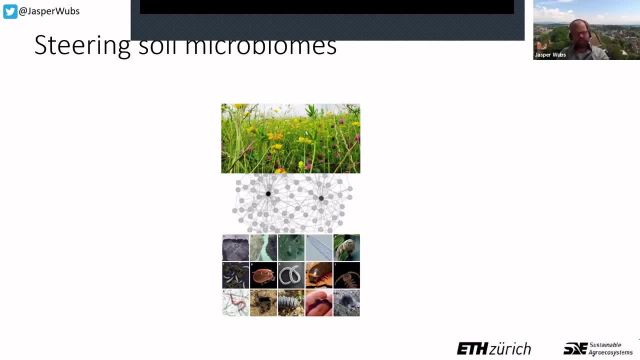 So thank you. OK, thanks, Jasper. Thanks, Katie. I apologize for the black boxes in the top. I cannot get rid of them. So my name is Jasper Wups. I work at ETH Zurich And my work focuses on steering soil microbiomes. 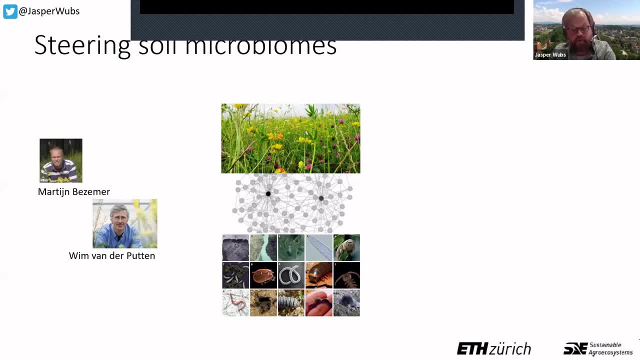 And I came to this as a plant ecologist focusing on plants And I was introduced to the beautiful world of soil biota by Martijn Bees and Wim van der Putten during my PhD And they showed me the amount of interactions that were going on above ground and below ground. 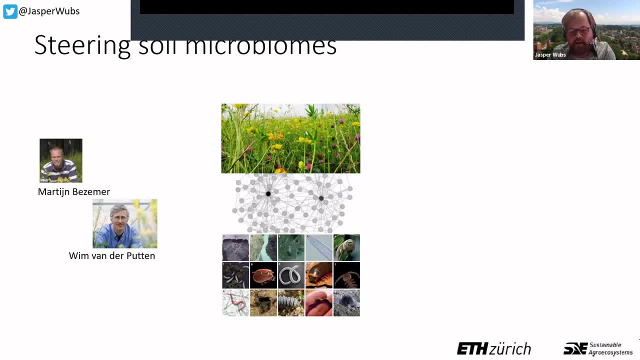 So above ground you have 30, maybe 40 species per meter Square. in the soil you have thousands of species that live together- bacteria, fungi, all kinds of fauna- And all of these interact in some way, And so I think there have been several decades of research. 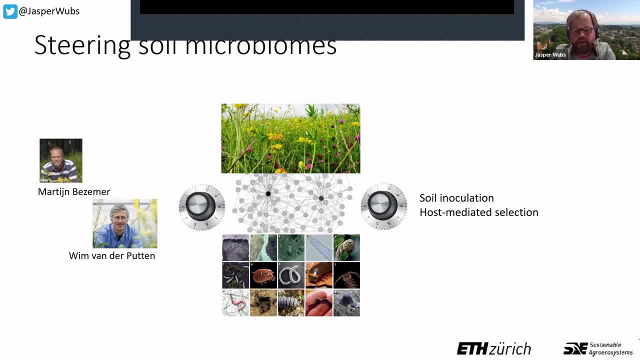 on this And I think the field is moving in the direction where we're looking into ways in which we can manage or manipulate these interactions for specific goals, for instance restoration And my research. I start from a different point than most people. 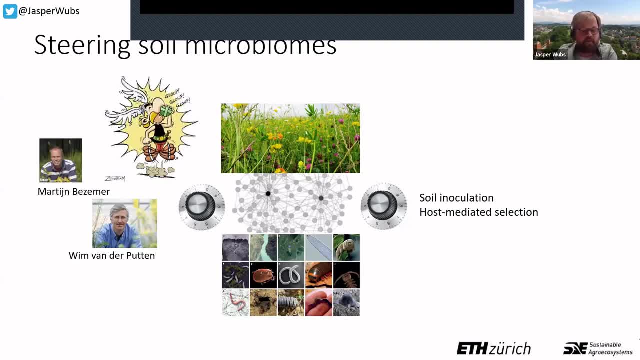 My research assumes that there's not one or a few microbial players that are super, super, super well-functioning, that do everything, But in fact I think, or I start from the point, that actually you need to get a whole community of soil biota. 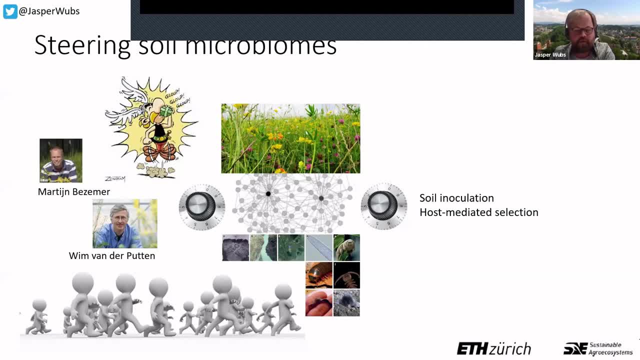 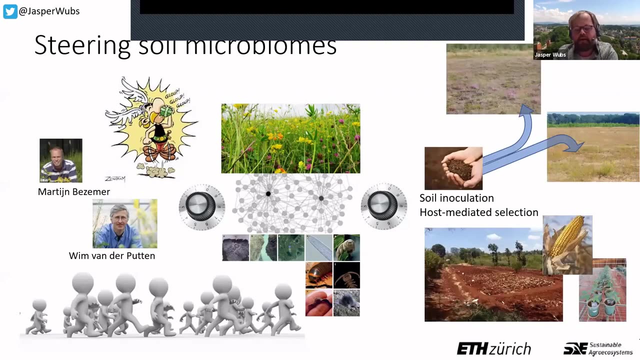 to move in a direction that's beneficial for what you want to do. So I'm looking for methods to change and steer the whole soil microbiome for soil functioning in general, And I've used different methods to do that. One is soil inoculation that I've used in field experiments. 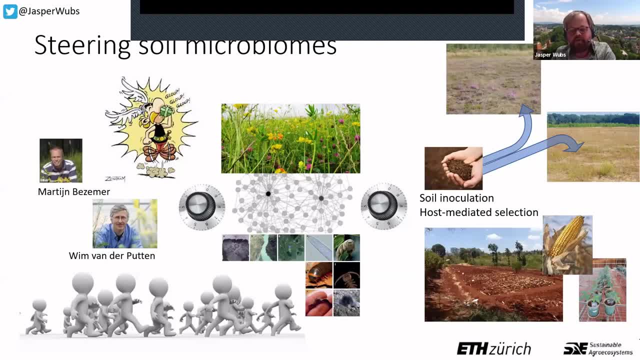 where we could show that the microbiome can actually determine in which direction the vegetation is developing, And the other method is host-mediated selection. So there's a way to manipulate the composition of the microbiome And we use that now in central Kenya to see if we could optimize. 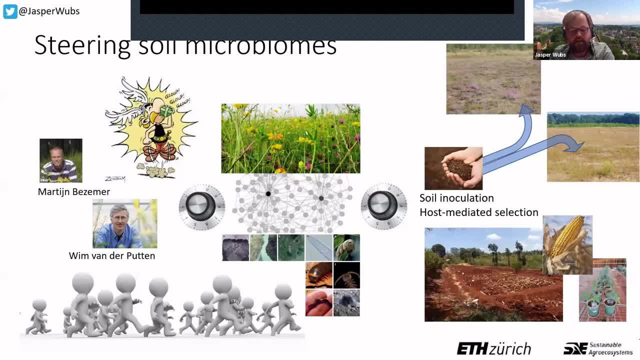 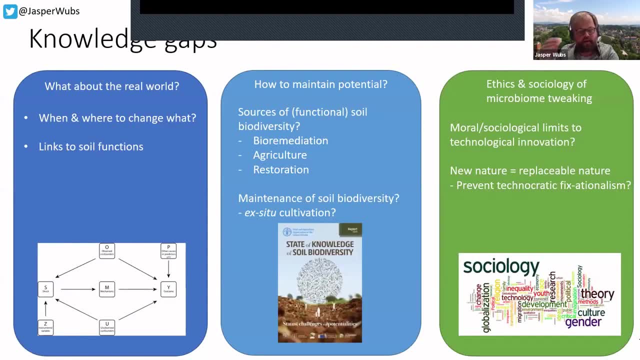 maize, And then we can look at the results of this evaluation- And I think that's a really important point- to see if we can actually change the way we use this, And I think that's really important side of questions, in particularly with respect to restoration and- and we need to do that in the field- 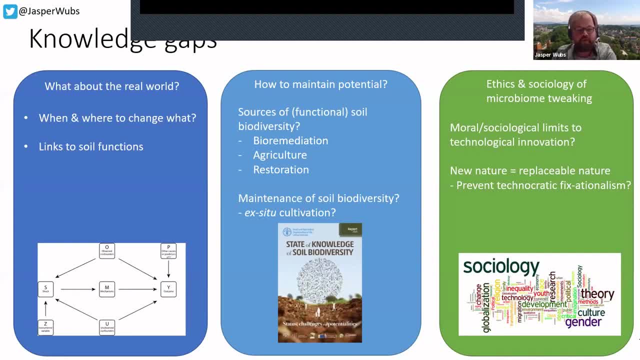 and we also need to link, i think, much of the soil biodiversity more explicitly to to how soils function, to be able to give those answers now. the second is: how do we maintain the potential soil biodiversity? i was recently involved in the state of knowledge report by the fao. 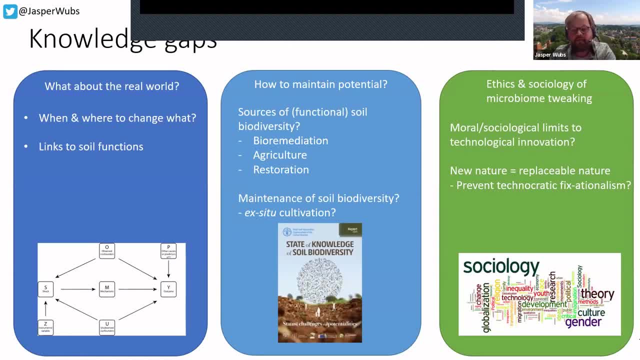 and there's a lot of microbes that have been found that they're beneficial for bioremediation for instance. but when you look at those papers there's actually very few that document where these microbes come from. so it seems that the best guess we can give that, if you want to, you know, if you. 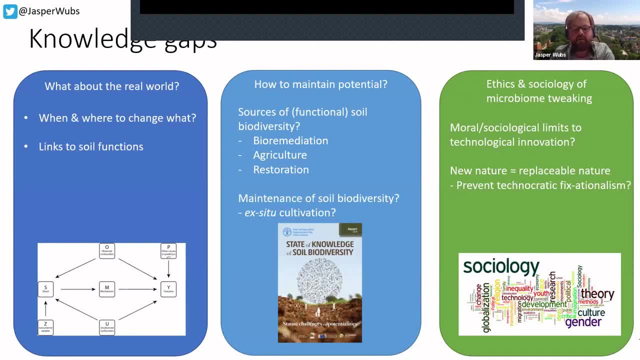 want to get rid of an oil spill, for instance, you go and look for microbes that live in oil spills, and that's about the best answer i think i could give you at the moment. so i think we need to to dig into that deeper. where is this biodiversity coming from and also how can we maintain it do? 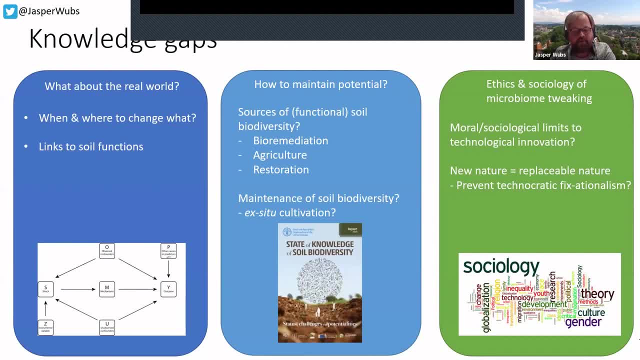 we need to maintain it somewhere, you know, outside of the soil, in a laboratory, or or can we? can we in the, in the, the management of our landscapes, can we make sure that we keep that biodiversity there? and the third thing is a bit more broad scope thing it's. it's about the ethics and 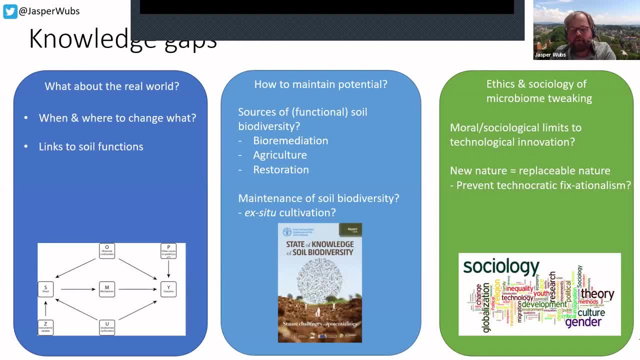 sociology of microbiome tweaking. um. so i think many people in at least i uh in restoration equality we have a bit of a technocratic approach to things. we find ways to fix perceived problems. we also have to take into account how society and how people relate to 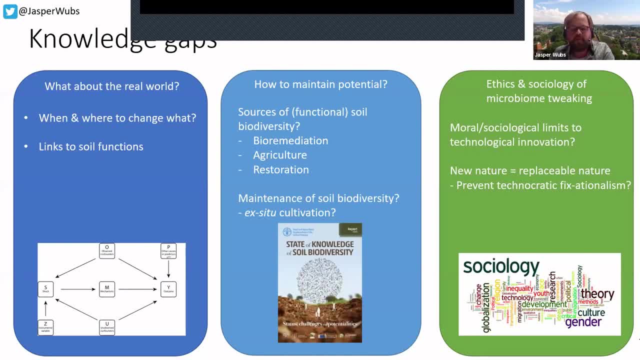 these, these innovations or these interventions that we propose, um, we should discuss what, what is, what is proper, uh, in, in, in moral terms and in sociological terms, in different cultural contexts? uh, and one thing that that has always struck me is a discussion with a philosopher. he said: 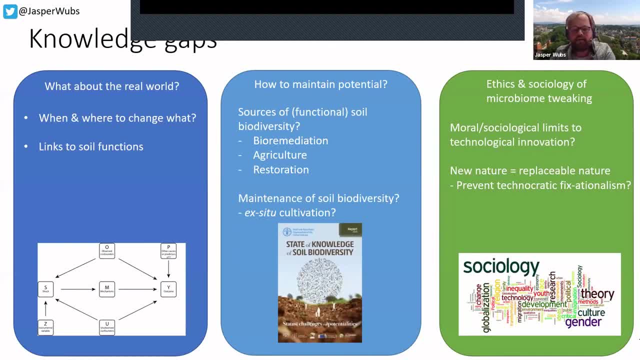 well, okay, the better you get at restoring nature, uh, the more ammunition you're actually giving other parties to destroy nature, because you know you're now better able to restore it. so why bother about conservation? why do you need to conserve? and i think in all our restoration efforts we are seeing that we can restore but we cannot restore. 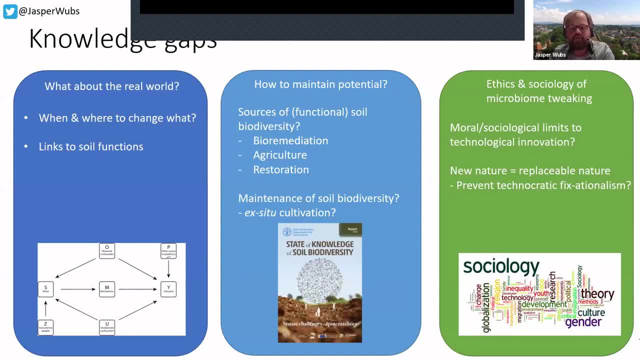 perfectly, not even close to perfectly, and so i think there's a real risk that that, um, you know, if we that we should not over emphasize our ability to restore- we can restore, we can make things better- um, but it's, it's not not nearly as good as what we. you know what we, what we're losing. 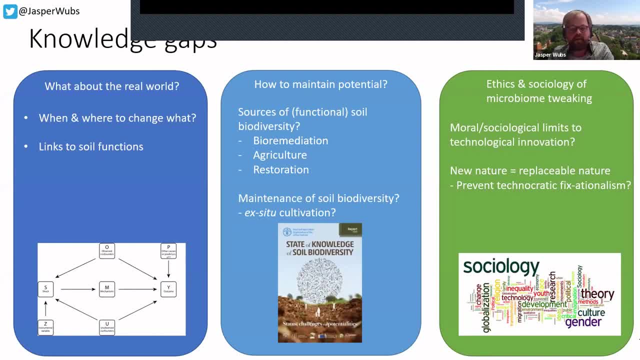 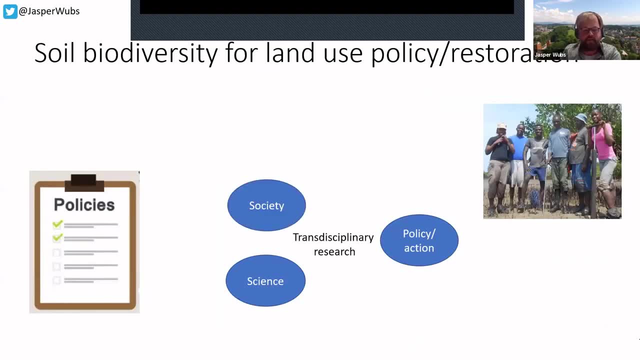 and so i think we need to be explicit about that and study that and study how that relates to to society generally. um, now for for policy, i think indeed, this link to society is very much key. we need to find out, not only you know how, how people in social sciences, are doing things, but particularly 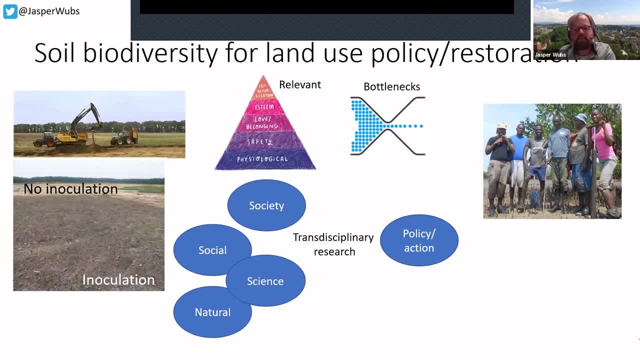 we need to find out what what is relevant for local communities, what questions are relevant for them and what are bottlenecks in in the problems that they perceive, and can we find solutions for that? i think in the in the resource-rich communities that i, for instance, work in. 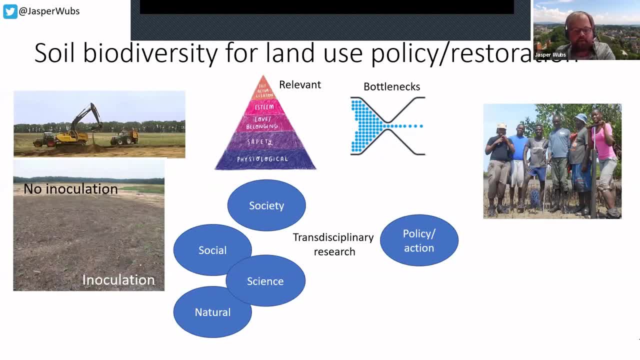 we need to to um, we need to develop the technologies, we need to to develop the options of improving things and those can then, after we, we, we know the rules of the game for those, for those interventions, we can start applying and we can can do more direct research. 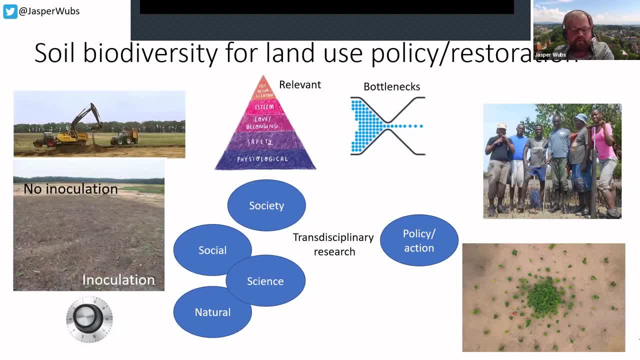 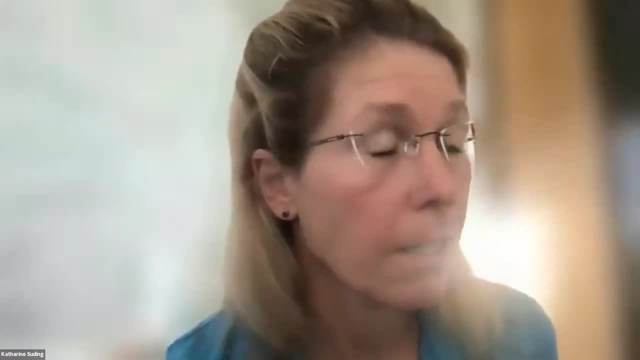 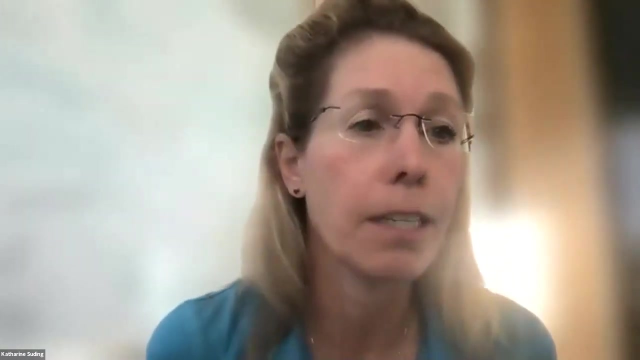 in other communities and and get them to solve the, the problems they may be in. um, that's all i want to thank you. thank you, jasper, um and and i really, really appreciate you bringing up um, the, the social and um and and and policy dimensions of of what we're we're talking about today. um, that's great. 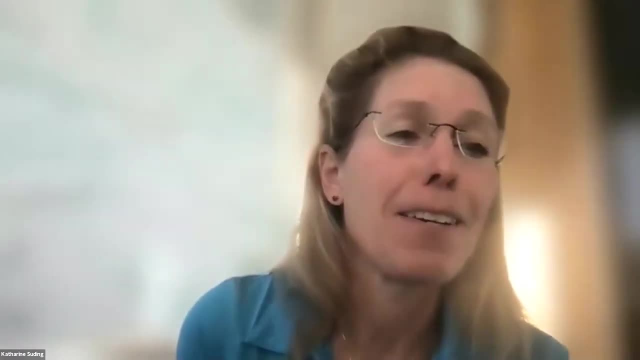 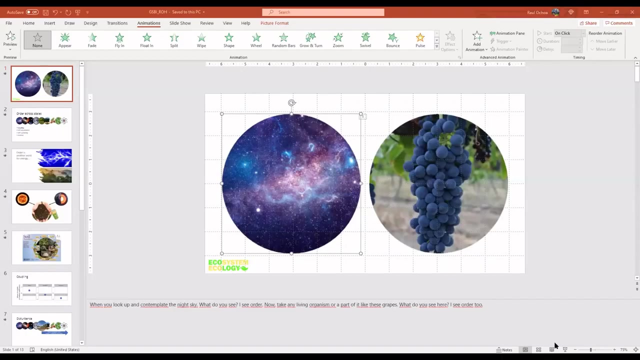 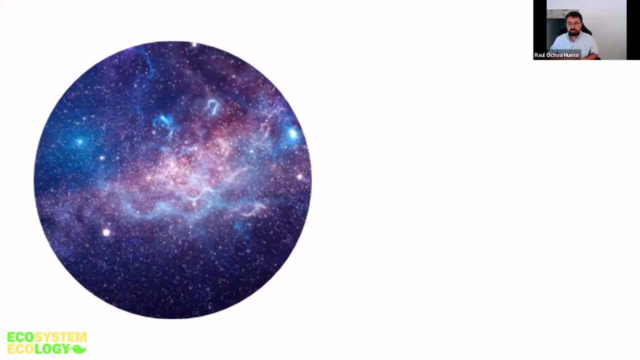 um, raul, um, you're next, i'm gonna hand it over, okay, perfect, thank you. okay. i will share my screen now, okay, i hope you're seeing it okay. so i'd say: when you look up and contemplate the night sky, what do you see? i personally see order. now take any living organism or a part of it. 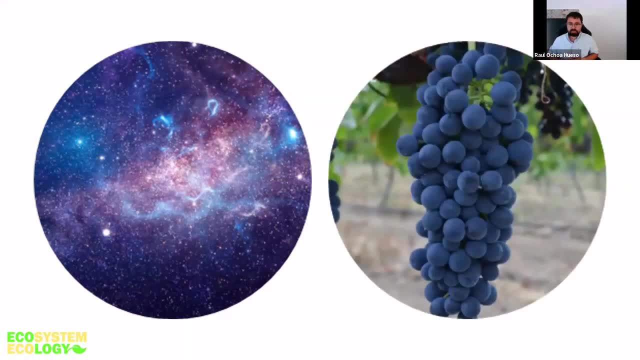 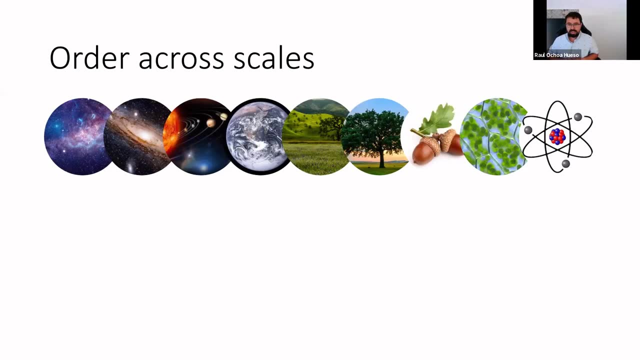 like, for example, these grapes, and what do you see? now i see order too. actually, nature is ordered across scales, and this order means that everything must be somehow good, connected to everything. such orderly connections define how systems are coupled. this order arises naturally, which means that it is self-organized. the other two main characteristics: 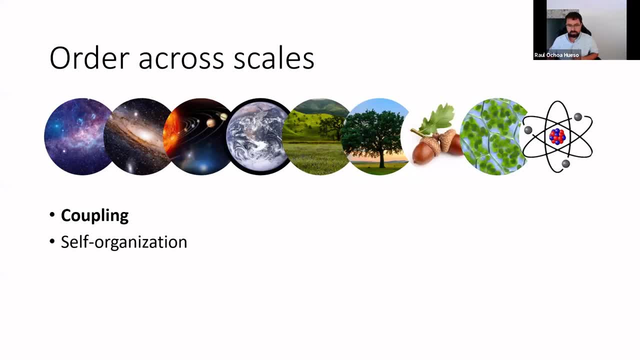 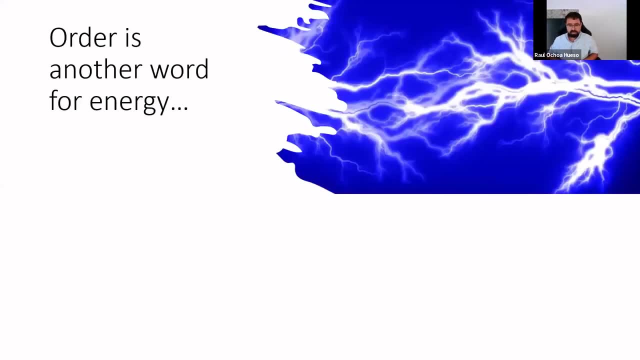 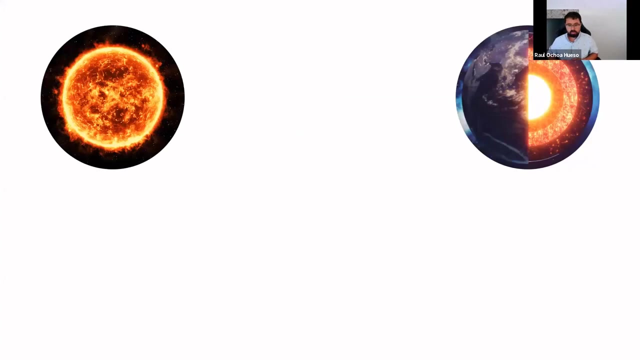 of self-organized, ordered systems is that they are self-sustaining and dynamic, or in other words, they evolve. the amount of order of a given system defines the energy stored within that system. hence, orderly, coupled ecosystems should be able to function more efficiently. in our planet, the energy comes from the sun and from the interior of the earth. 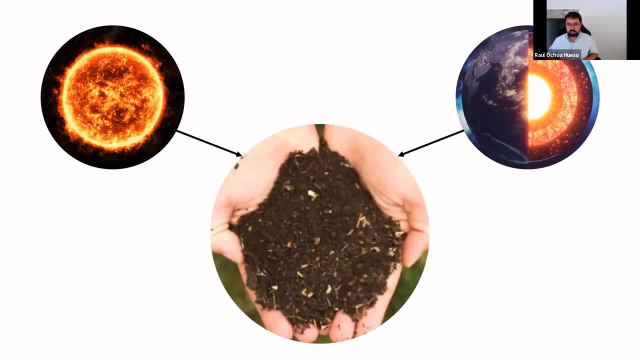 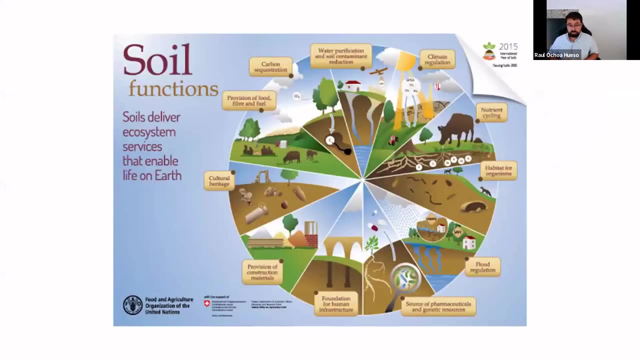 and we know that soils play a key role in the processing, transfer and storage of that energy. somehow it is like the soil is the battery that helps to keep ourselves and the earth ecosystems running. this is actually compatible with the view that soils are central to support life on earth and, of course, soil biodiversity is central to this. 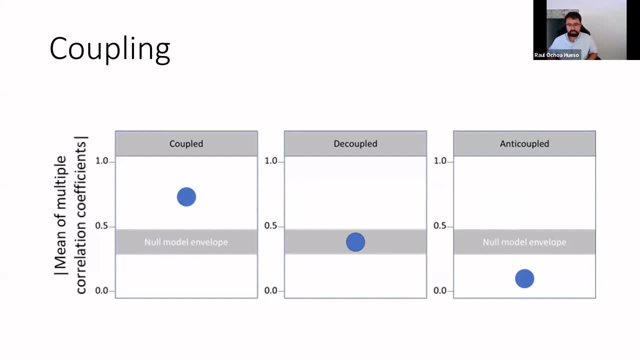 now i hope that i have convinced you that order across scales, or in other words coupling, is a critical feature of functional ecosystems, including production systems actually based on associations and other structures and solutions. so in this case, i have presented the example of the solution of an analysis that i developed within the lab, with a lab called the. roberto honeywell, and there is a lot more to say, and i'm happy to do this, but i bones editing. this video of the system can be found in the original modeling approach, which is what i use to define coupling operationally in my research. ecosystems can be found in free coupling estates: coupled, de-coupled and anti-coupled. are we ecologists normally look for coupled patterns, right? seldomly care about the couple of ones, and i would dare to say that we never look for anti-coupled patterns. am i right? like i said, we can keep on using them for another long time. why wouldn't we? 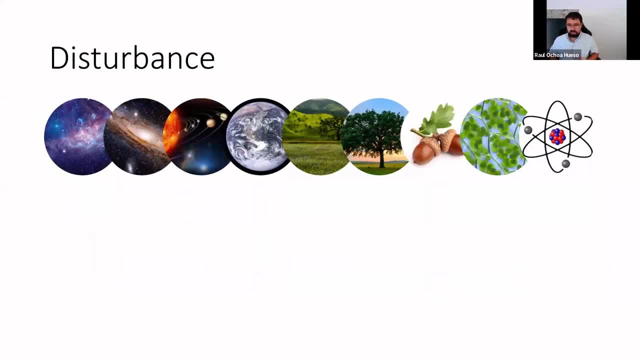 for another long time. why wouldn't we? nature is ordered across scales. So what happens when we break the fractal nature of coupling? The disorder wave propagates to the lower level and that results in a generalized energetic downgrading of ecosystems. So in other words, if we want to bring back the energy and 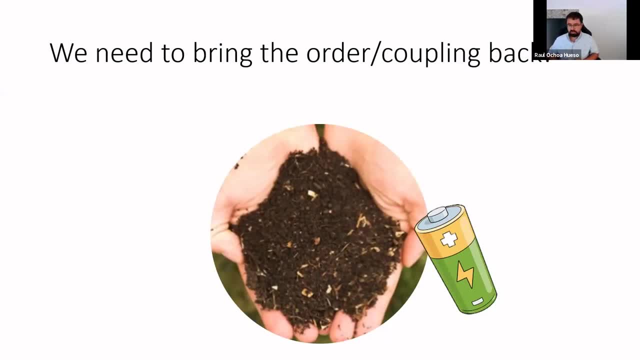 the functioning of the soil battery and its associated biodiversity. we need to bring the coupling back. We must do so by considering the three main characteristics of coupled systems that you know already: That they are self-organizing, self-sustaining, and that they evolve. 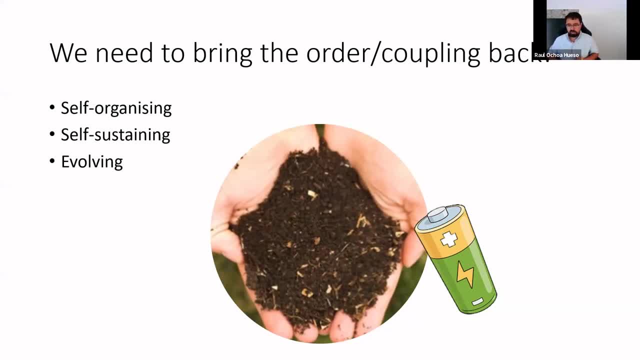 And also that they need to be fed an ordered source of energy to be able to comply with the second law of thermodynamics. And so how can we bring the coupling back? It is a matter of how we bring the coupling back. In my opinion, we need three basic ingredients. First, we need to bring back the soil organisms. 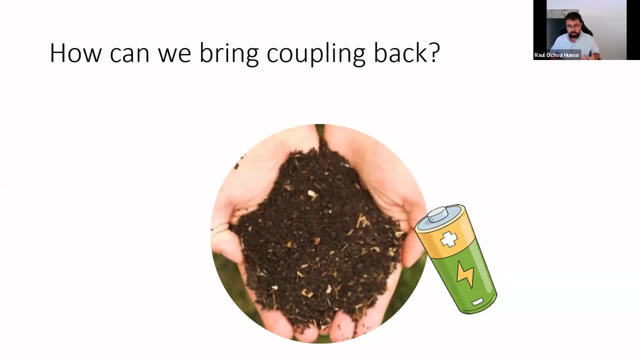 that may be no longer present, For example through inoculation, like Jasper or Susana said before. We also need seeds of plants that will contribute to recharge the soil battery by pumping energy from the sun into the soil, like Sara, for example, suggested. And, last but not least, we need large 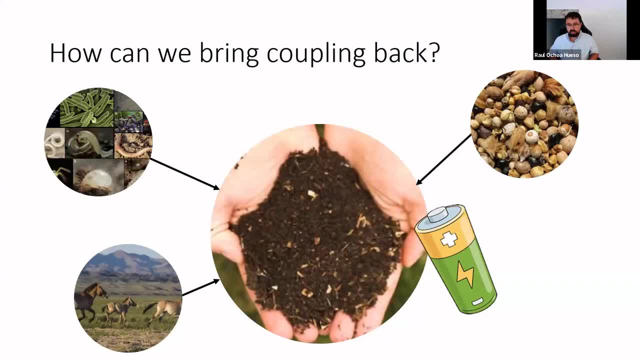 animals that are able to survive in the soil. We need large animals that are able to survive in the soil. We need large animals that are able to survive in the soil. We need large animals that are key to the circular economy of the system. After this, everything else should follow. 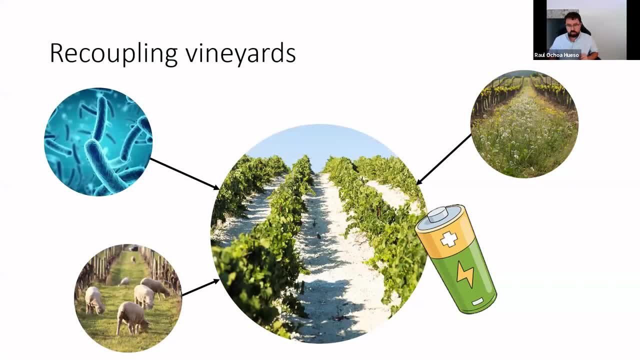 And this is actually the approach that I'm taking in my research to regenerate the life of vineyards from the Red Serri region in the south of Spain. These vineyards have a hugely long history, since the times of the Phoenicians and the Romans, But they are now highly eroded and biologically 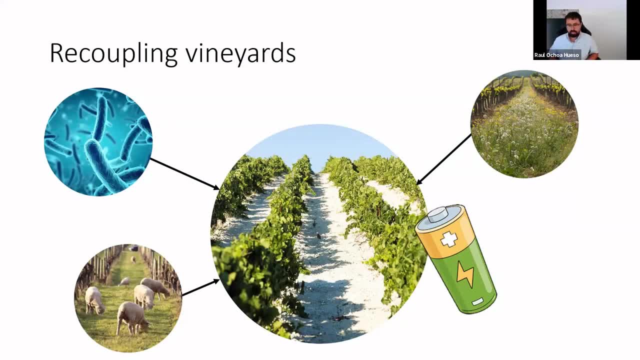 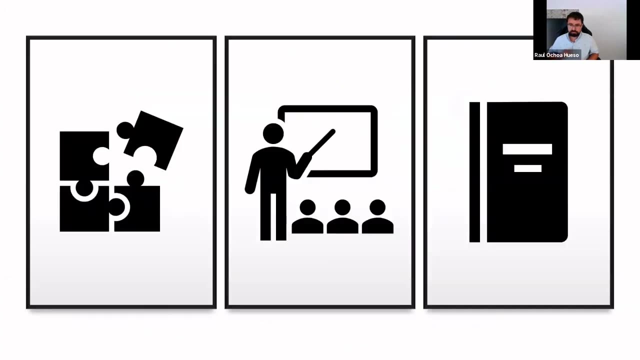 impoverished. They are now highly eroded and biologically impoverished. They are now highly eroded and biologically impoverished. The to this, My goal with my research is to bring the capping back. For this I'm leading to research and innovation projects. One is called Living Soils and the other one is Future Vines. 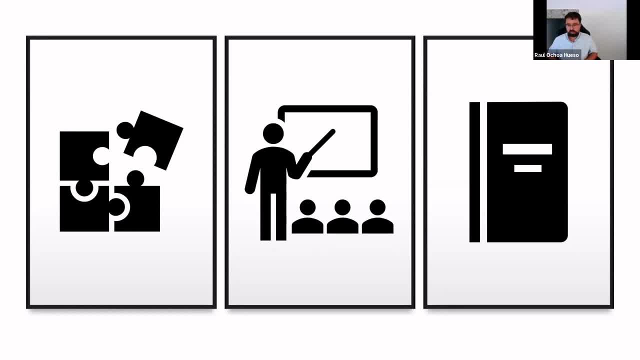 One of my main goals with this project is to generate manuals that can be available to growers and wine makers and to be in touch with various stakeholders, Thus being involved in various projects, thus being able to steer the future sustainability of vineyard soils from my region. 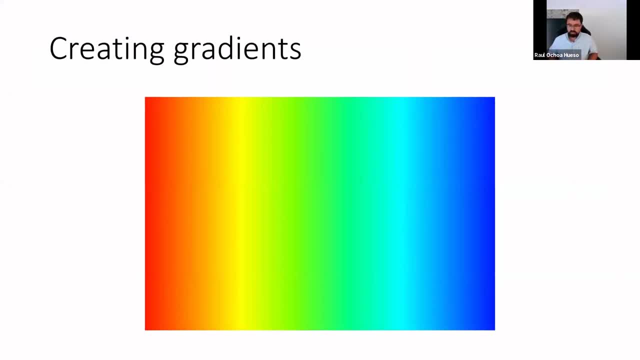 To me, one of the critical aspects to achieve this is to create different types of gradients that will channel the fluxes of energy and matter. If you think about it, this is somehow equivalent to bringing back color to ecosystems. So let's put back the color to our ecosystems. 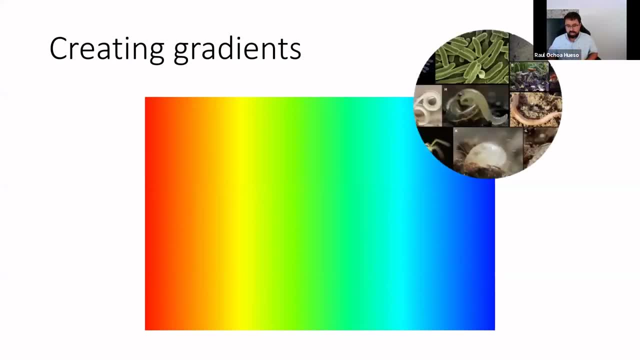 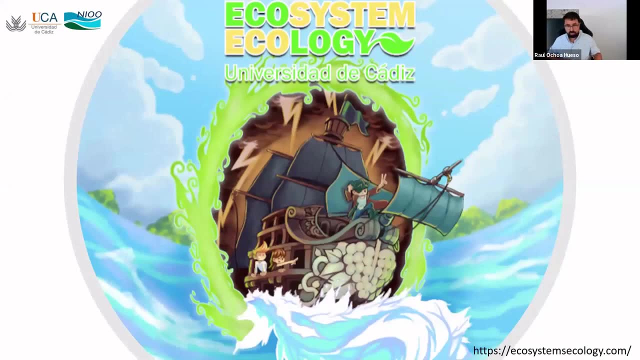 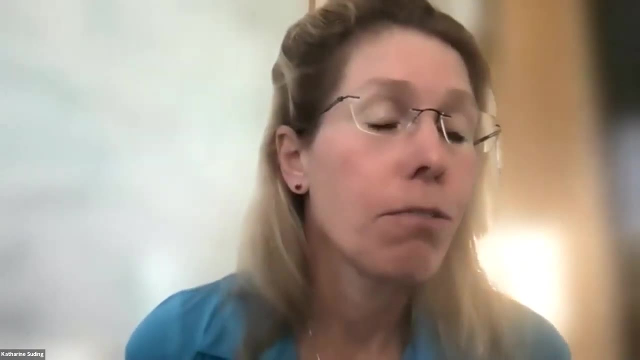 and let's not forget that soil organisms are a critical component of the unseen palette. And with this, I thank you for your attention. Great, Thank you. Thank you, Raul. So now I'd like to invite all the panelists to turn on their videos. 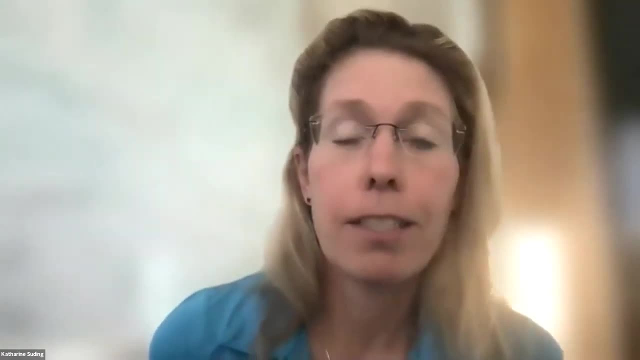 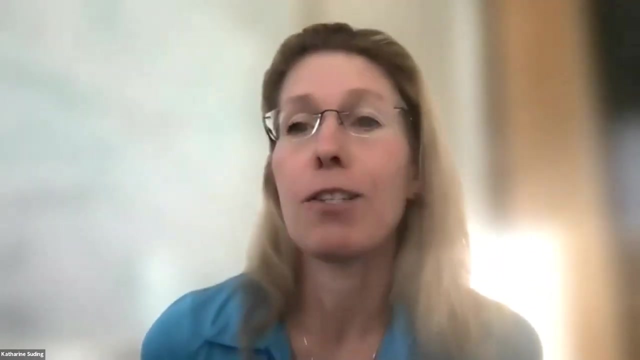 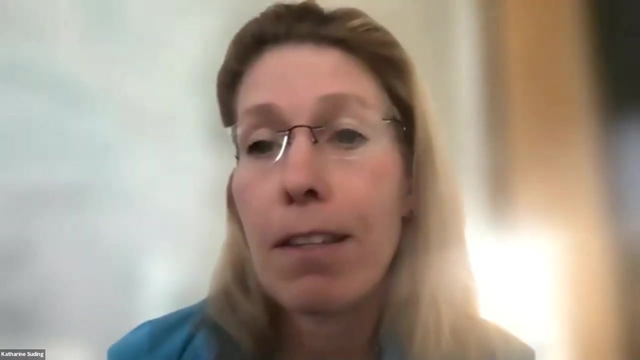 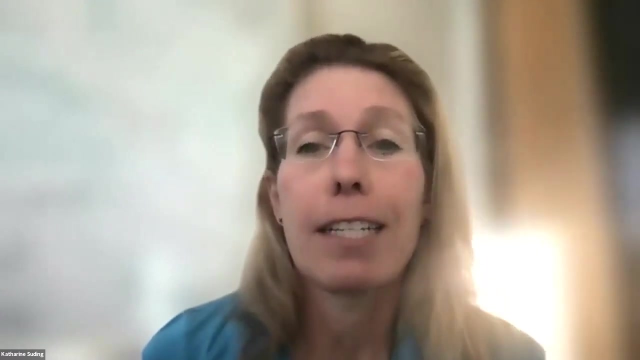 And we have. We're getting a lot of questions and I'd actually like to start with one myself, and then I'll try to get to as many of these questions as I can. They're just amazing thoughts coming from the audience. So what I am really interested to know from you. four: 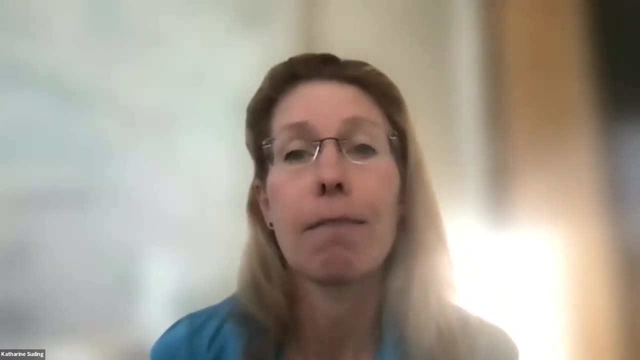 is just given where we are now and the amazing progress that's being made, and all the all the information that you're sharing with us, where do you think we will be in 10 years, Or where would you like us to be in 10 years? 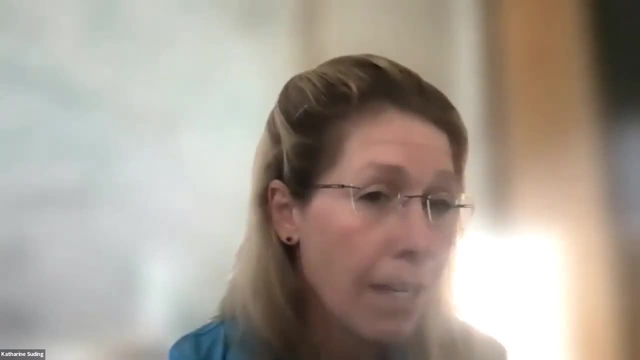 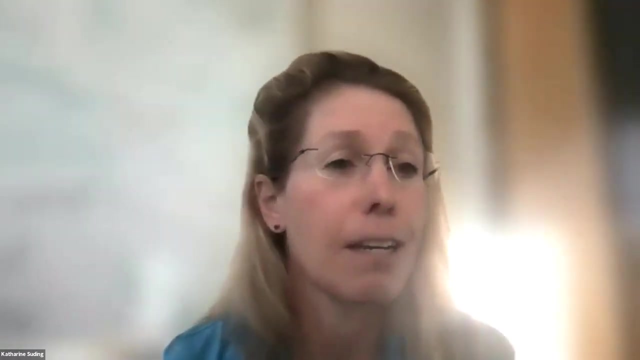 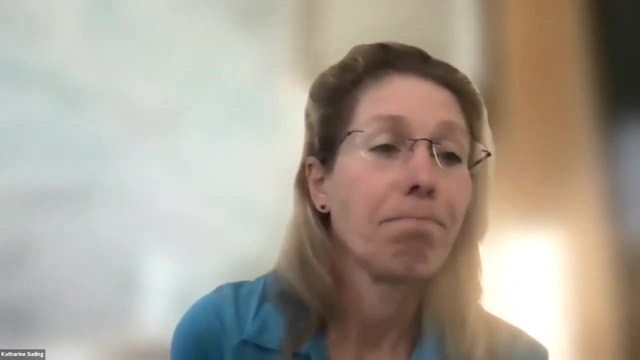 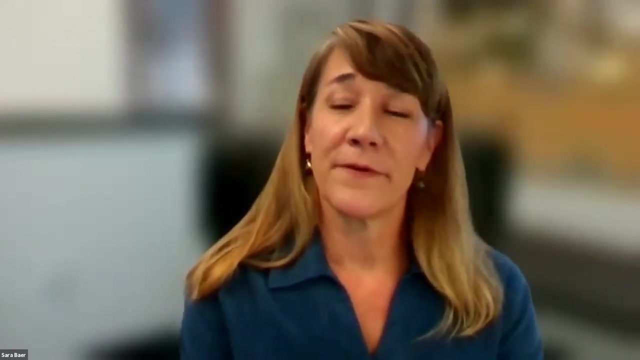 in terms of kind of incorporating soil biodiversity and soil processes in these grand kind of restoration challenges, And what are your thoughts on that? Thank you, Sarah. Thank you, Sarah. So I mean I'm hopeful that why I come from the grassland perspective. 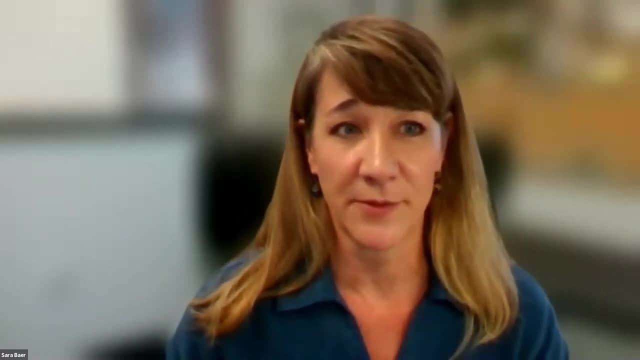 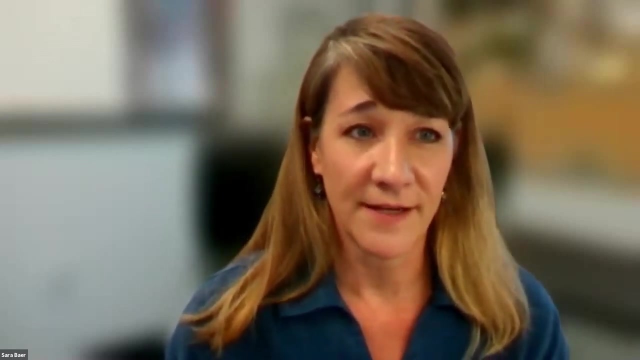 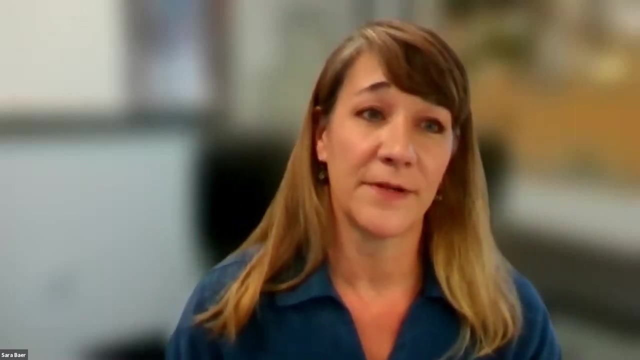 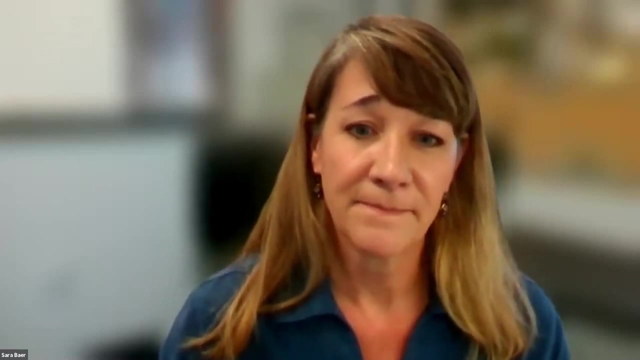 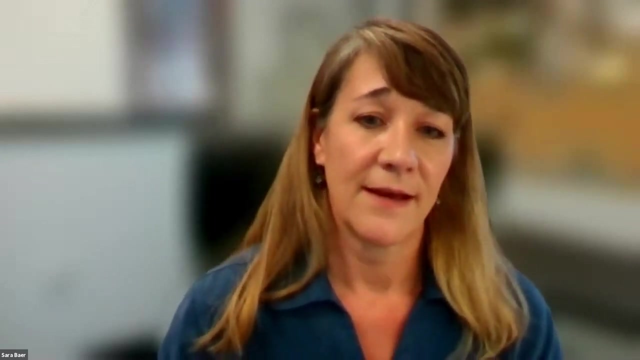 and agriculture is a major degrading influence on soil, but I think the more extreme climate events that we have will will will make producers- or I'm hopeful that it will result in a feeling of needing to be a better steward of land in regions that are resource scarce. 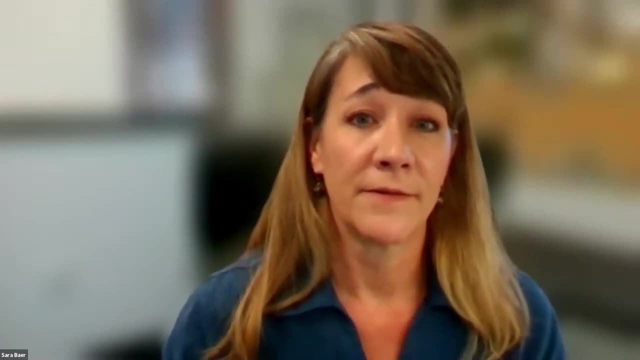 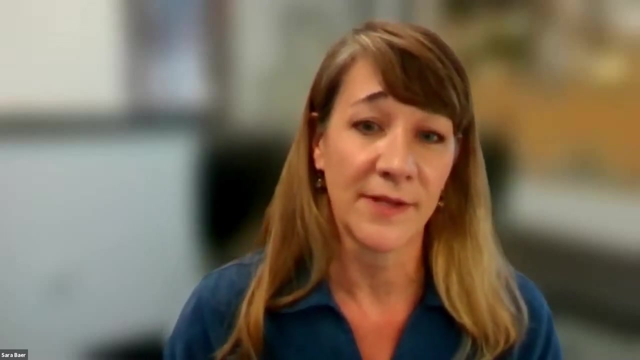 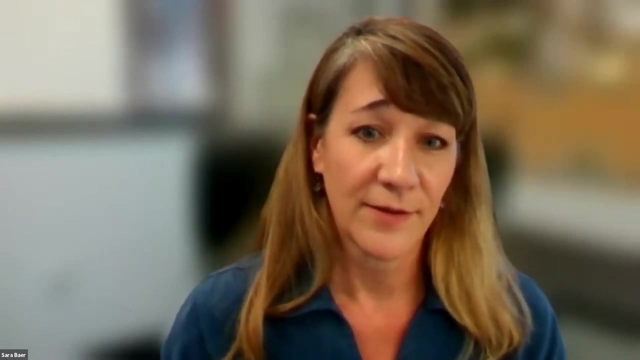 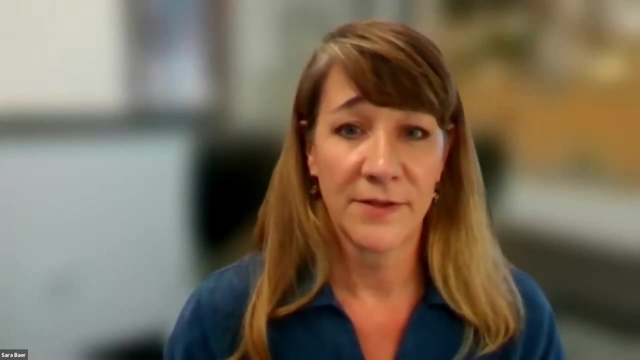 Growers are knowledgeable of soil, biota and aggregates and mycorrhizae. because the resources are so limited, So I actually think it might be sort of forced upon us, you know, collectively, through nature, And that force, I am hopeful, will result in a greater trend. 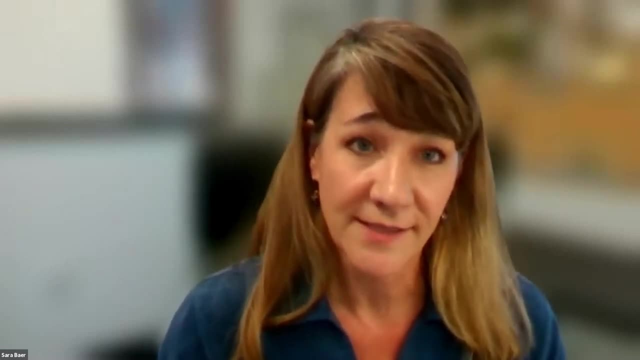 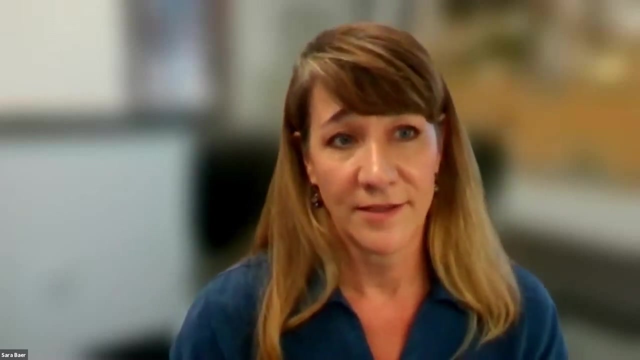 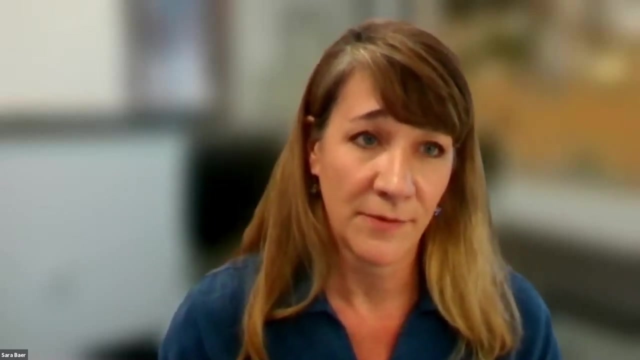 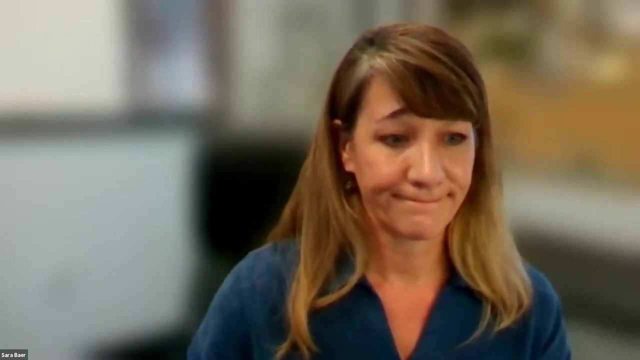 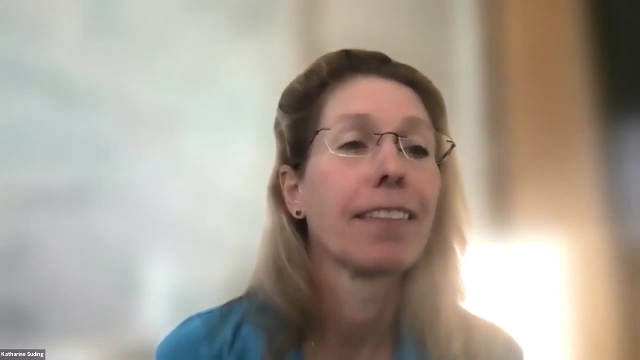 of using conservation practices in agriculture and conversion of a lot of marginal lands to grasslands, And I hope that this decade of a focus on ecological restoration will result in more incentives to do that. Awesome- Anyone else You know I mean. in my opinion. 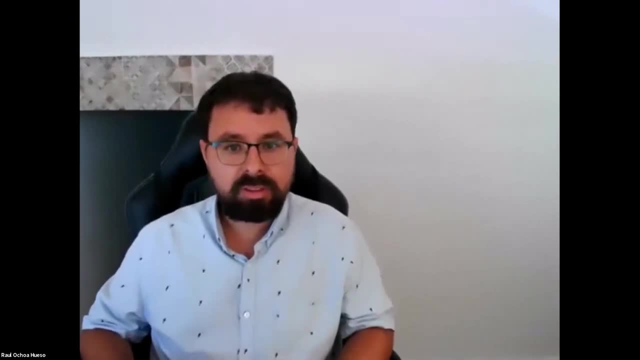 I would say that it's important to consider that somehow the energy is within right, So there's no alternative. There's no alternative to using the power of nature to drive the functioning of ecosystem, And the same happens if we want to regenerate. 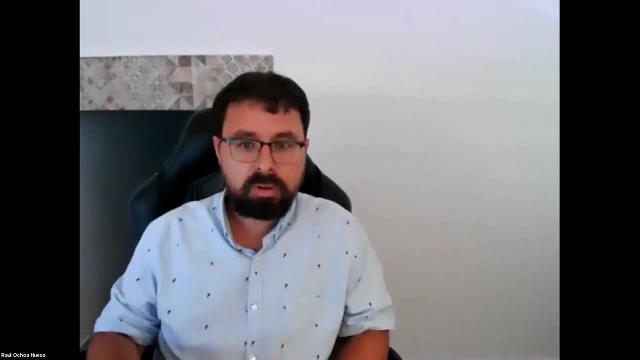 So I'm pretty positive that we will all realize that that is a- I mean, it's a universal truth, And many of us know that already is like our health depends on ourselves somehow, and how we manage our own lives, And the same happens with ecosystem. 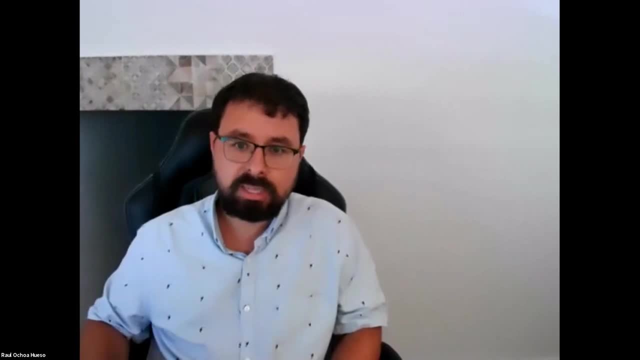 So, once we all realize that that's the way to go, That's the way to go, So we are going to move forward, that I think that the solution is at hand. Jesper, I think you were going to, yeah. 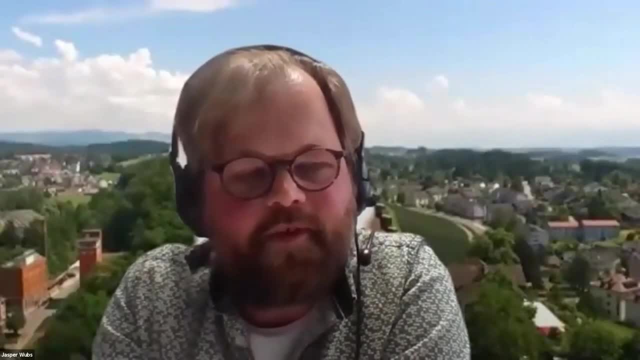 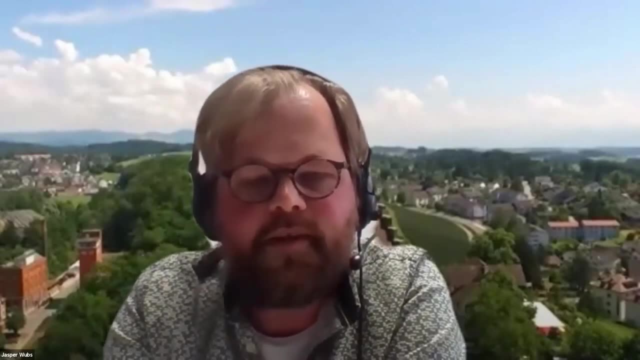 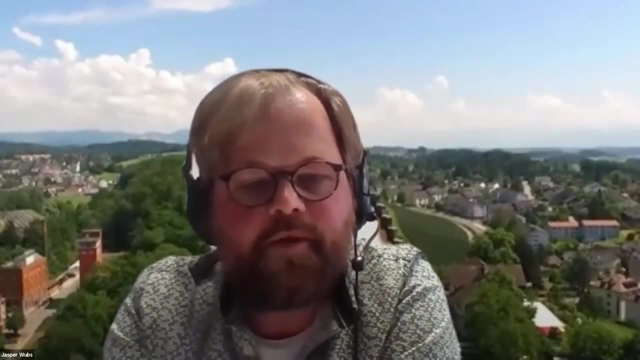 Yeah, sure, Yeah. I really love the points of Sarah and Raoul. I want to add to that a bit. I think there's a lot of momentum growing in different parts of society and, I guess, in society at large, about people realizing the value of biodiversity, of soul biodiversity. 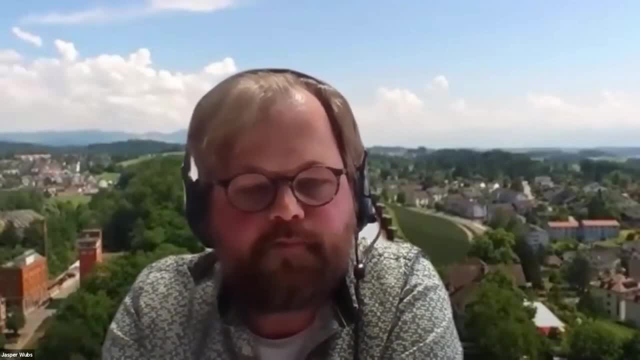 and of the need to restore ecosystems. So I'm very hopeful that that, indeed, this decade will bring a change. But I also think that we, as scientists, need to work hard to make sure that we bring all the evidence and all the data together, because it seems that, in many cases, blanket solutions 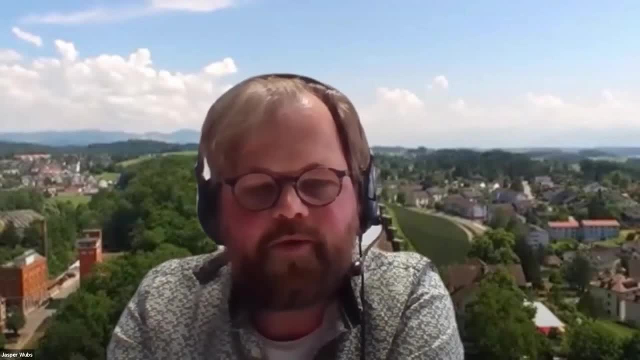 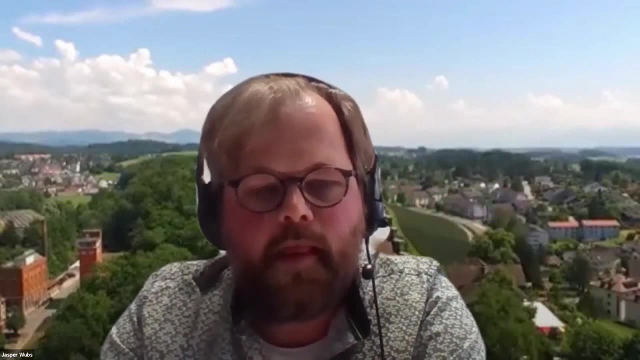 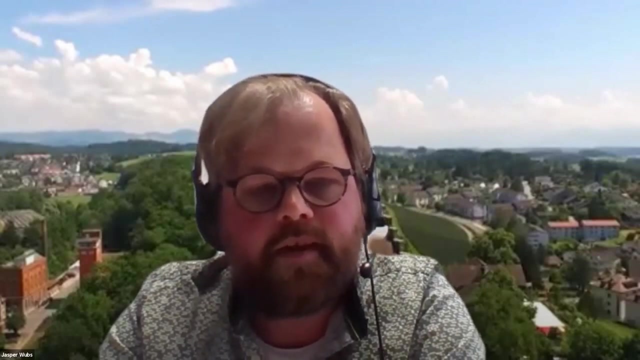 do not work everywhere, So we need to, you know, we need to untangle what is working, where and why, by bringing all that information And also bringing the socio-economic context into it, And I think that will be a major step for us to do in the coming years. 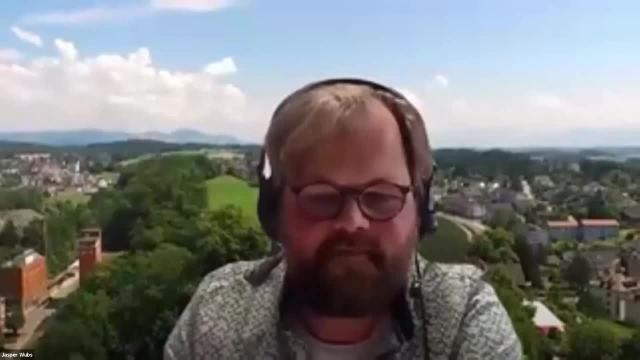 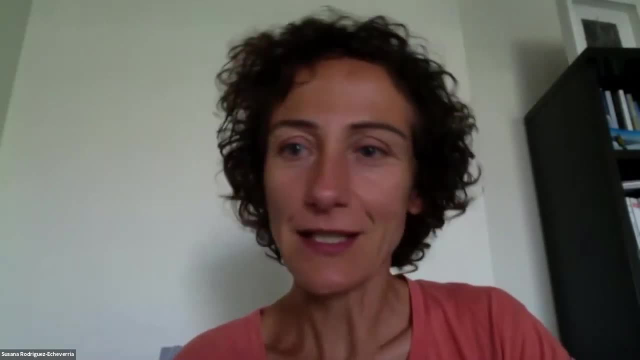 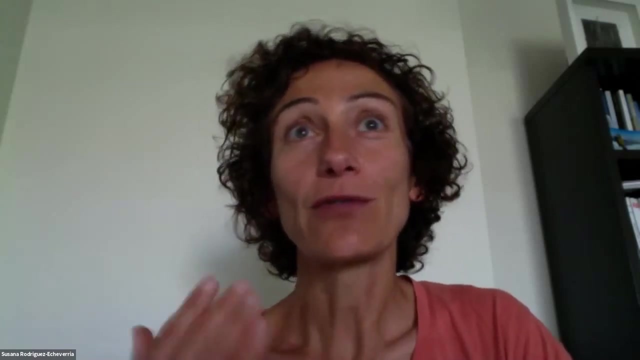 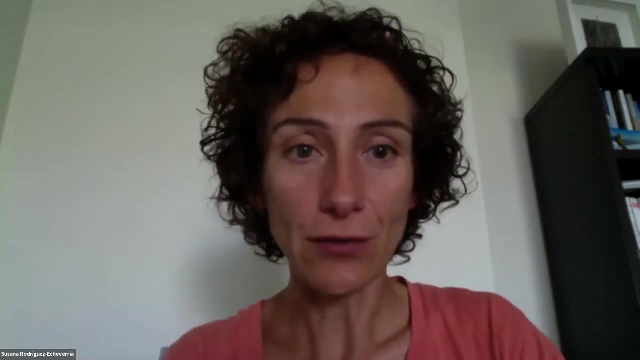 Excellent, I agree. Yes, I just wanted to add to what Sarah and Jesper said that I think is very interesting. I think that if we look from now to 10 years, we look from now to 10 years backwards. In the last 10 years there has been a very- I mean- the interest for soil and soil diversity. 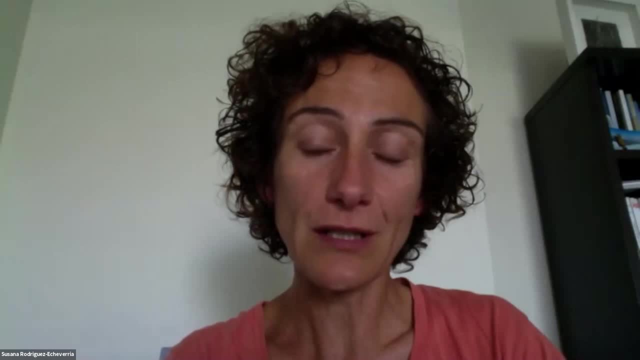 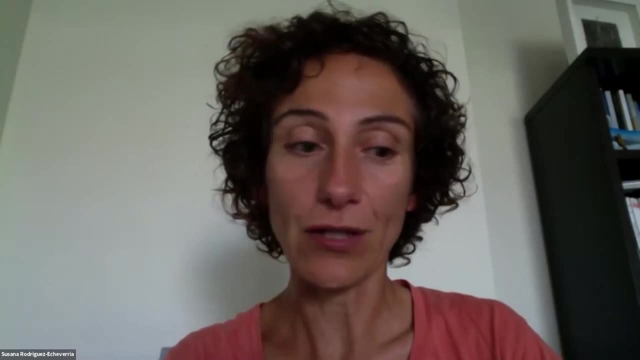 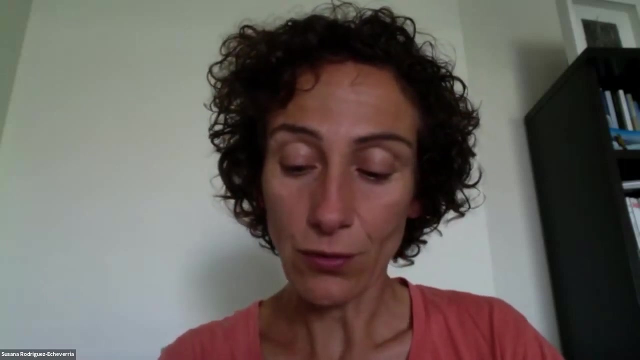 has grown a lot in the community of ecologists and restoration practices and also managers, And I think that is not going to stop. It is growing And I agree with Jesper that we need to make an effort to transmit all this information in a better way. 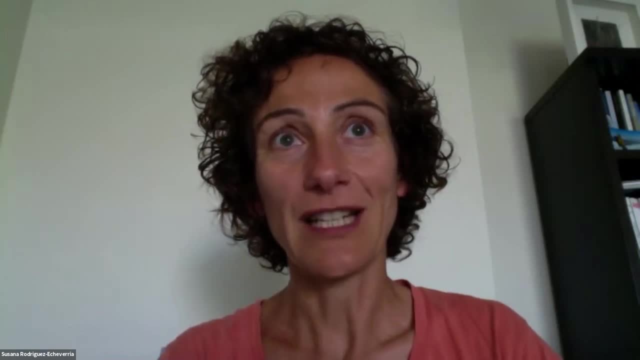 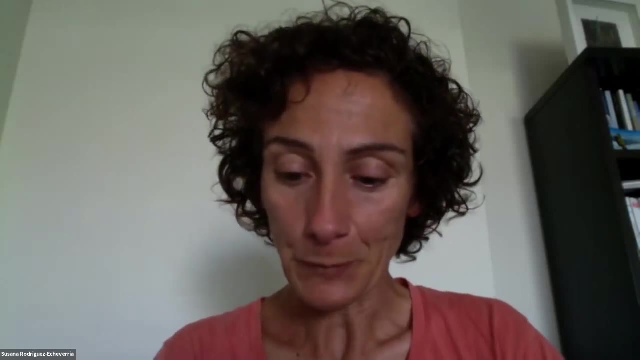 And to say: you know, we need to do this in a better way, that not like he was saying, that we don't have a unique solution for everything. i think that is very important because, um, when something is tried in one side or two sides and people doesn't see a 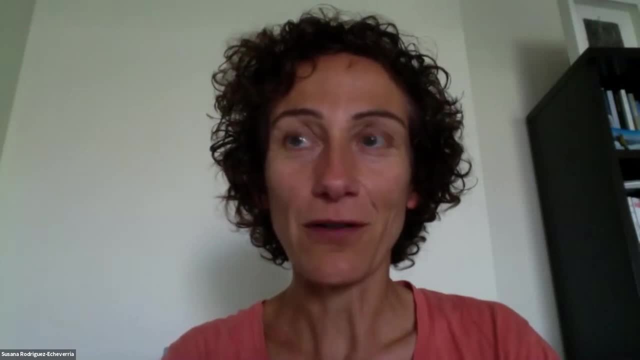 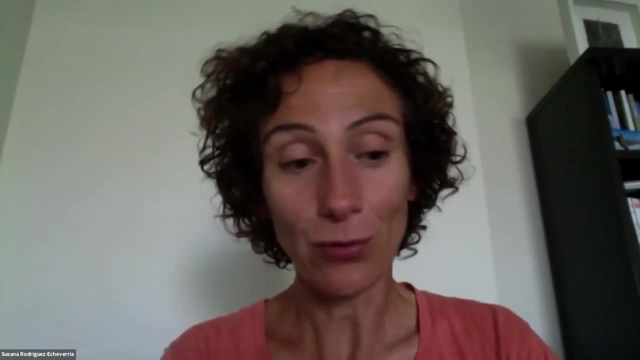 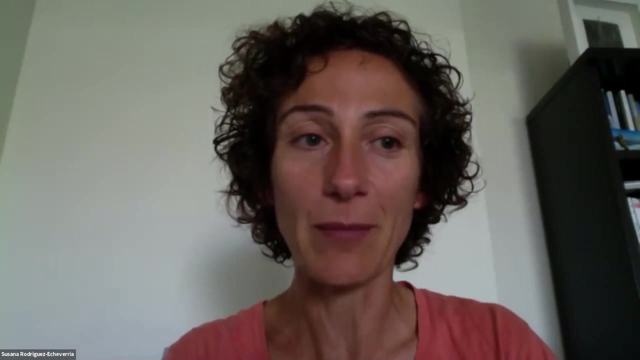 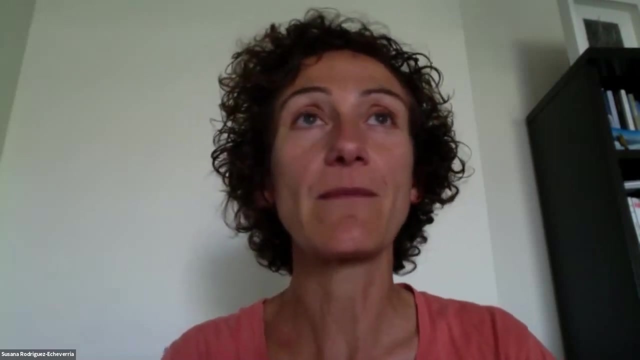 result, then it's very difficult to recover that confidence. so it's better to go with the information at first hand, um to, to, to try to to keep people interested in what we're doing and in how things can be done, and also, i think that many people is now at least in europe, or many people isn't- 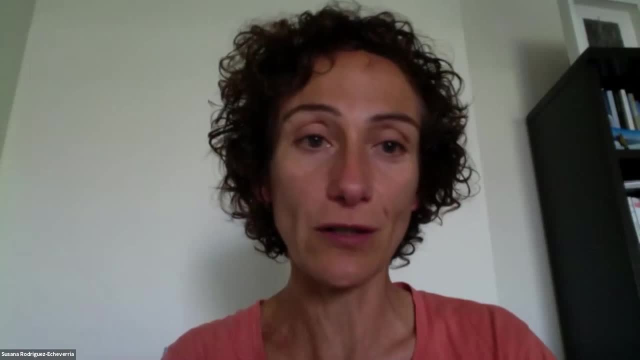 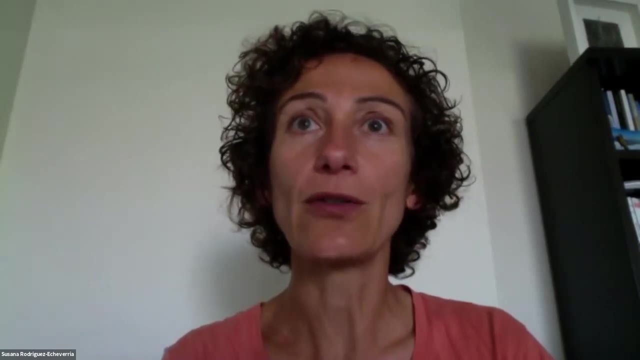 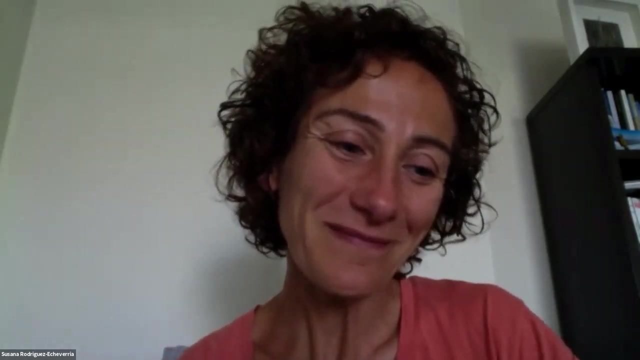 there is in close contact with land, like small agricultures or small farmers, are more interested in how the soil works, and bringing that knowledge into into management is a very interesting thing that's going to happen in the next years. great yeah, i think just paying attention to land is um is incredibly important um. 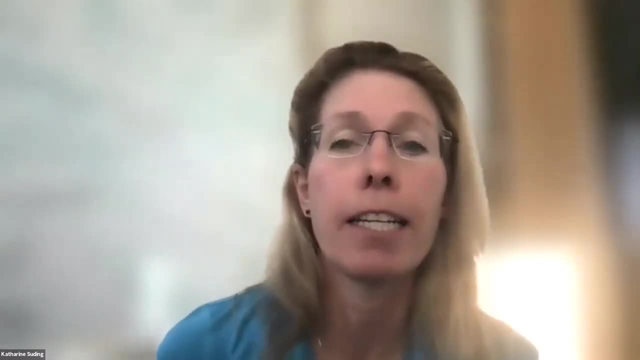 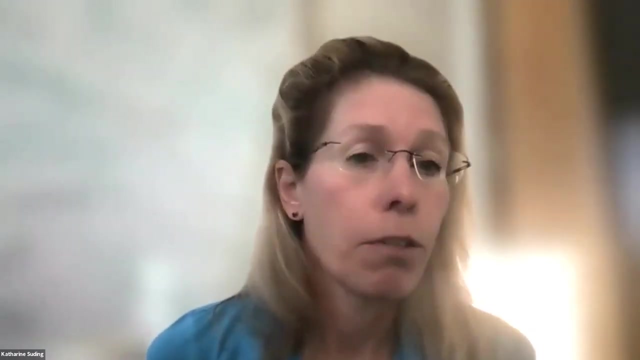 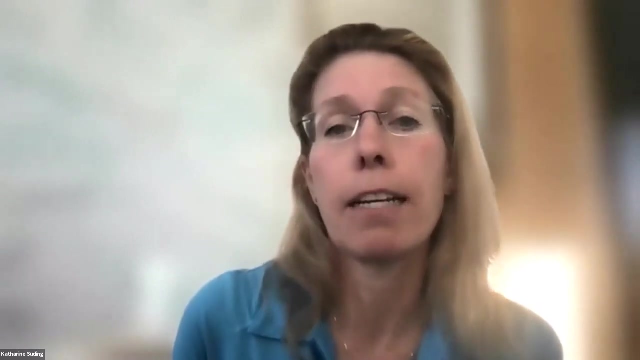 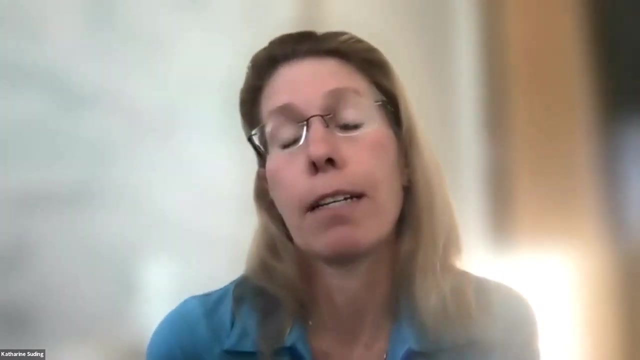 so there's been a lot of questions um from our audience about um kind of active interventions, interventions to address um soil- mostly soil- um micro microbial, um diversity and and processes um and so um, i just want to ask a couple questions from um, from thomas and francisco, and particularly 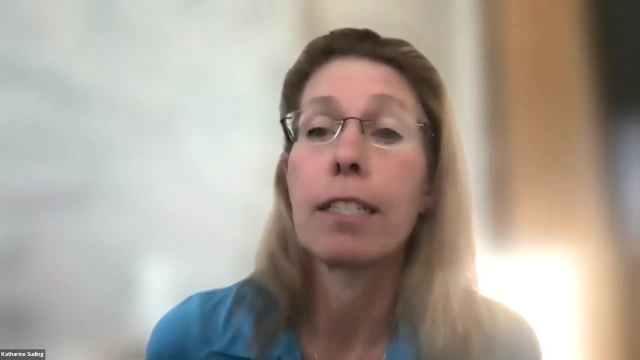 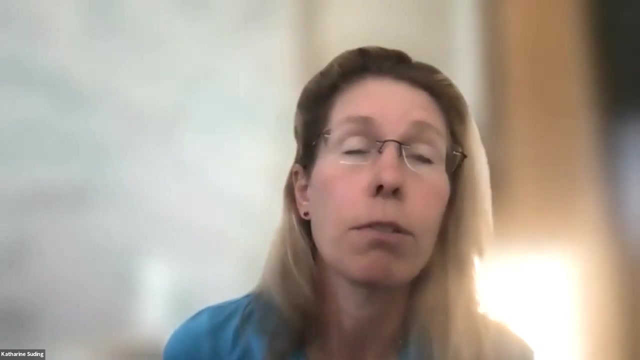 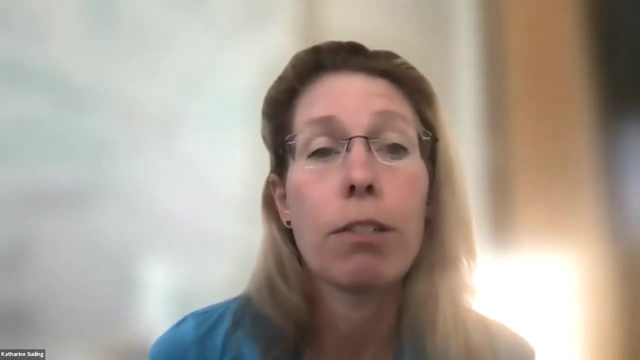 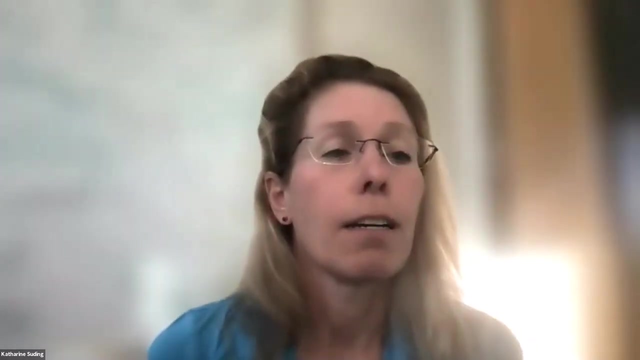 about kind of this active um restoration. so, um, first question is just one really general, is that that? is there a way to kind of uh address, if you want to do some active um restoration to address soil biodiversity, um, which groups would you address first um and how and how would you go about doing that? like is 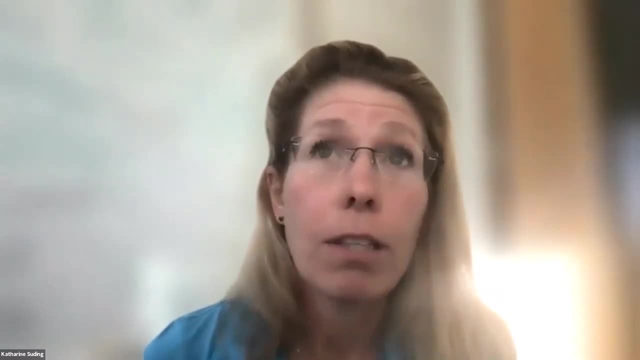 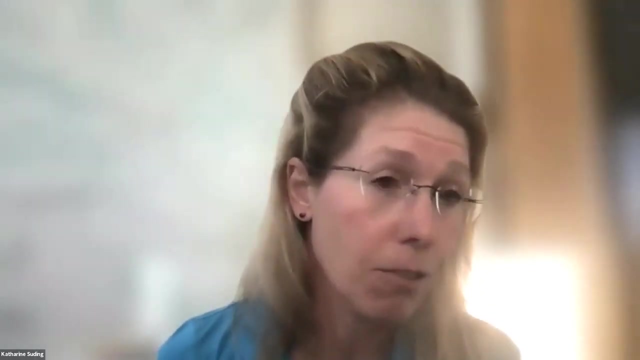 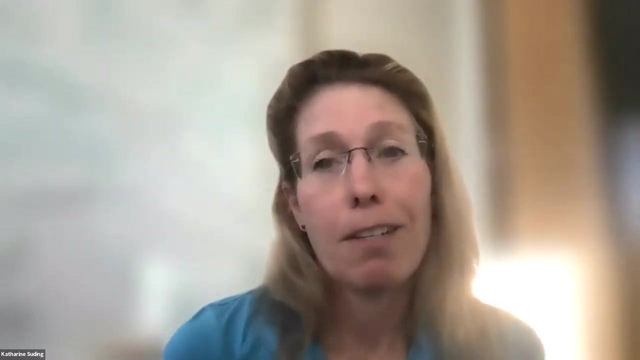 there particular um methods that you think are um, are particularly um promising. and i know, suzanna, i think we should probably start with you first, because you kind of start, talked about that most explicitly in your presentation, but i'm sure um um the rest of you all to have. have thoughts about that too. so well, um, from the point of view of course, all i mean, i will say that you need to restore the mutualist together with the plants. uh, because it's going to be very difficult if the soil is very degraded, it's going to be very difficult for most plants to establish and grow and reproduce. 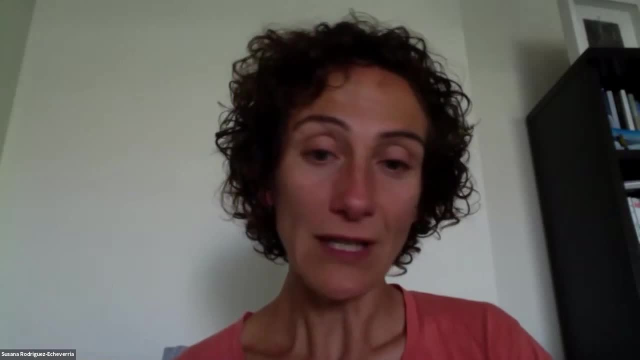 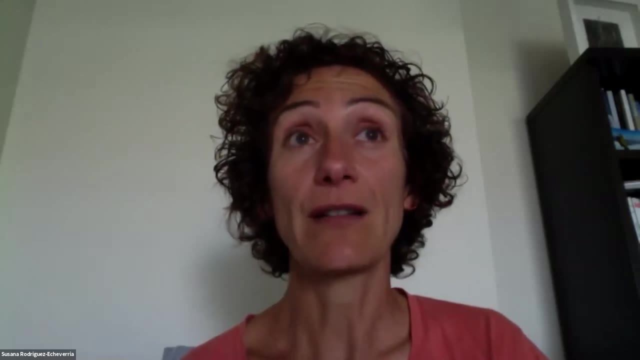 if they don't have their, their mutualist there, um, but also um, and you can try to do that, but i think fracas is also another way, but also if it's going to be very difficult to restore the soil, either um with uh, with the with theменal estás winder and e here i uh may address just with. 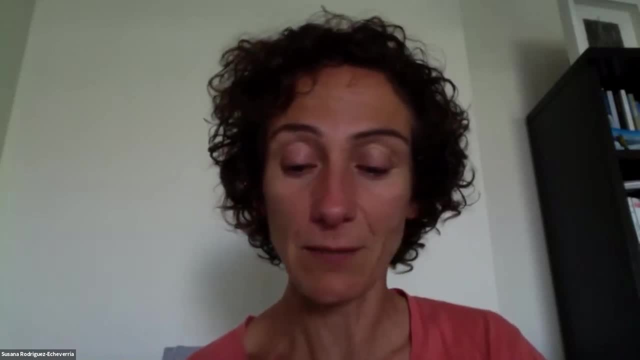 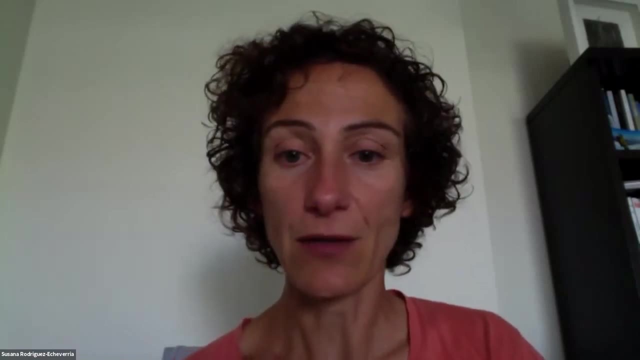 to try to do that by inoculating isolates. eh obtain from nearby ecosystems- like more reference to design tadi ecosystems, but also you can. what you can do is to use top soil transplants from nearby ecosystems and then you bring the whole soil community together and that will work much better because 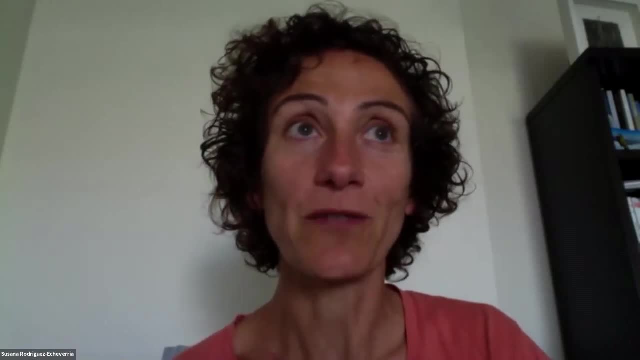 otherwise um is going to be very difficult to restore all the functions of the soil. but follow up you have- i mean i again- is one that that's a really good start. so i would would just like to you guys help me to try and provide um some umụr crush at the end. so, for example, if you have anything i'd like you to 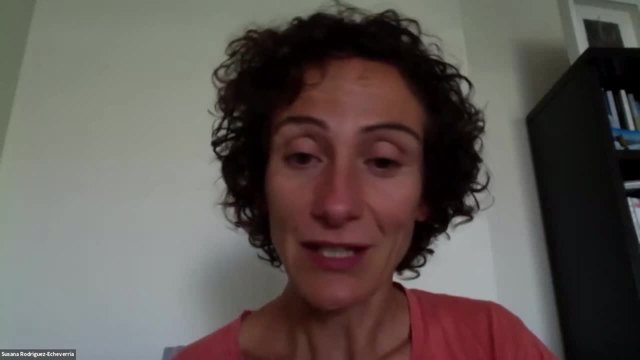 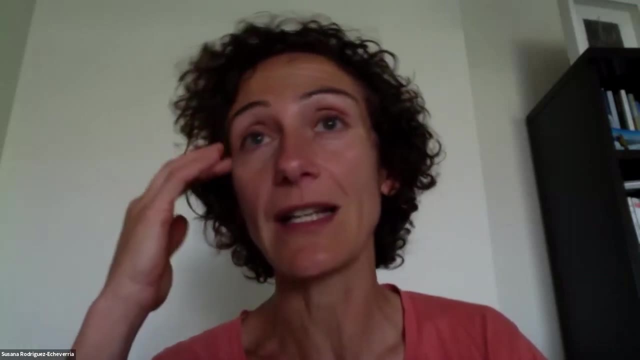 share this um because just niza reolia, no matter if this is a science or something, if you speak to us, um, there are super- is very dependent on the situation and which is the disturbance that is that happen in the soil and the current status of the soil. If your soil is totally degraded in physical terms, then you 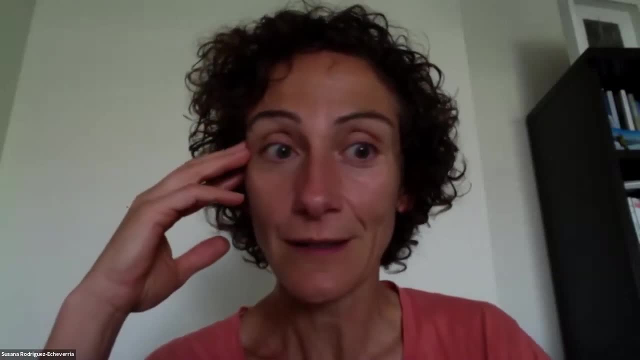 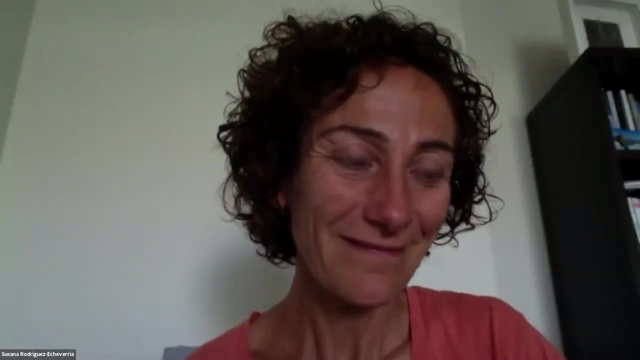 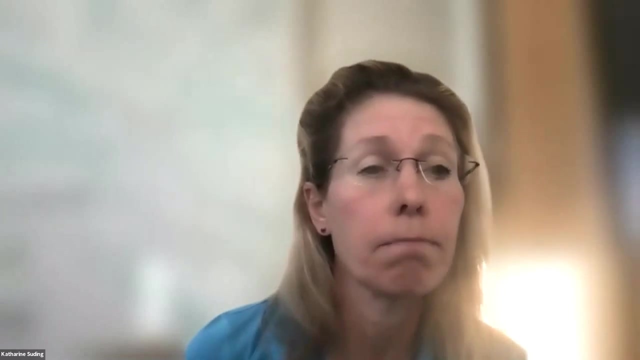 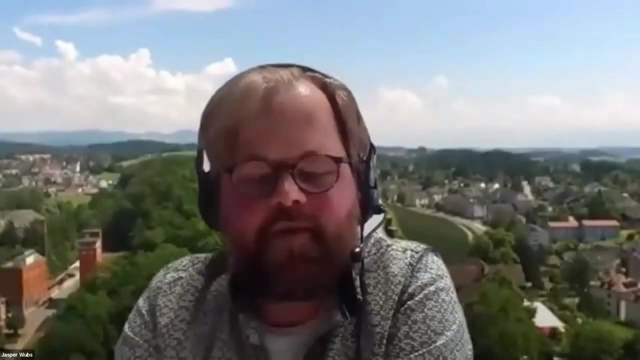 need to address that before you introduce anything. Great, Thank you, Susana. Anyone else have any ideas about how to approach active restoration to address the soil microbial community? Yeah, I don't know. It seems hard to give very general rules. I mean if indeed the soil is physically destroyed, you have hard-gaining microbial biomass, And restoring that basal biomass- the bacteria, the fungi- seems like a good first step. But of course you need active root exudation to keep these guys going as well. So you need to introduce the plants. 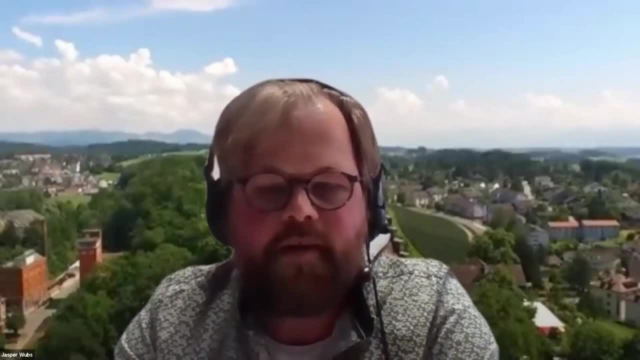 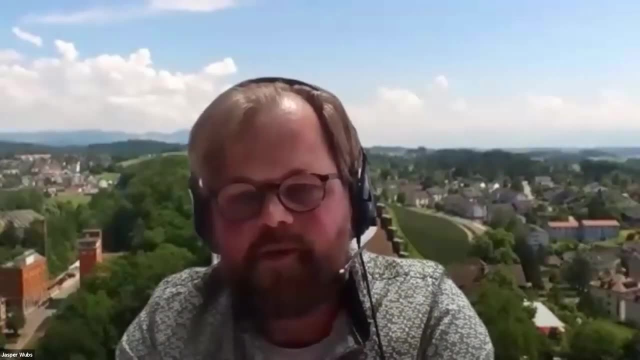 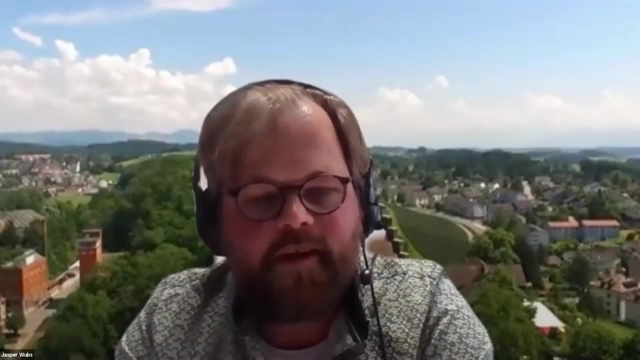 I guess at the same time There are more specific things that you could do. I guess, if your problems are not so big, If you have a problem with compaction or so, maybe you could do things with earthworms or stuff like that. But I think it really. depends on the type of degradation and where you're at what should be the focus, Raul? Yeah, so to me, one critical aspect would be to restore the aerobic decomposers, and particularly aerobic decomposers that simultaneously support the immune system. 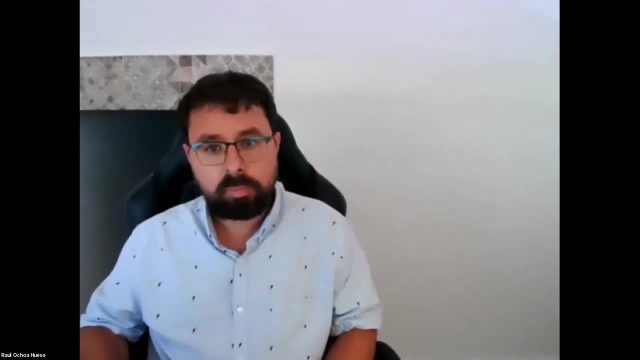 of the plants. For example, so many of these aerobic decomposers can also simultaneously produce vitamins and other components that are critical to the health of the plant. So if I have to make a guess or to propose something, I would say: let's go for phyla-like actinobacteria and 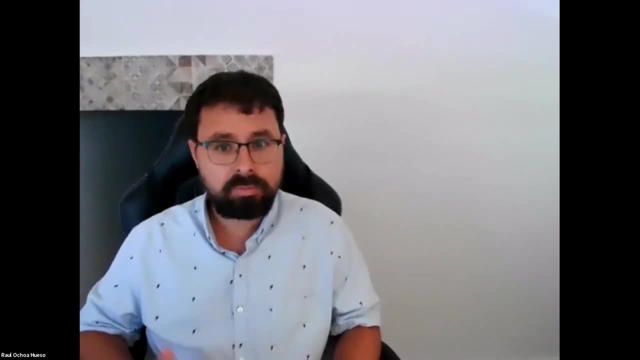 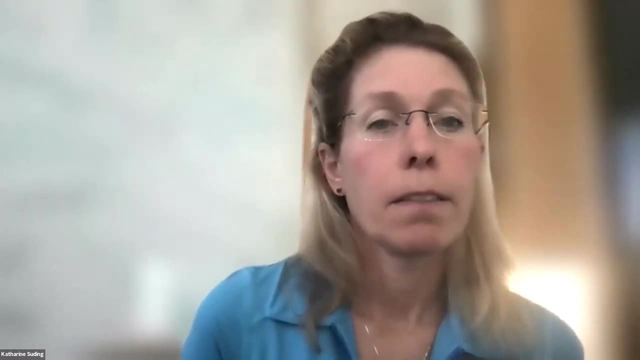 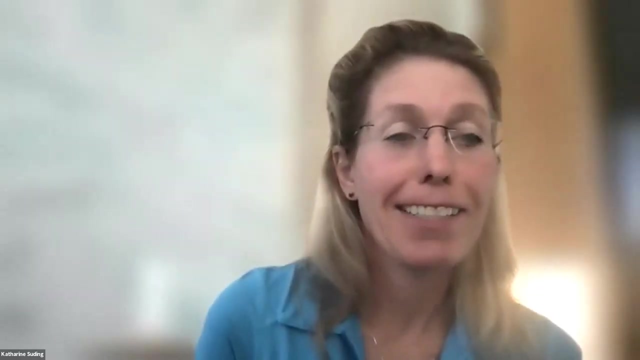 things like that. To me, those are critical to get the functioning. you know started Great. yeah, Sarah, do you have anything to add? Yeah, I wasn't sure where you were going. One by one, One by one. 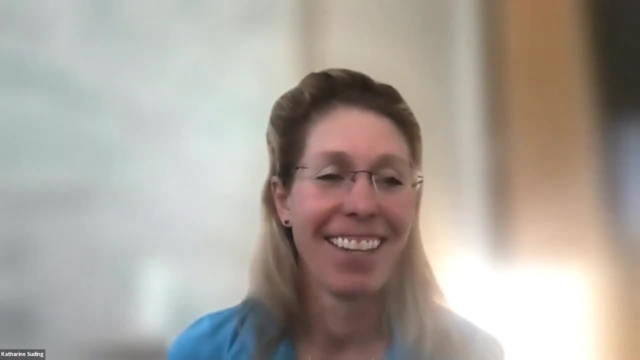 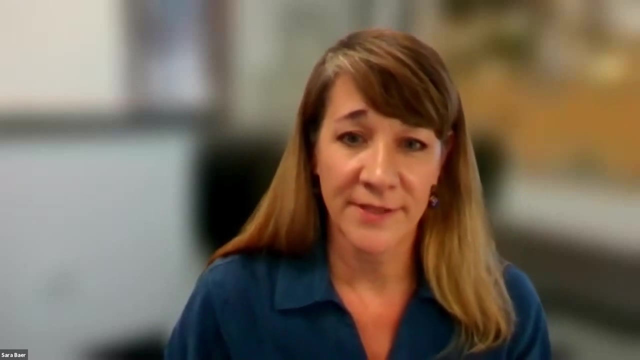 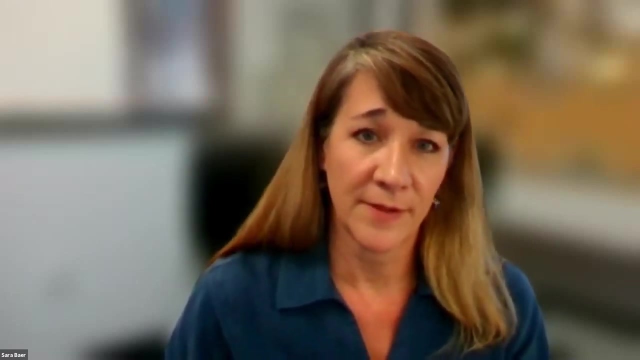 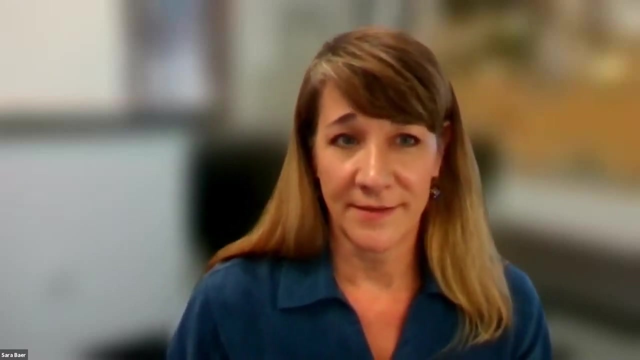 No, don't Just jump in. I mean, a lot of our work shows that there is a lot of recovery. that does occur naturally And I think imparting as much plant diversity in this system will help to blow ground diversity. But I think the answer to that question, at least in prairie systems and systems that I work in, 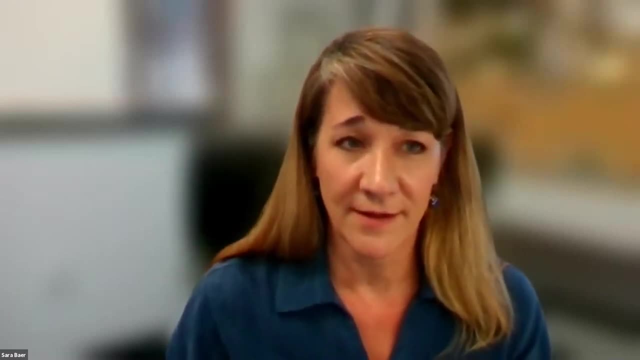 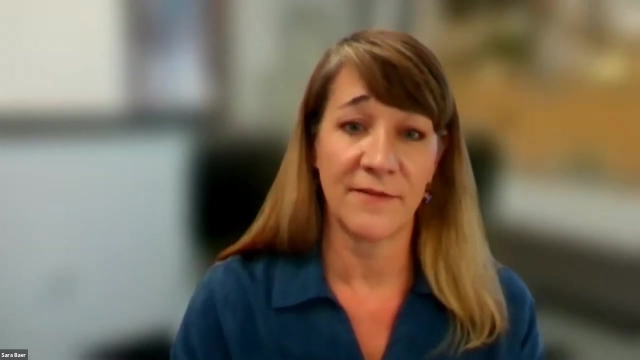 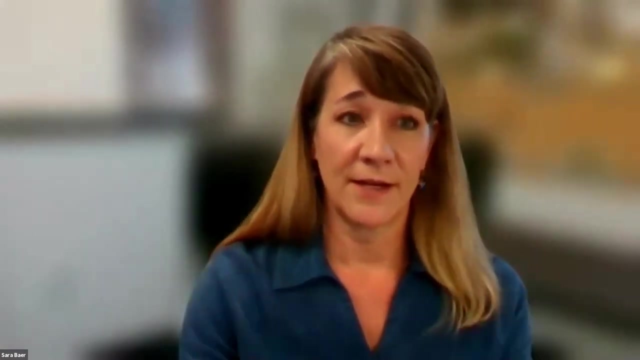 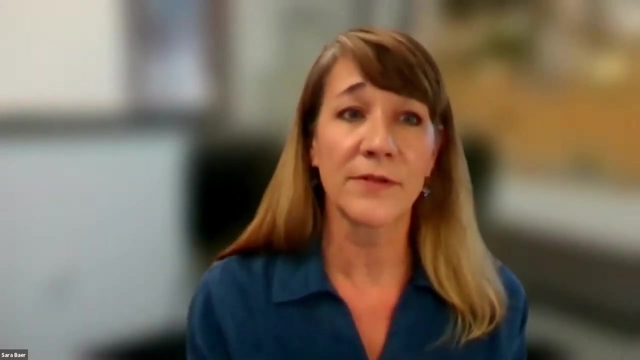 are forthcoming. We have a a project going on here in Kansas. A researcher at the biological survey has taken like blocks of native prairie, undisturbed prairie, that they have removed to build roads and then inoculated those blocks into an agricultural field to look at that dispersal. 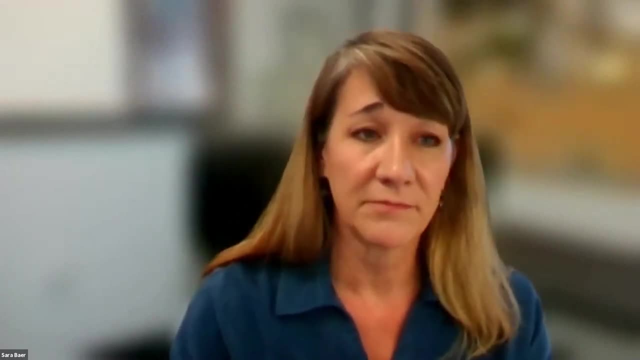 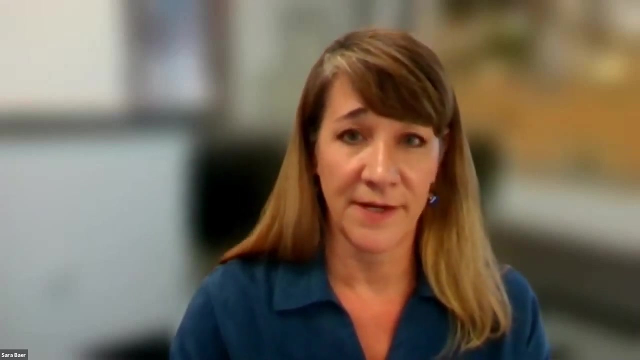 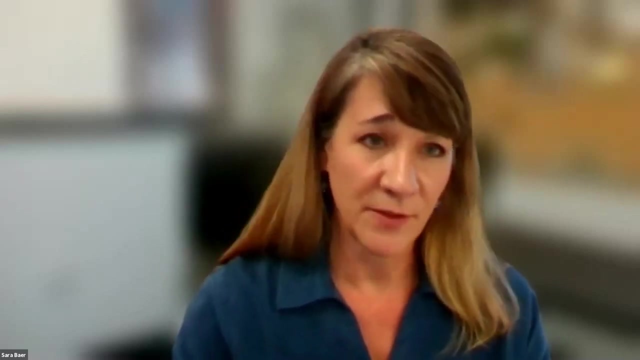 of the soil, microbial community fungi and bacteria, and then certainly there's a lot of research on very, very host specific mycorrhizae that do need to be cultured and need to be cultured on their living host plants and then and then using those. 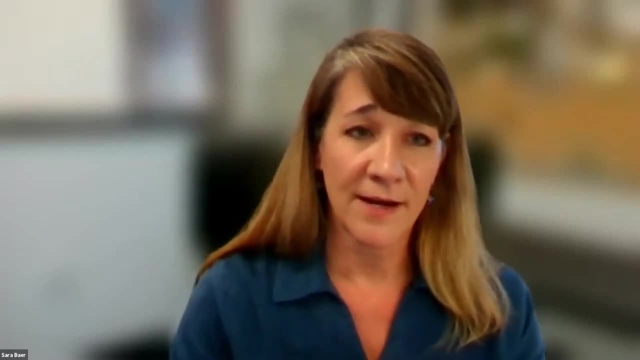 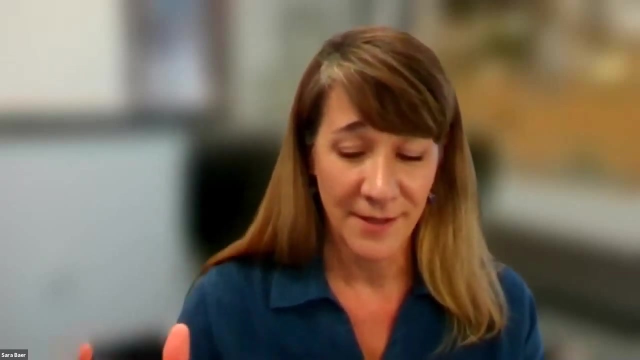 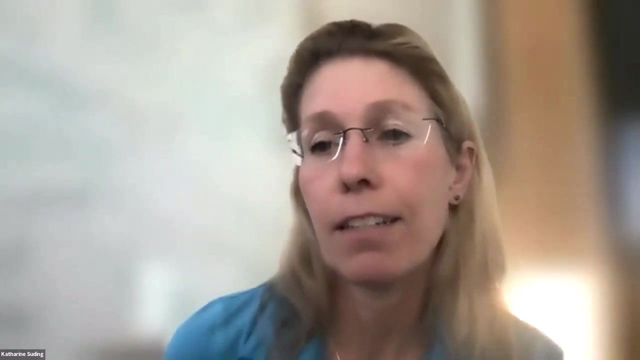 inocula or those potential plants. so I don't think, I don't think it's easy. you know, I think there's natural recovery, but if you really want to rapidly restore soil, microbial communities and diversities, it would take a lot of effort. and so I guess, just as a as a as a synopsis, I think that 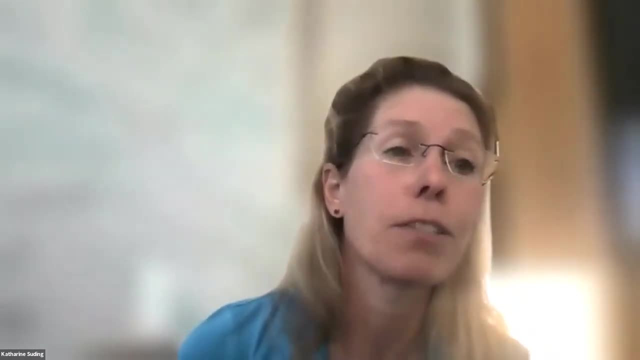 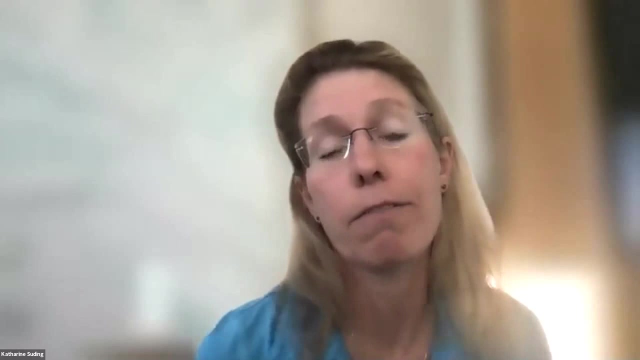 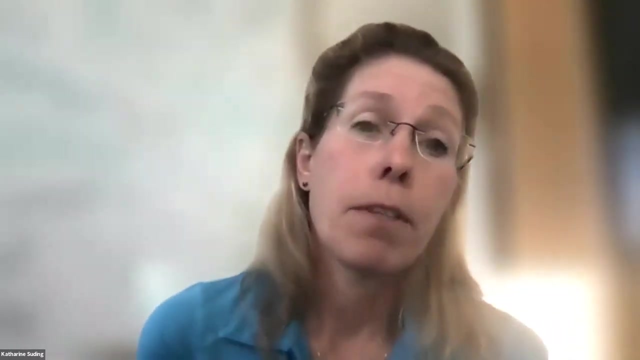 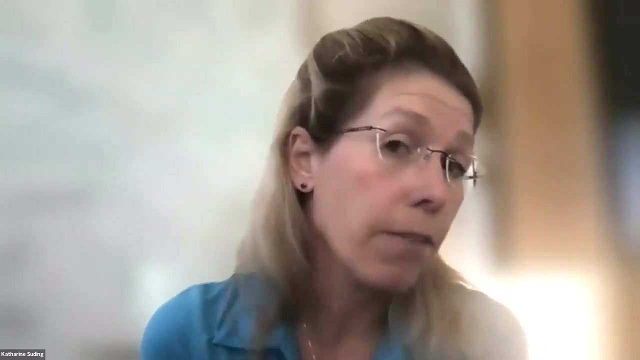 the idea is about kind of whole soil restoration and kind of trying to introduce the, the whole suite of soil biodiversity, back in the system as long, along with the other components that the, the soils couple with particularly plants, are probably essential. I have two really more specific questions that 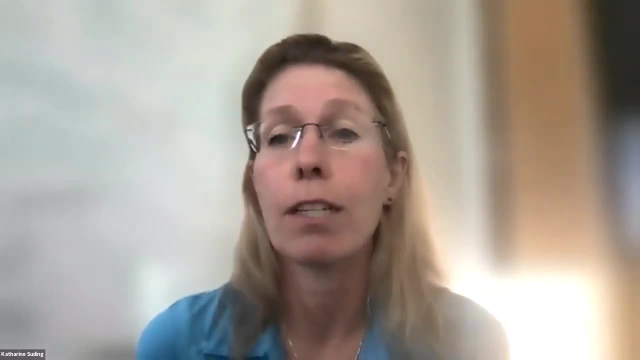 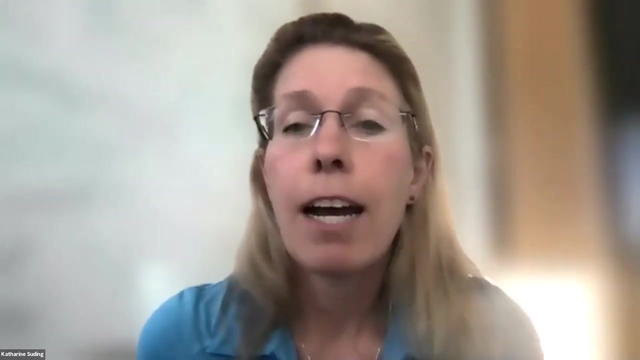 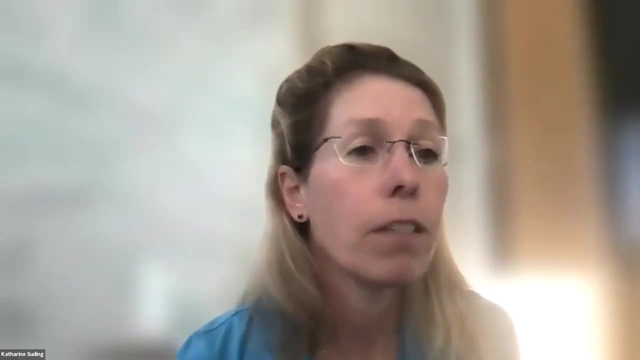 that that, I think, might be just helpful to address really quickly. first of all, there's a question about if you inoculate a system, how, how fast, how fast would you expect that inoculation to spread? you know, in terms of, in terms of affecting the, the, the whole, the whole. 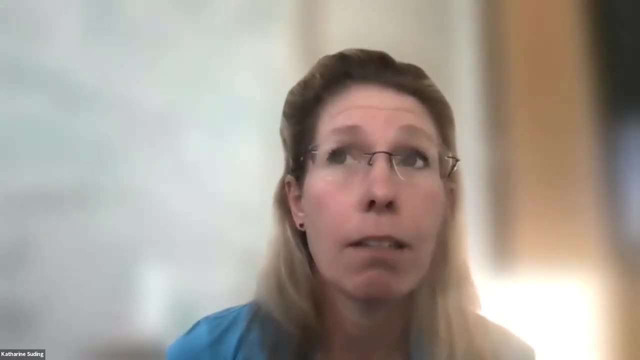 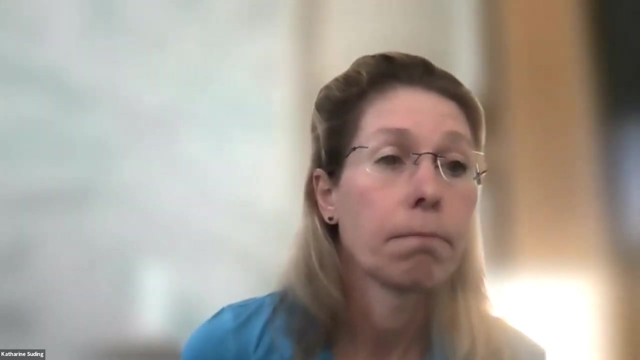 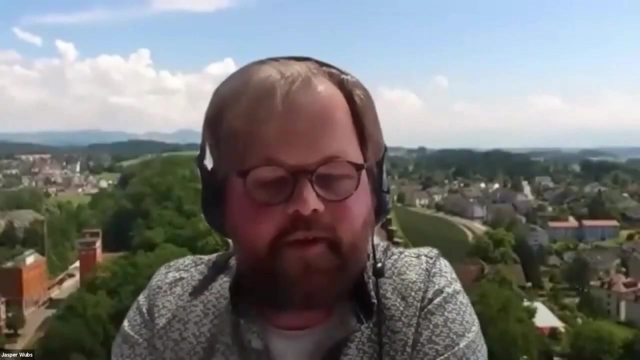 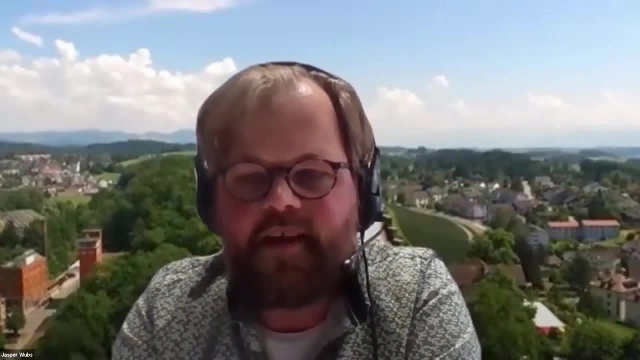 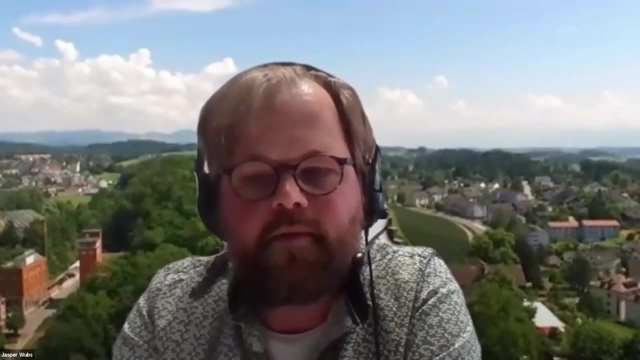 if you inoculate a patch it, it seems to pretty much stay there. it does spread a bit, I mean, but that's, we're talking meters at most. I would say: um, for many things. I mean there are papers that show that, that on the meter scale, you know, if you inoculate a mycorrhizae here, then the plant two. 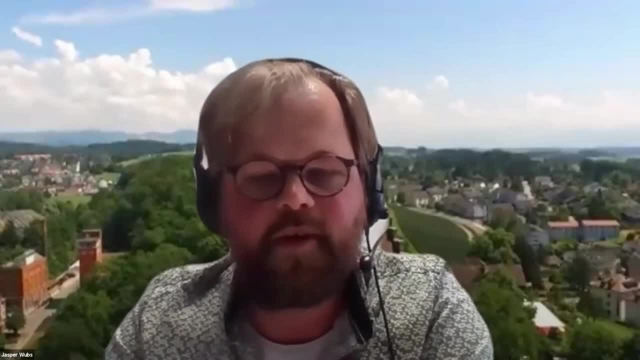 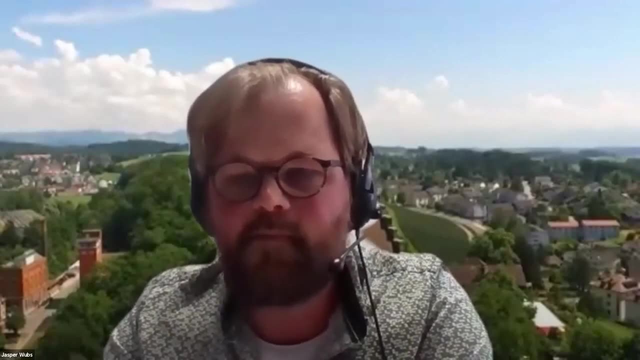 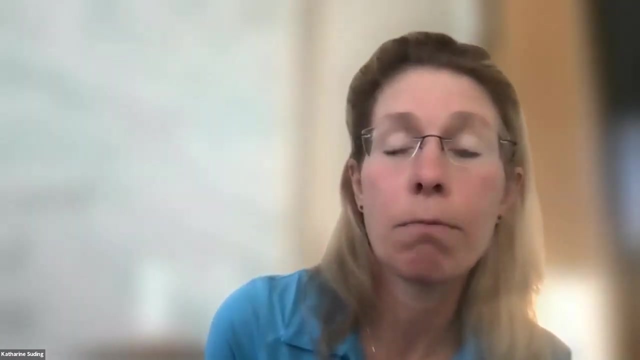 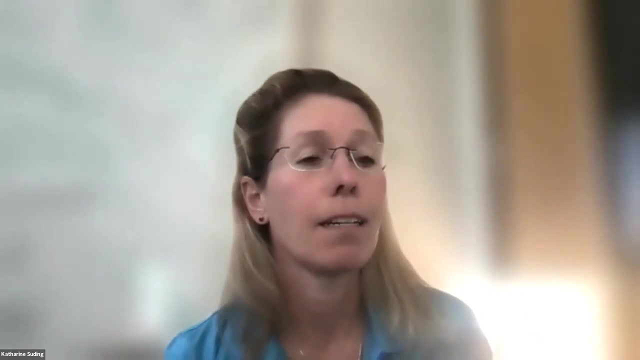 meters away, can, can, can respond to that, does respond to that positively, but I don't think it will be hundreds of meters in in in a few years, right? yeah, I think that. I think that inoculation is something that, even though a lot of microbial processes are fairly quick, related to plants. the spread of an inoculation is not necessarily. 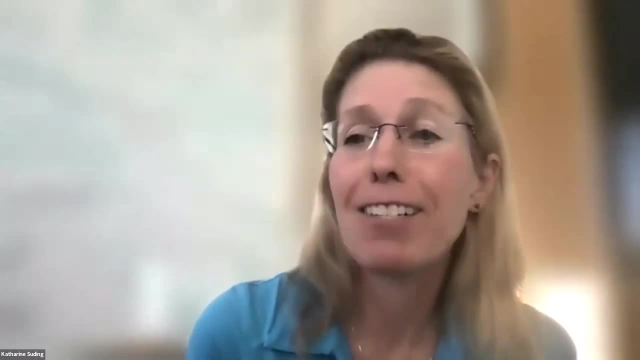 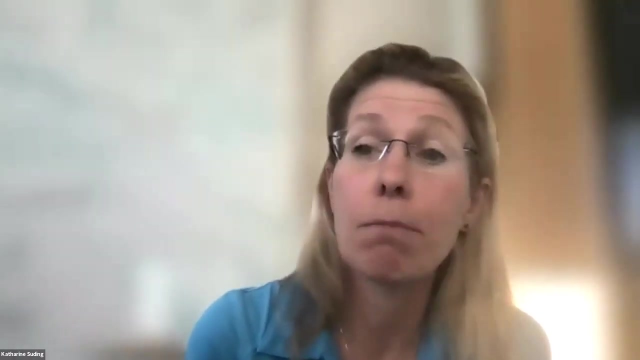 lightning fast and there's a lot of interactions there. I think that gets to Ryle's comments about coupling and decoupling right. you have a system that's in place, that could be degraded but could be really resilient to the interventions that you're trying to. 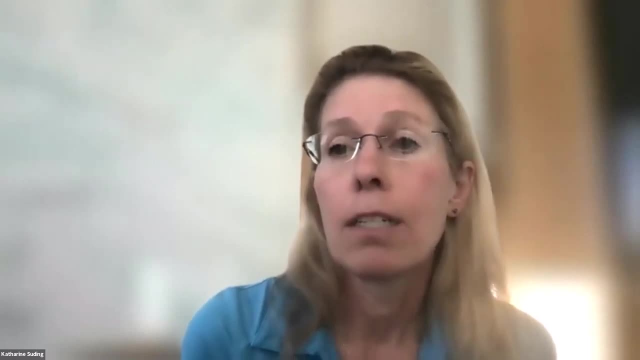 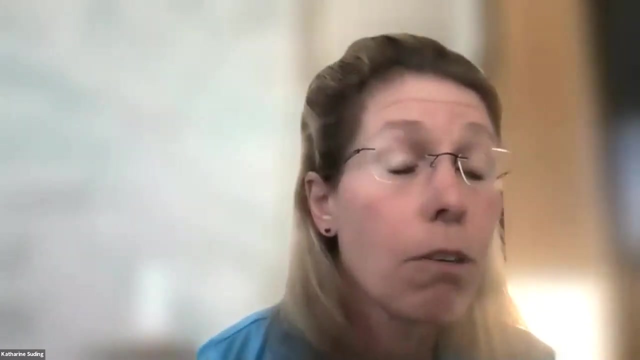 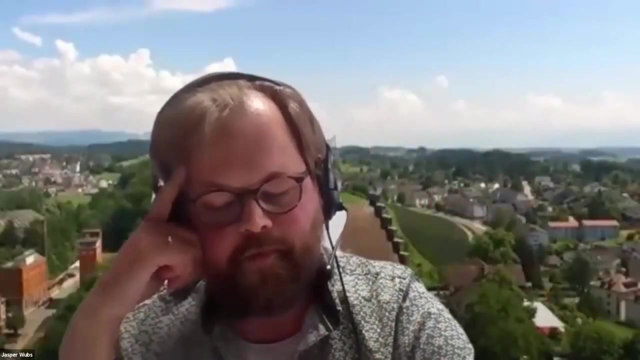 um to apply. so I wouldn't expect um necessarily that that process is quick or easy, even if you add the, the right um or the organisms that you desire. yeah, Jasper, yeah, just one one thing to add: maybe, and this is something I wonder, I mean, a lot of the research on this seems to be done in flat places, so 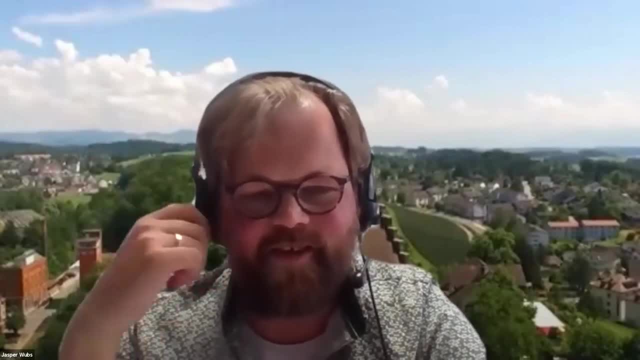 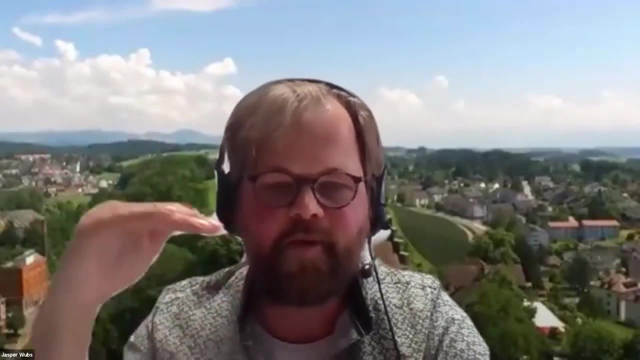 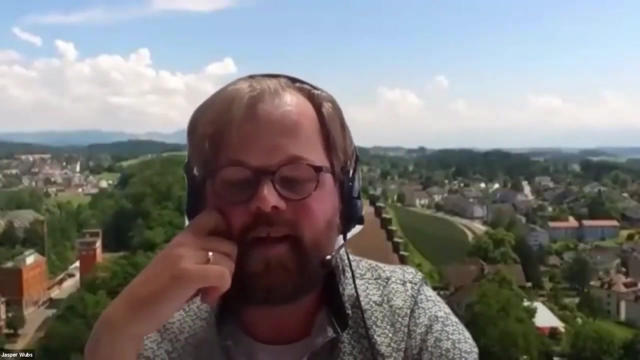 the Netherlands obviously qualifies as a flat place the the Midwest in the US as well, and there I guess most of the water flow is is is vertical down the profile. so I wonder if you, if you're on more sloping terrain, if the, if the spread rates going down are better? but I don't know if that's the case, but I think I mean it's. 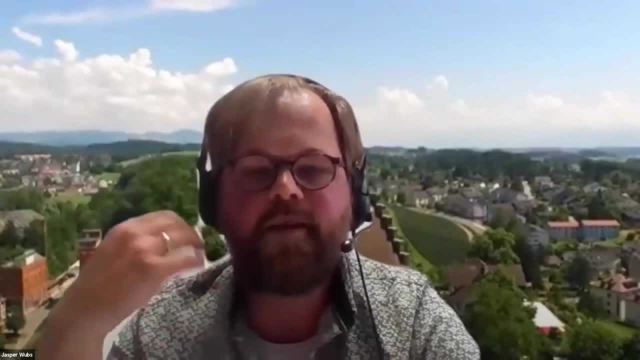 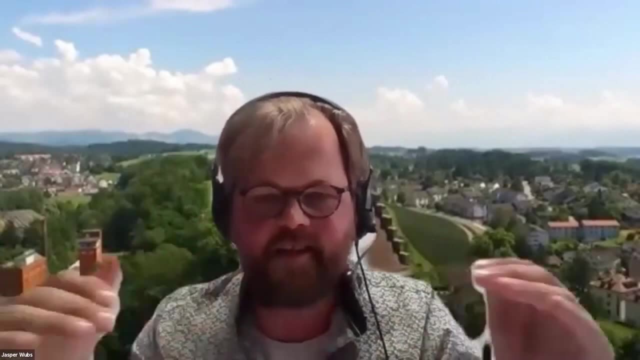 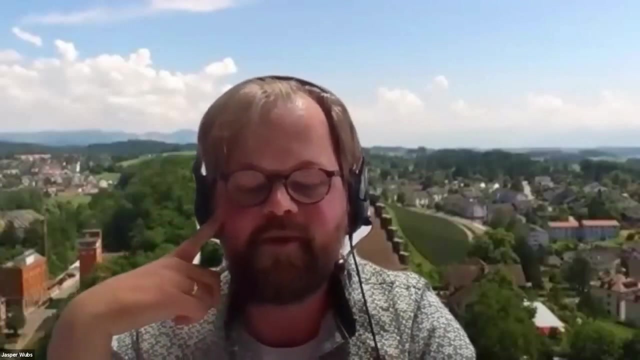 it seems to me that there's a mass action effect. uh, you know, you need sufficient numbers of microbes to really transition a system, um, and this doesn't seem to be happening in in a flat place. uh, you know, going going horizontally, but maybe if the, if the water flow is more lateral on average. 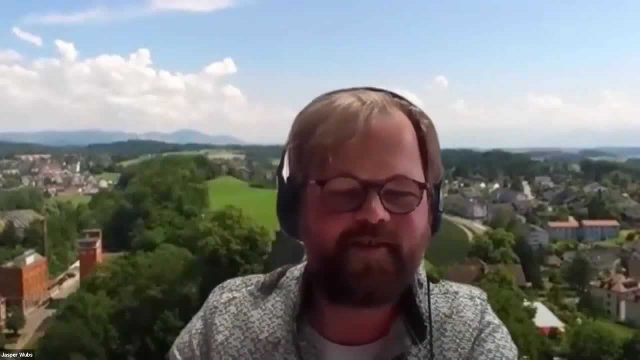 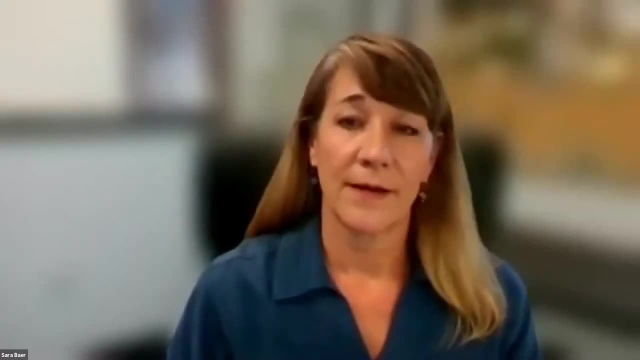 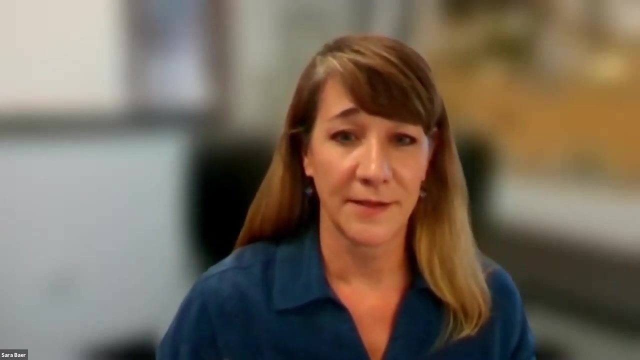 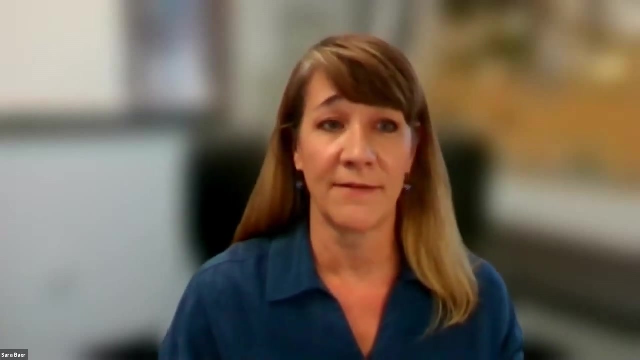 um, maybe that would help. I don't know if others have thoughts, Sarah, do you have any? um thoughts about that? so, uh, I often wonder if, if the, the stage of restoration matters, you know is, is inoculating at the onset, would you have, you know, no aggregate structure in a severely degraded situation? you? 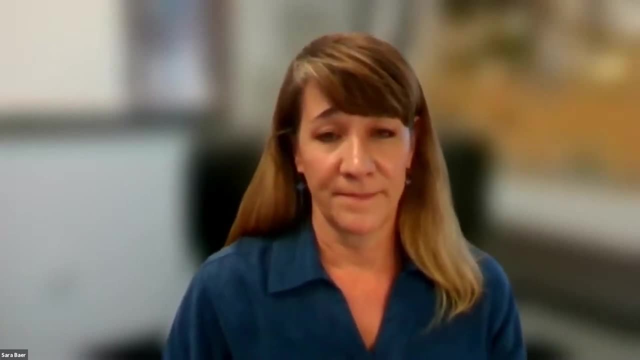 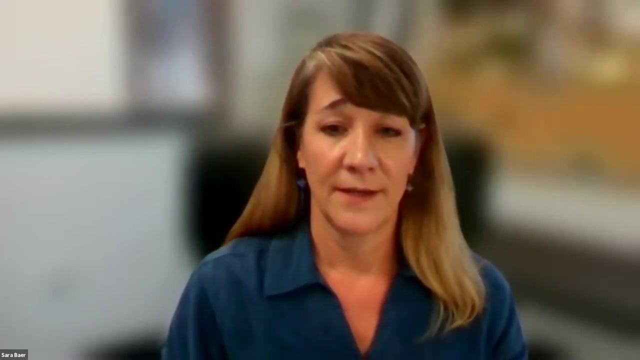 might have high levels of nutrients. um, you know extreme wet, dry conditions. I don't think we have a good sense of you know when. when is the best time really to intervene if we, if we can restore some of the plants and some of the function, um, and let the 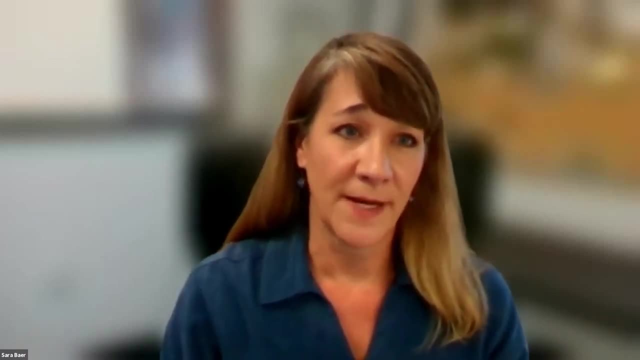 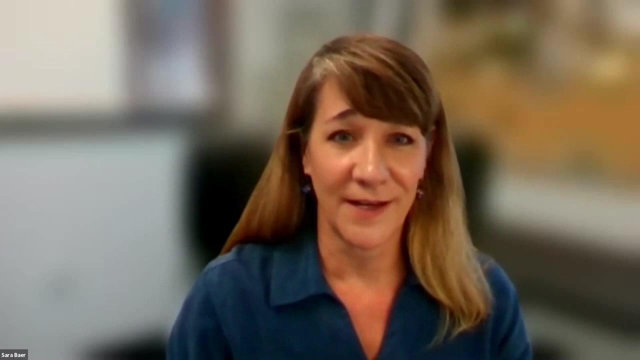 ecosystem and facilitate the recovery. you know when would be the best time to to inoculate, uh, the soils? I just don't think. I don't know if we know, I don't know if any of you have have seen any research on that, but we, we have a tendency to want to go in with. 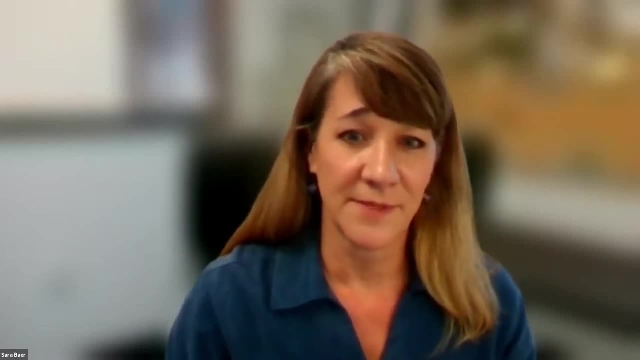 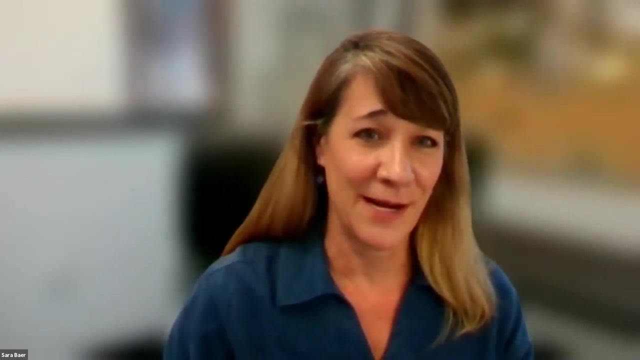 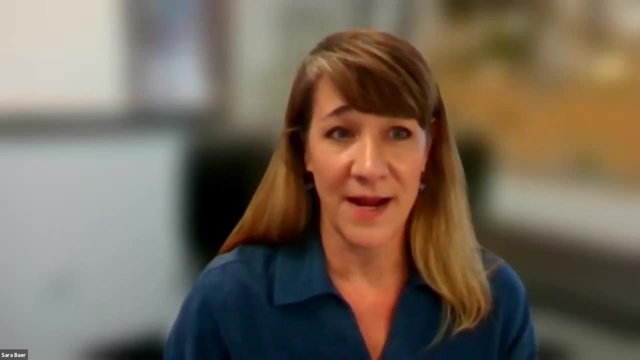 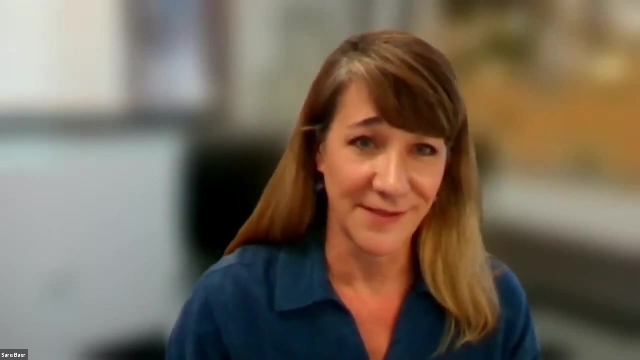 privacy and and see Grand change over short time scales, and that might not be realistic and I, and I want to give a shout out to Jasper because, um, his daughter Phyllis, the philosophy that we can repair everything can be dangerous, you know, because it can undermine conservation efforts and uh, 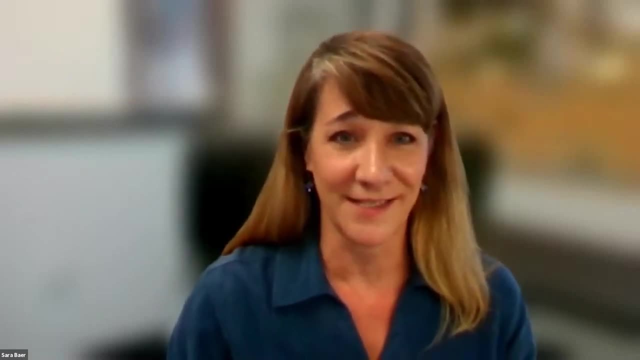 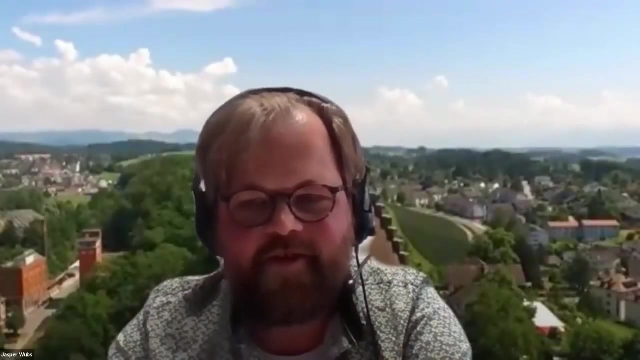 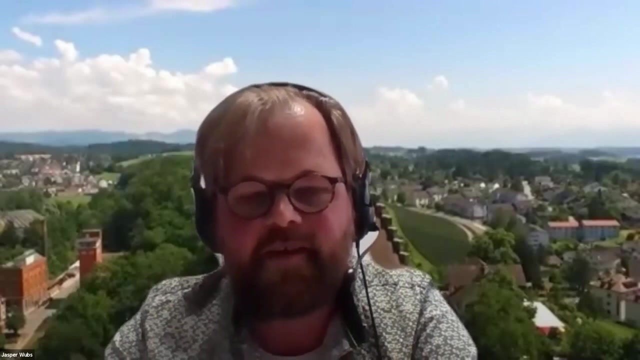 I smiled because when I teach my restoration ecology class, that is the paper we open up with. yeah, i fully agree with that. i think rule number one in restoration ecology should be: should be: keep what you have, you know, try, try to stick with the ecosystem that are still looking okay, try to maintain those. that is the best we're, we're. 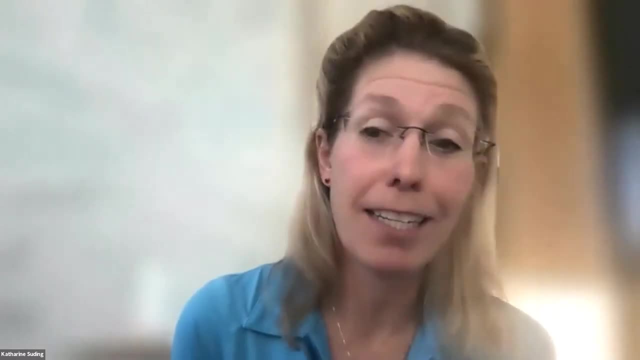 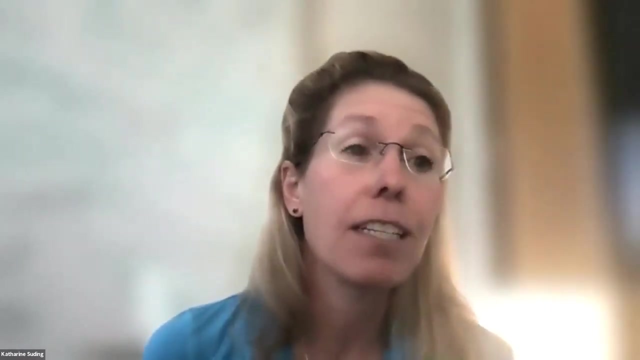 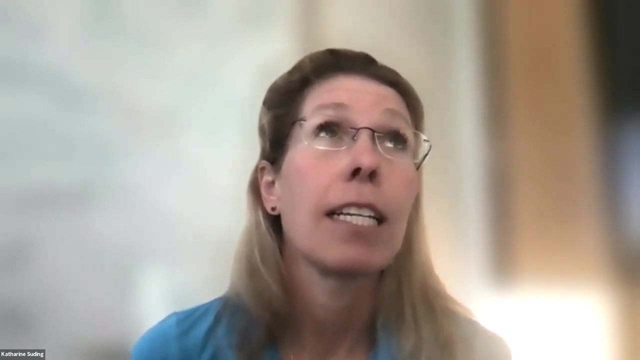 we're getting at the moment right- and have humility right- that you can't um, you can't drive everything um rio. i wondered if you could just jump in a little bit about um, thinking about these processes, and how would you take a system that is decoupled or maybe even anti-coupled and 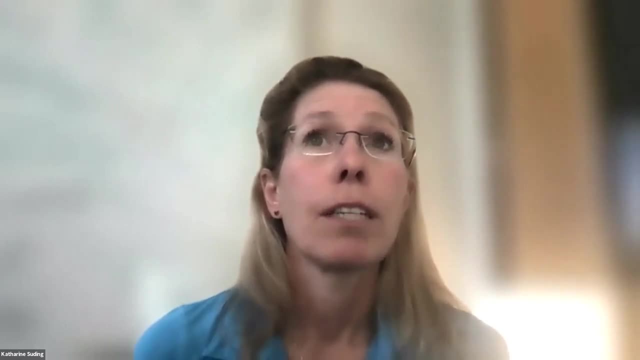 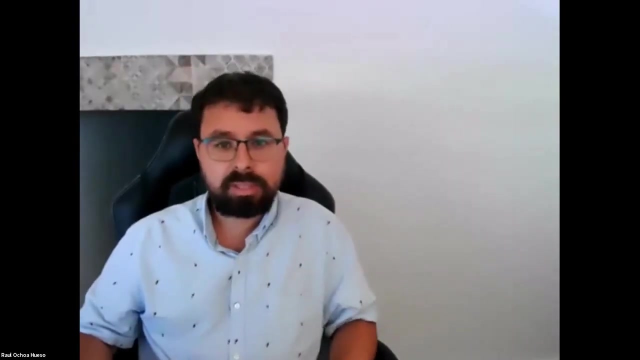 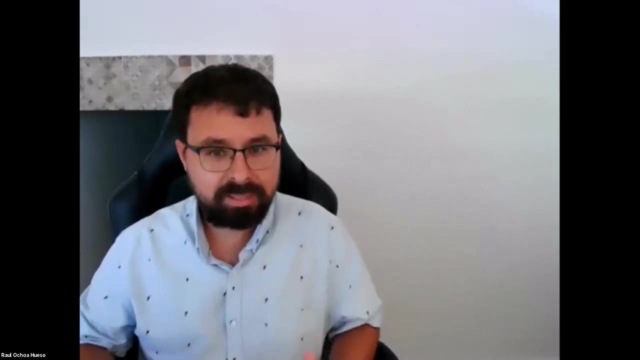 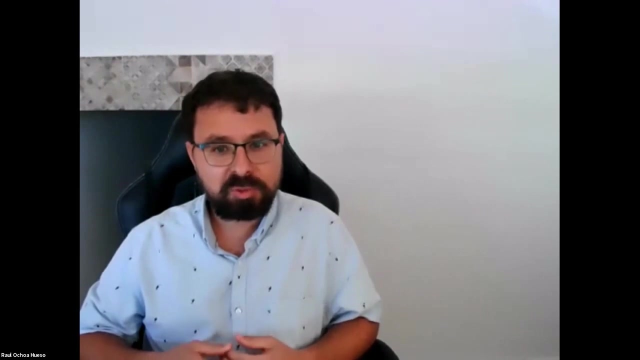 kind of what does it take to kind of recouple those components and, in your view, okay? so to me, the first thing that i would like to say is that i consider regenerating ecosystems somehow similar to playing guitar, if you allow me the comparison, because you, if you want to play a tune, normally you want to, you know, touch different strings simultaneously. 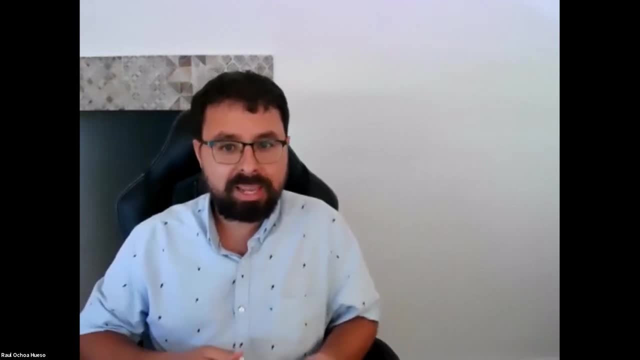 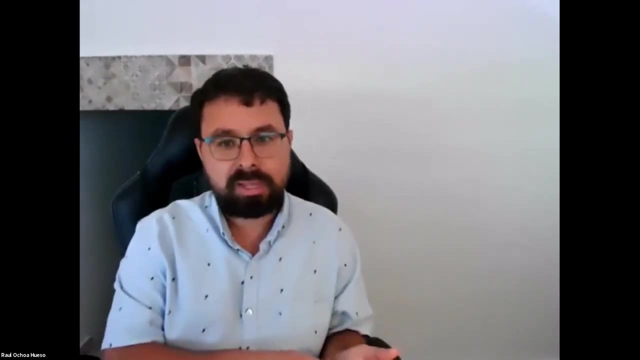 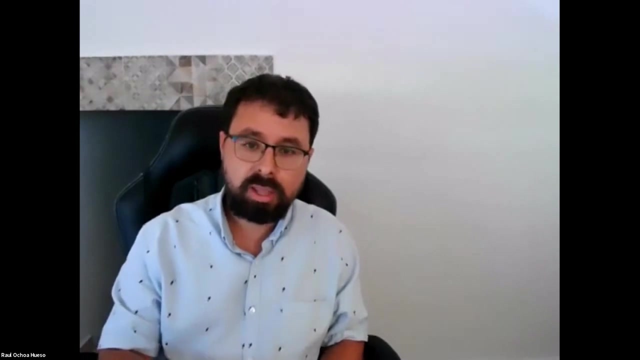 so playing a tune involves different strings. so playing a chord, and if we want to play, or let's say, to reattune back that ecosystem, we need to consider that. and so recoupling means inoculating, of course, but that would be one string. then we also need: uh, like i was saying in, 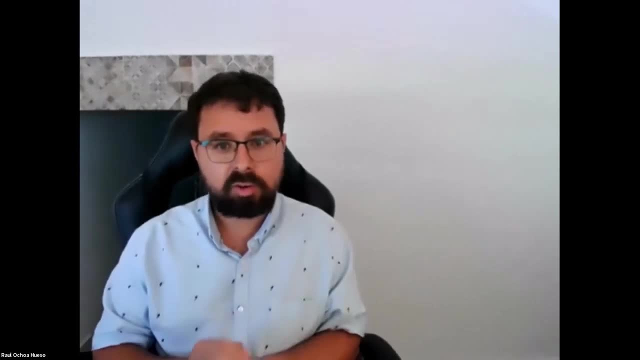 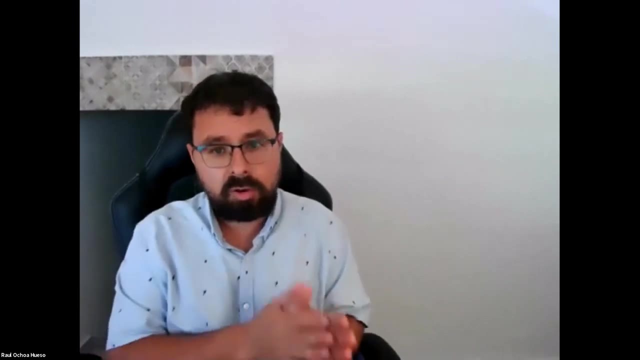 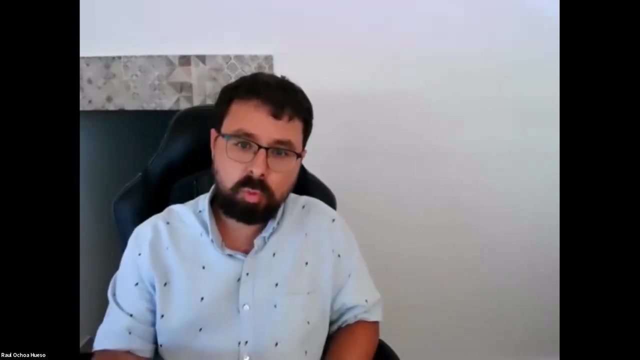 the presentation. we need to create gradients. i think that's the core of how to bring back the function into ecosystems, because uh gradients is the only thing that allows uh energy and matter to flow, and that's what we want to recover. actually, we want to recover functioning. 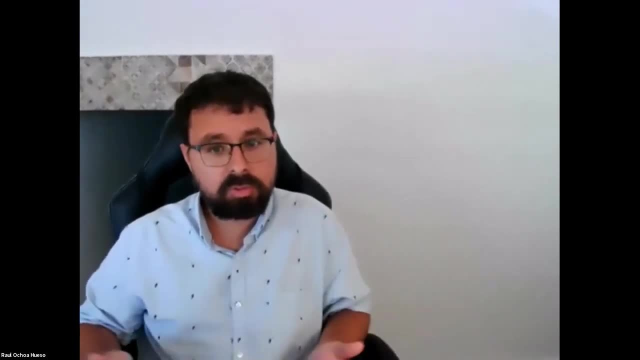 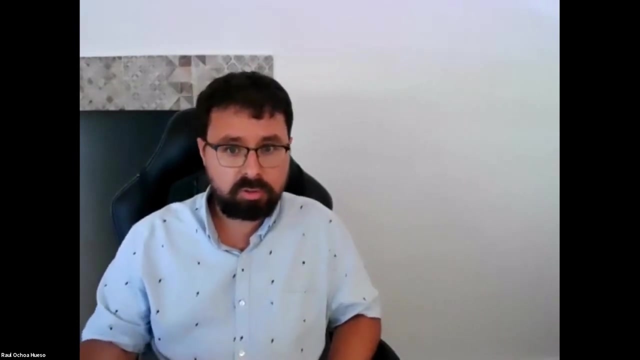 no, and that function is only allowed if we have gradients, otherwise nothing moves. and if we create gradients artificially, for example, inoculating is creating gradients. also, sowing plants is creating gradients of plant diversity. obviously that's not going to be homogeneous and maybe, along with those microbes and with those plants, perhaps you could add um small amounts of. 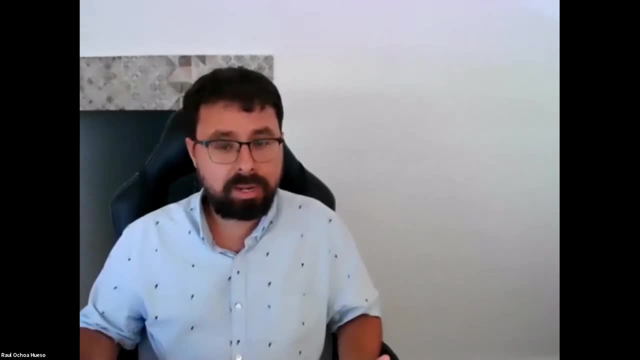 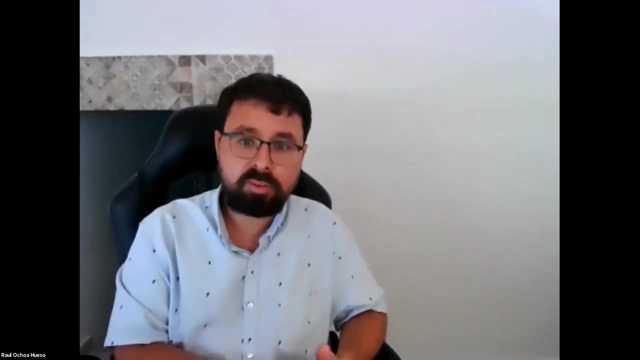 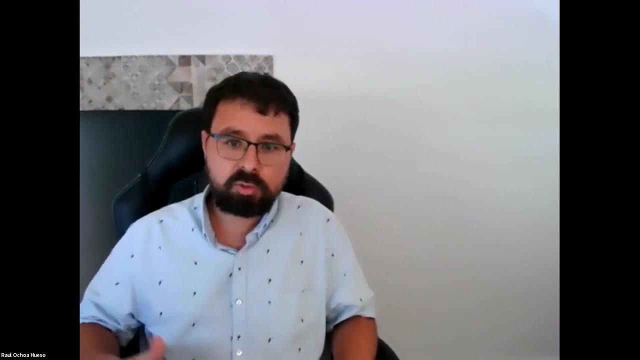 clay, for example, in the form of pellets, and then you spray it over your fields and then somehow you can bring the large animals which, in my vision, are like composters. so they're like, they're just recyclers and we need to bring that back. and once we bring that back, we start the ecosystem. let's 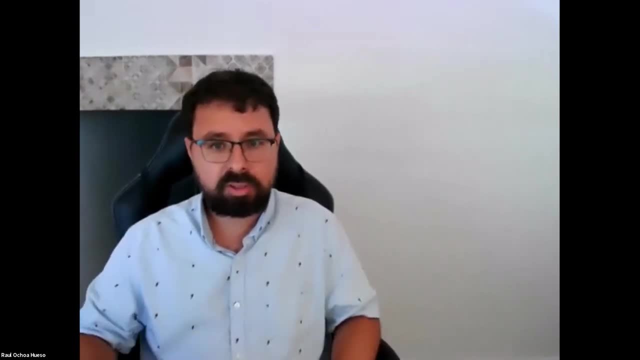 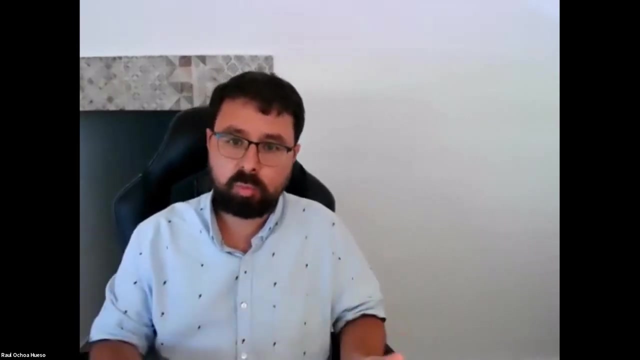 say we await the inner power of the ecosystems, although i know it sounds a bit esoteric- no, but that would be my vision. so i don't say that we need to leave nature. we need to help nature to awake by playing the strings that we want. in other words, we need to 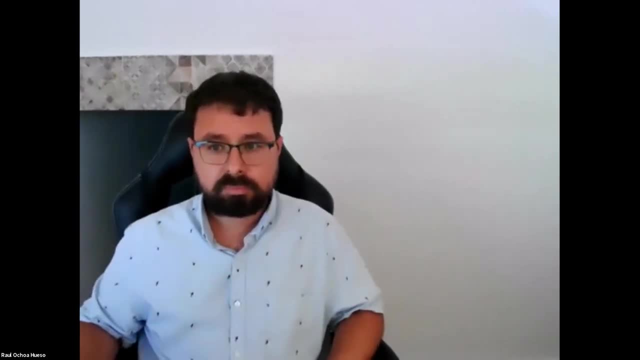 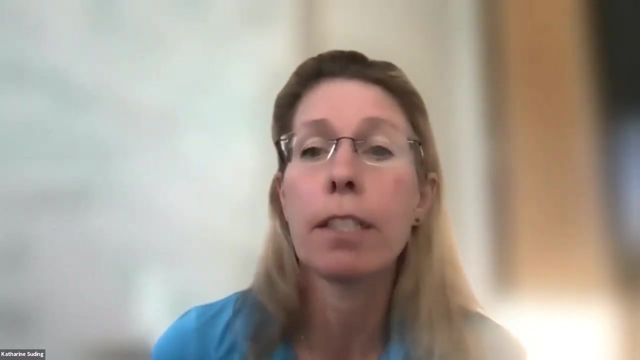 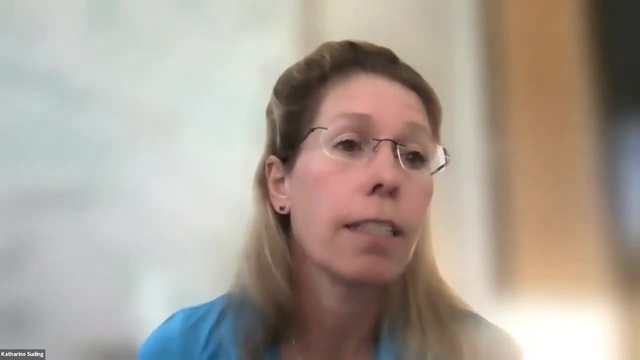 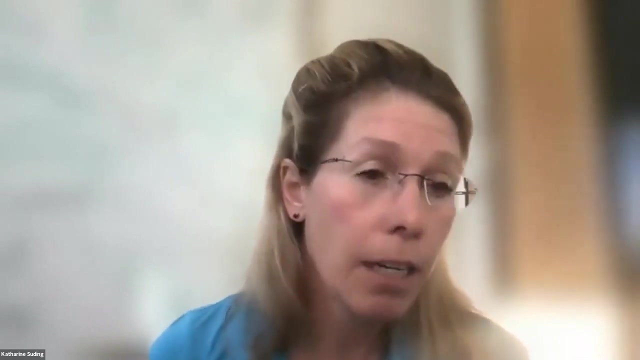 use the right chords. we need to resonate with nature. excellent, i'm glad that you, i'm glad that you, uh, you brought up also the other ways of intervention and particularly we have a couple questions about um, about grazing or large animals or even soil fauna. so i was wondering if people could speak to what role you think um those kind of other elements of. 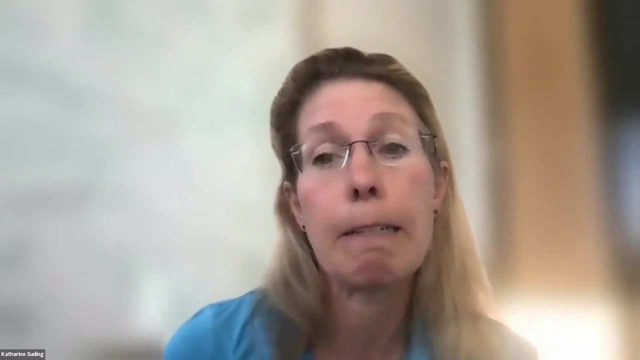 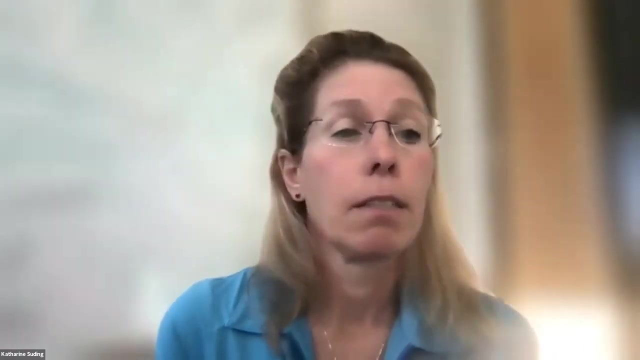 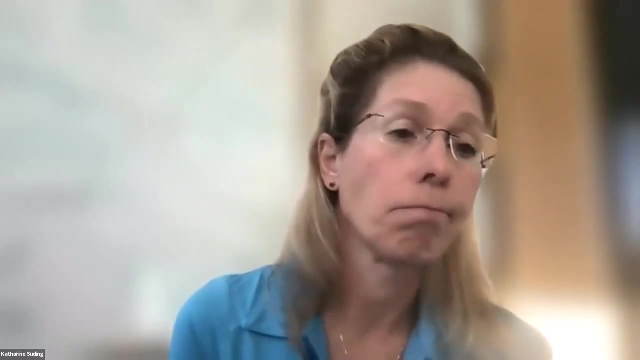 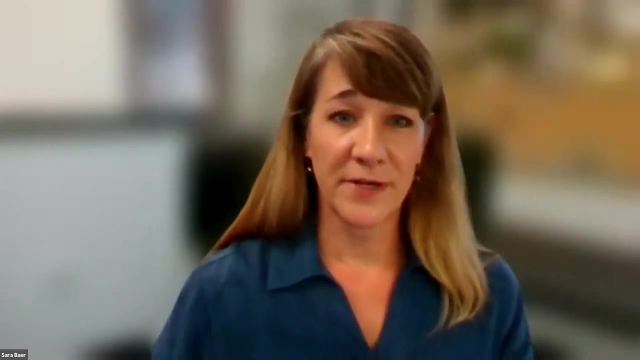 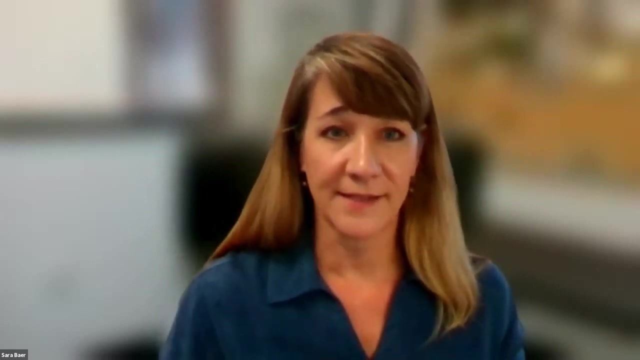 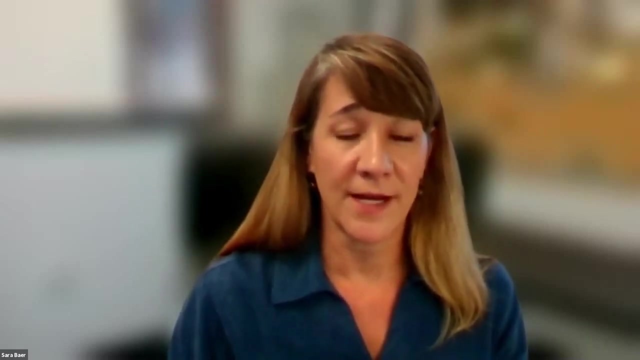 the of the ecosystem. have um on um, restoring soil, biodiversity or establishing um, those, those couplings. sarah, do you want to just talk about grazing? yeah, i think raul brings up a really good point about the potential for bringing in um, or access to, large animals. grazing animals i mean, even even proximity, i think, to other 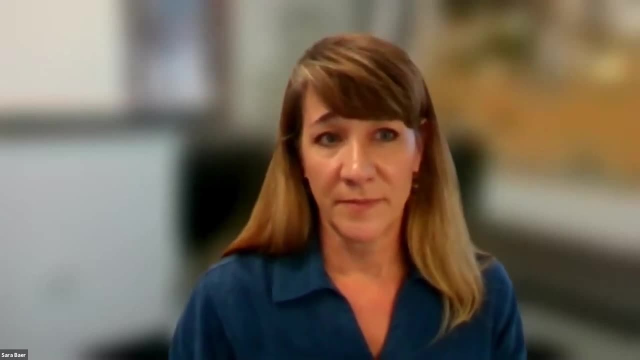 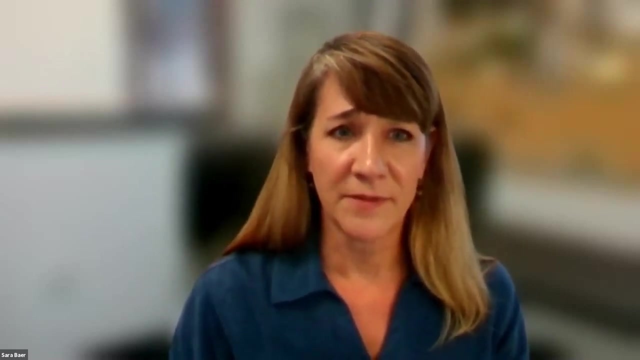 natural lands and connectivity um could be really could be important. um, i think there have been some earthworm additions to reclaimed mind lands, uh studies on that i mean, but that's uh a lot. i mean i know that they have been used as like a- you know a- bioturbation. 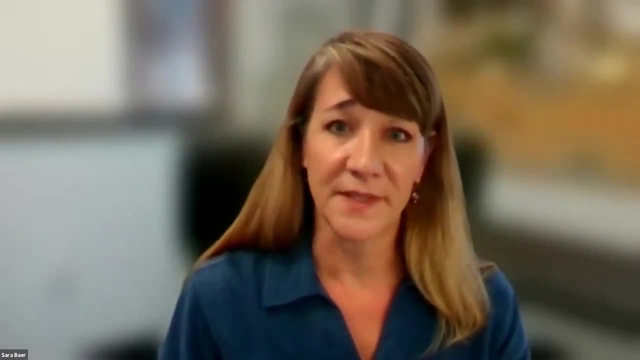 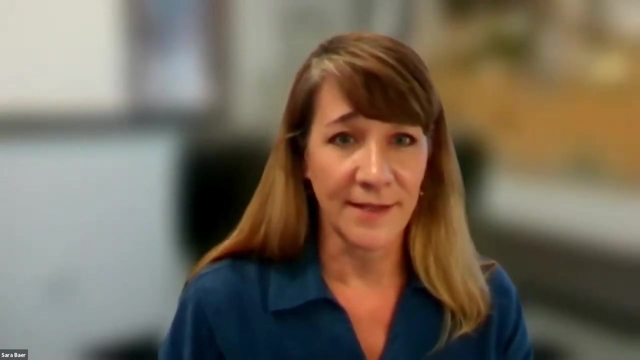 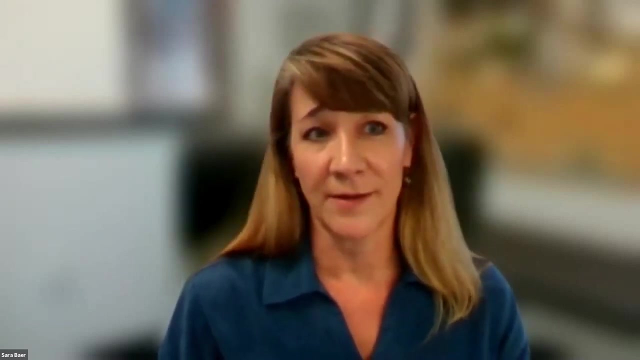 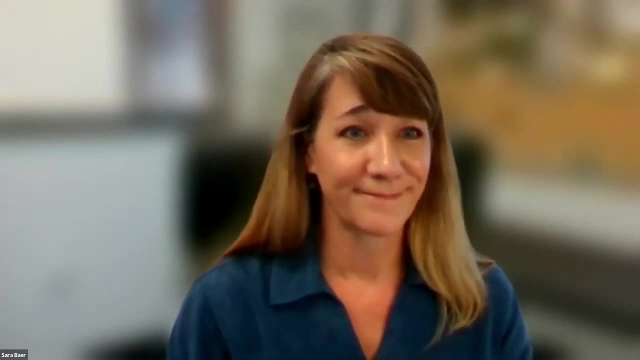 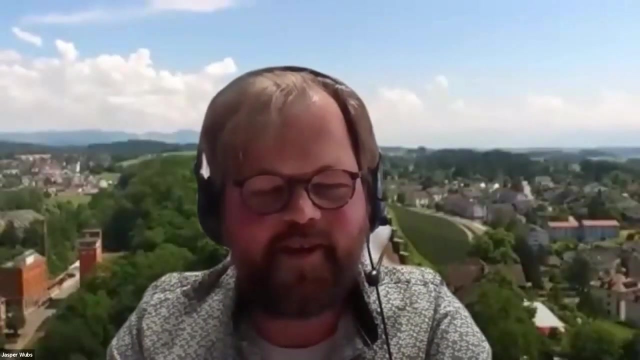 like tool to reduce um compacted soils that then enable you know seeds to germinate and facilitate the cycling of nutrients. and of course, they're microbial hotspots as well. anyone else want to jump in? i know very little about soil fauna, but i guess it could be important. i mean i i have heard stories. 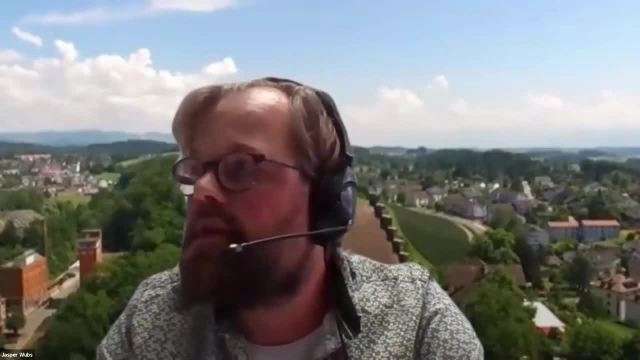 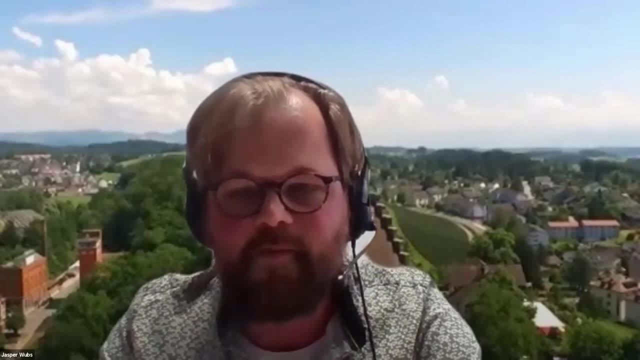 about grasslands where, um, for some reason, the, the fungal, but the dead fungal biomass was not degraded and and and i, i, i think i remember that was part of the reason why i was not able to. and i, i think i remember that was part of the reason why i was not able to. in a flood in the during the winter of the early 20th century. in a flood in the early 20th century, it was the diversity of species that remained in the system id. it was the diversity of species that remained in the system and it was partly because, indeed, the shredders in the system, so the vertebrates, that break. 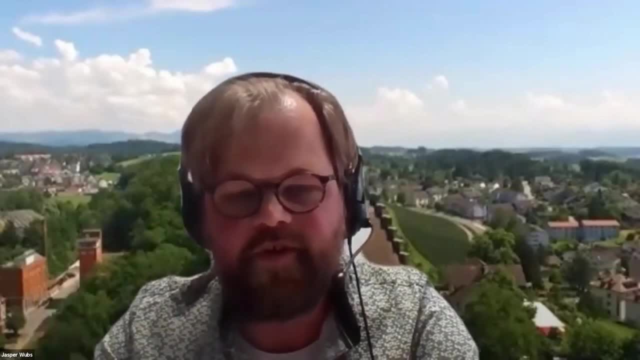 and it was partly because, indeed, the shredders in the system, so the vertebrates that break down the massive chunks, uh, they were not there, and so so the whole decomposition by fungi and bacteria was not happening, and so it may be that, in particular cases, the system gets stuck and you 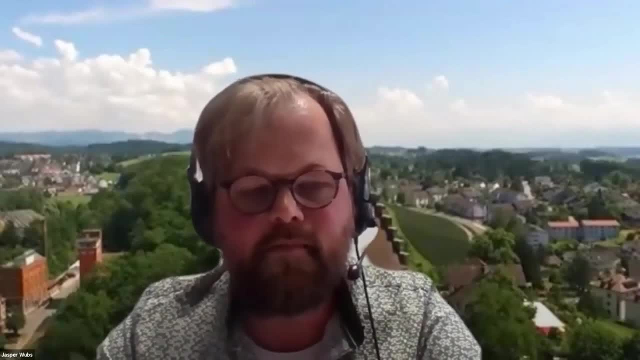 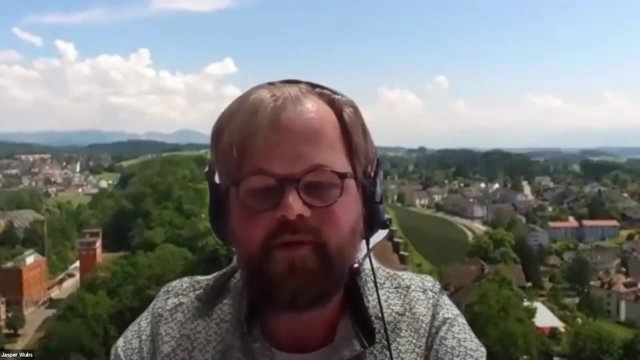 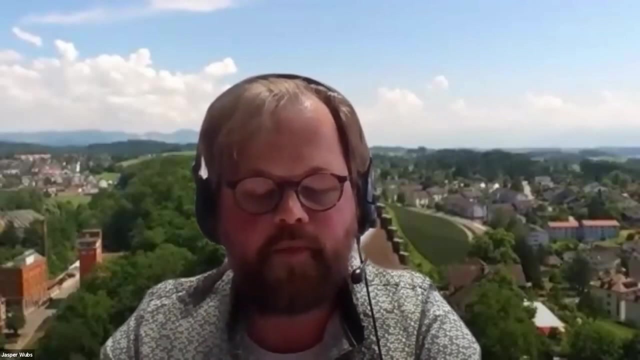 need these fauna to to unstuck it. i have the feeling that, more generally it's it's more about process rates than than things being possible or or happening versus not happening. so in many of of these fall, i think, speed things up um process rates by geochemical process rate, um, but you know. 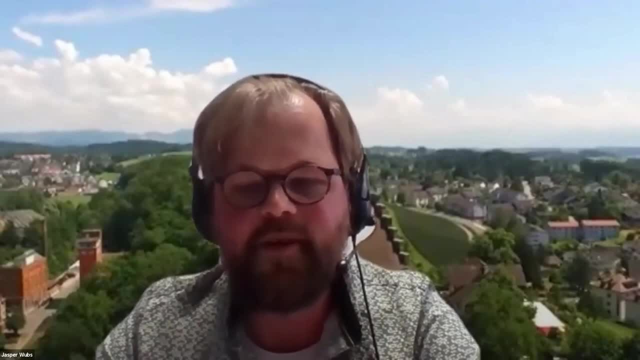 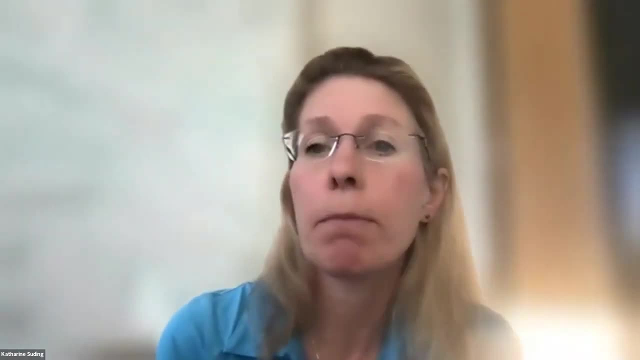 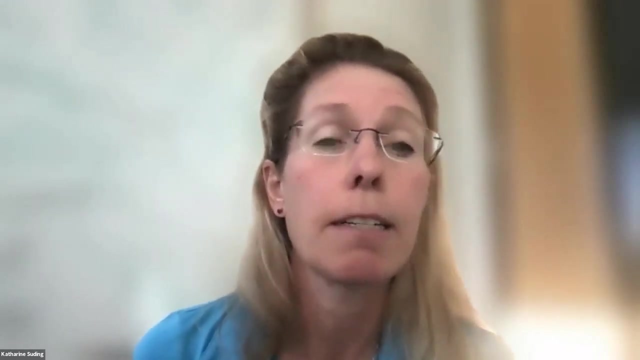 i. i guess it depends a bit on what you want from the system whether that's beneficial, yes or no. great thanks, um, i'd like to shift a little bit. we have multiple um questions about monitoring and whether um you think that, um, we should start monitoring soil diversity. 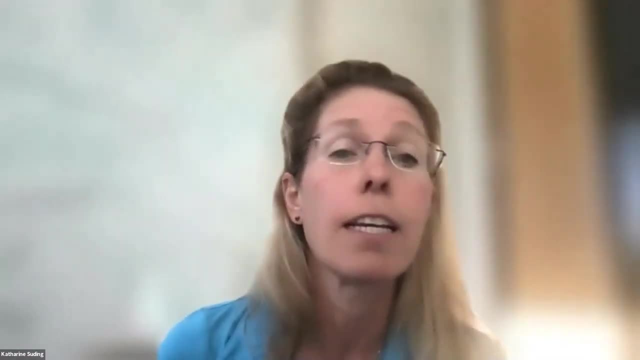 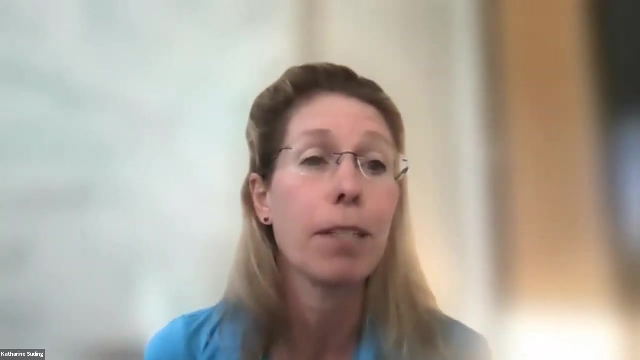 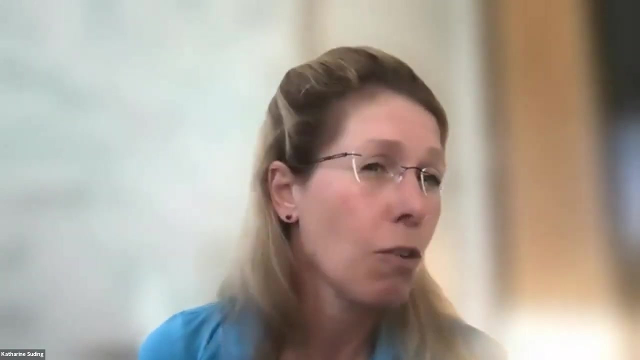 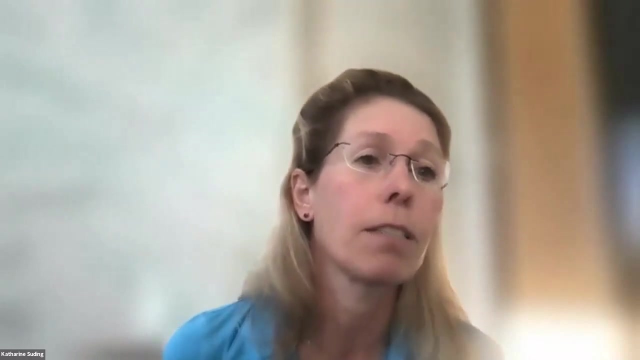 and restoration to determine success, for instance? and if so, are there kind of keystone, kind of indicator? species that are taxa, that might be ones to focus on um and um? you know whether we should start thinking about that is even an indicator of bigger data, right when, when a system is is starting to lose its integrity. 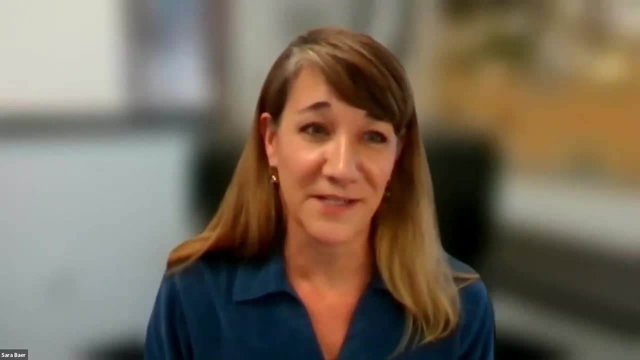 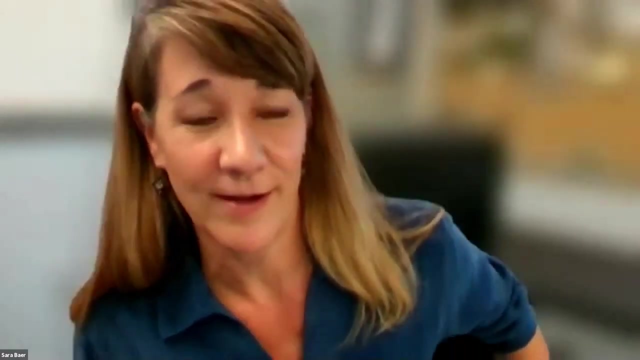 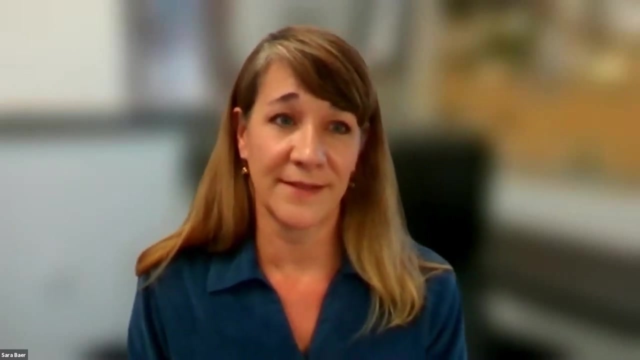 i would. i would say my first thought is: is monitoring soil microbial communities would not be easy. i mean, i guess i'm i'm not exactly sure that you know the context of of the question- like if it's something, uh, um, an agency could go perform easily. 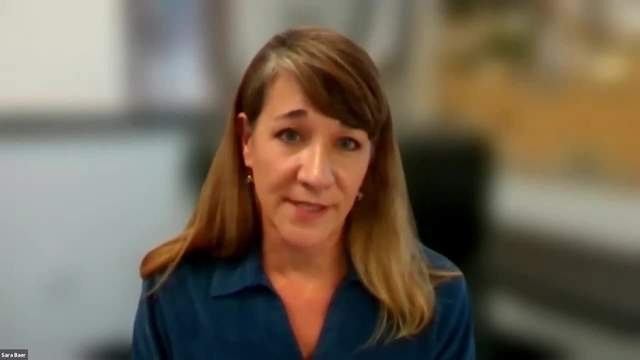 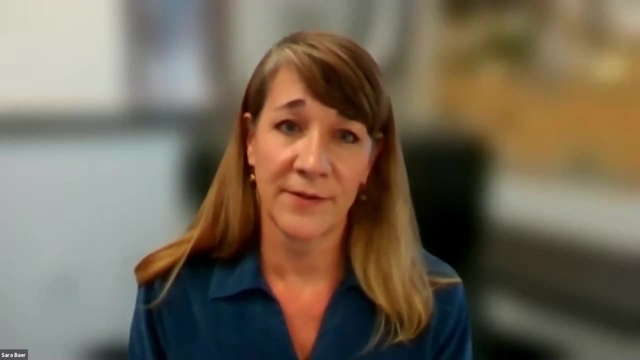 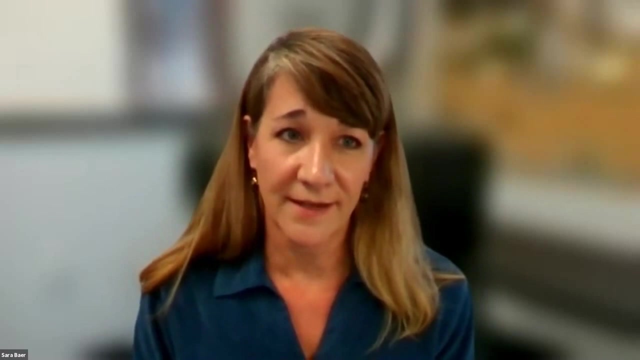 um, i mean there are, there are our core syndicators. i mean looking at that, at that fungal biomass, um could be really important. i mean the fungi are critical and forming uh aggregates and they're hyphy in the soil for transferring nutrients to plants. i mean there are an aggregate stability i i think there are a variety of other metrics that. 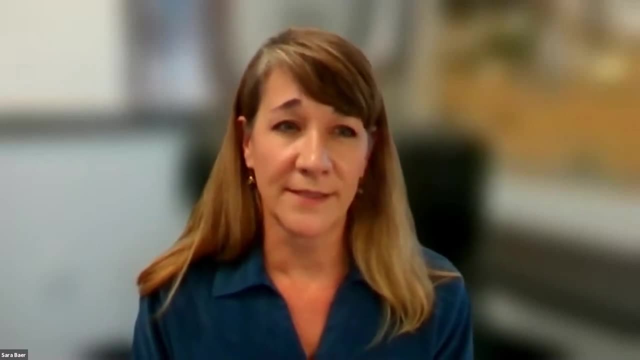 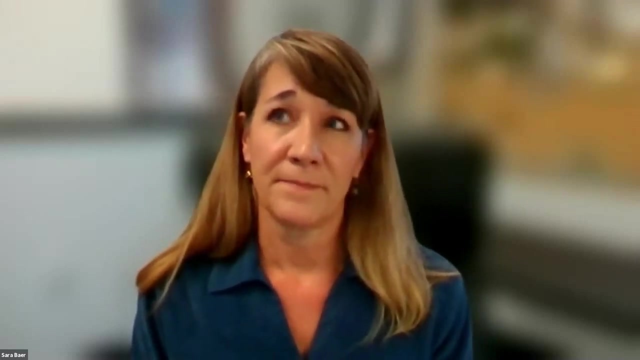 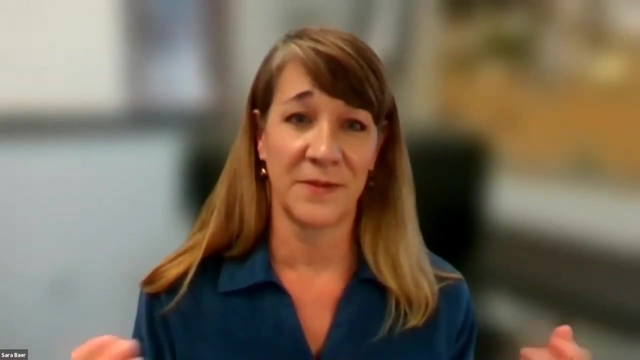 will be helpful to predict how this is going to happen. so, for example, that might be a little easier to look at. that could be indicative. So I guess what we really need might be an index, you know, an easily measurable index of the soil microbial community. 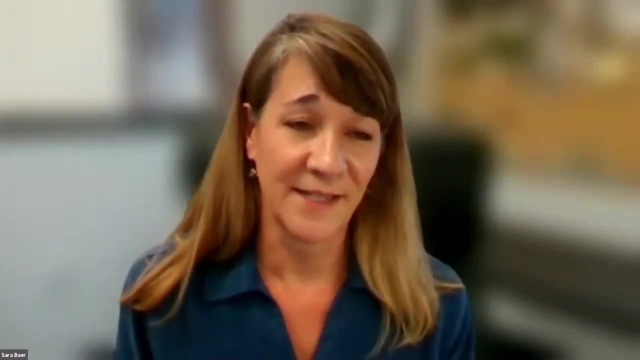 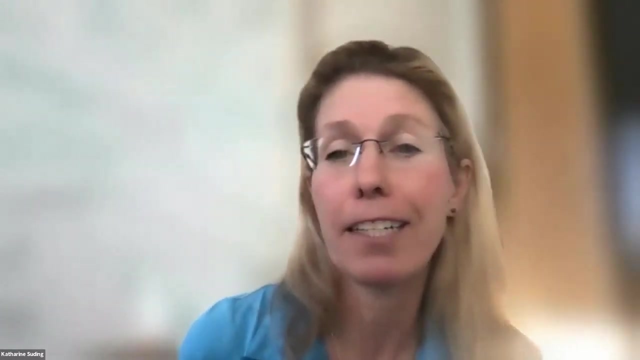 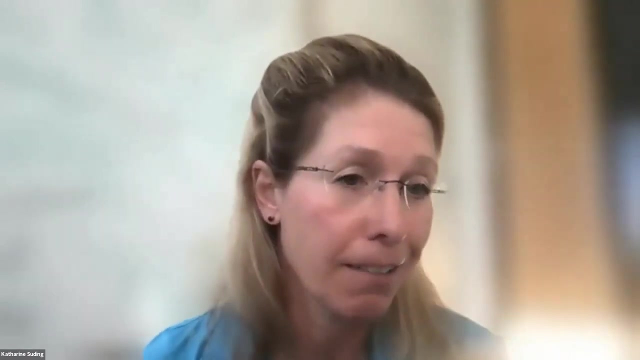 and then that related to plants and diversity. Right, I think that we shouldn't. you know, molecular methods are great and good for for some questions, but certainly not for getting these practices to scale up on the ground to impact large portions of the globe. 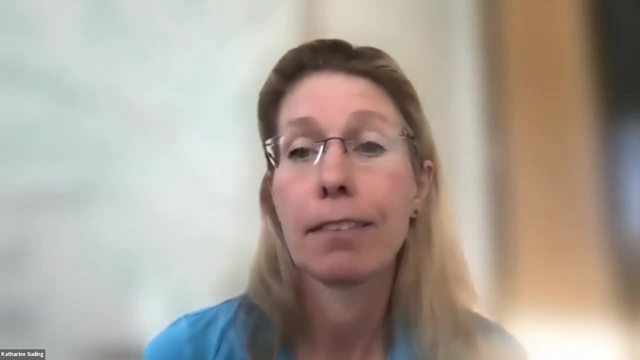 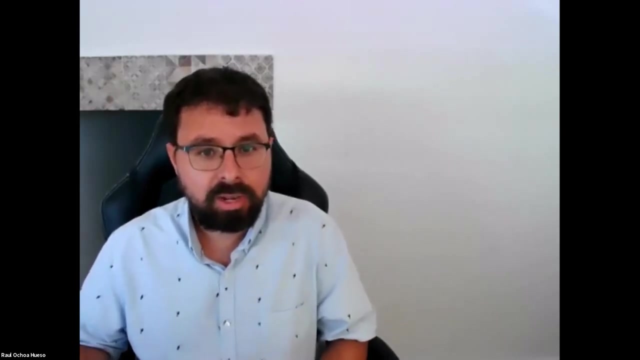 Anyone else? Yeah, Raul, I mean I would say the very classic method to monitor the health of soils is to use a soil enzymes. Right, I mean, that wouldn't be soil biodiversity, but they are very, very important And I think that's a very, very important thing to do. 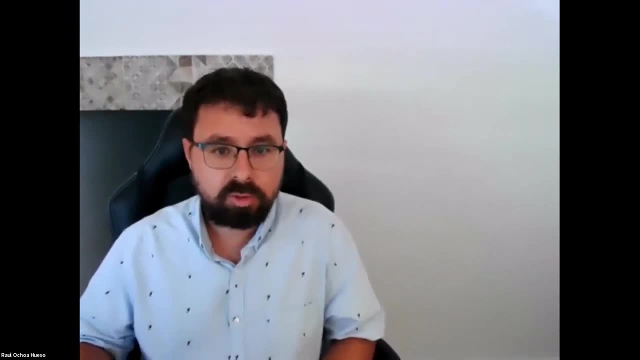 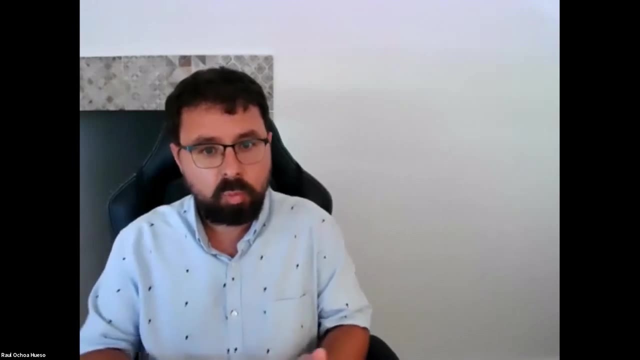 How, let's say, my daily- produced by soil biota. So perhaps if we want to money to monitor how soil biodiversity is doing, we may do it better by looking at how they are functioning. So in other words, we just may be able to measure enzymes, perhaps a variety of enzymes, and then 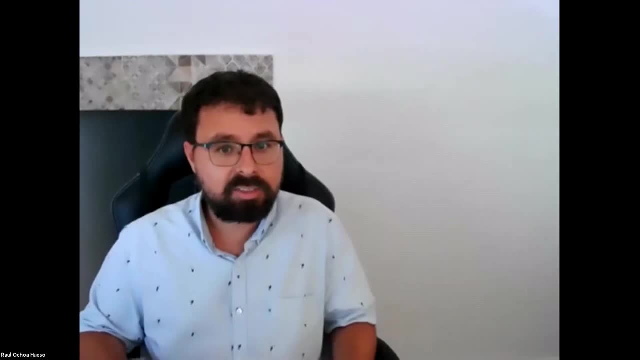 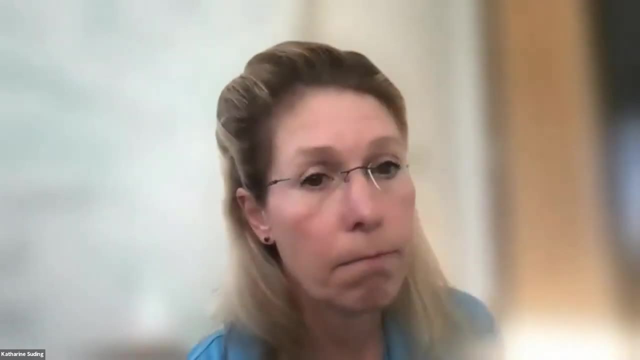 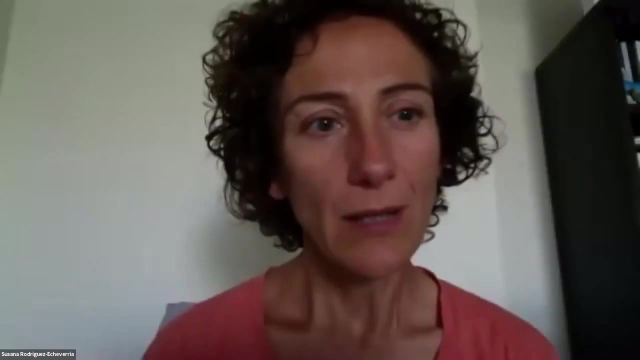 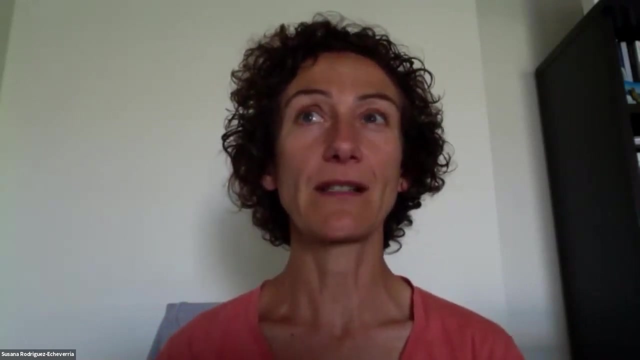 derive an index, It could be a cheap alternative. Susanna, do you have any thoughts about root endophytes, or you know that aspect of the system? Yeah, well, it's like you were saying before: monitoring soil microbial diversity is. 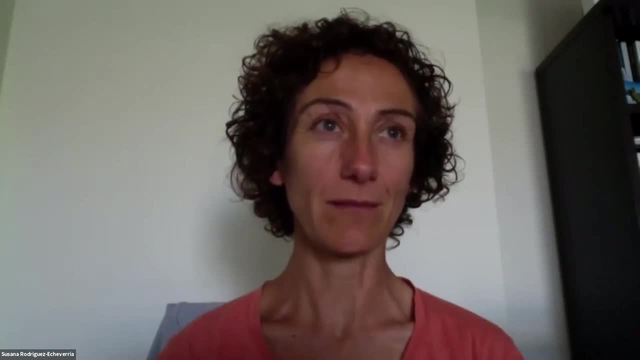 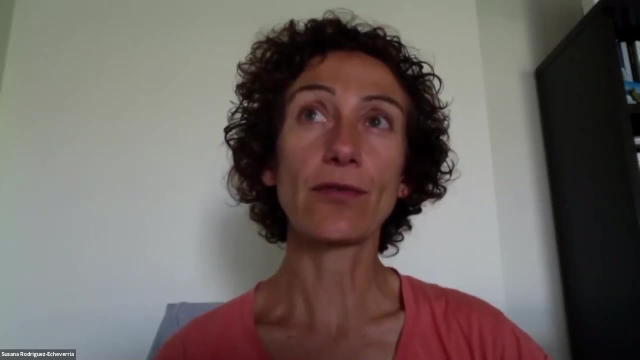 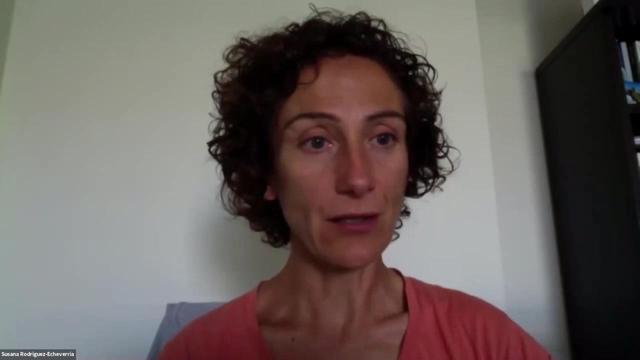 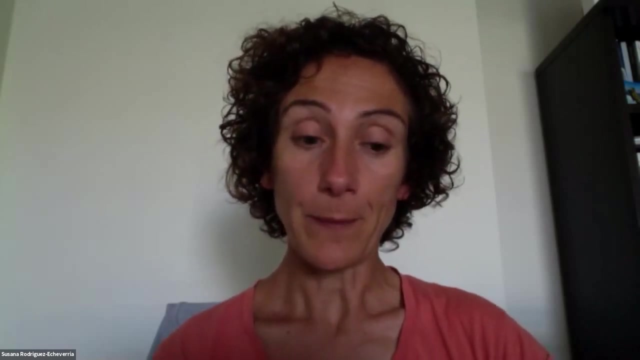 expensive and not easy for managers and even for many scientists. I think that it would be better to focus on function, like they were saying in soil, functioning not only enzymes but other indicators of decomposition or nutrient flows. And then for the root endophytes, there are cheap ways to 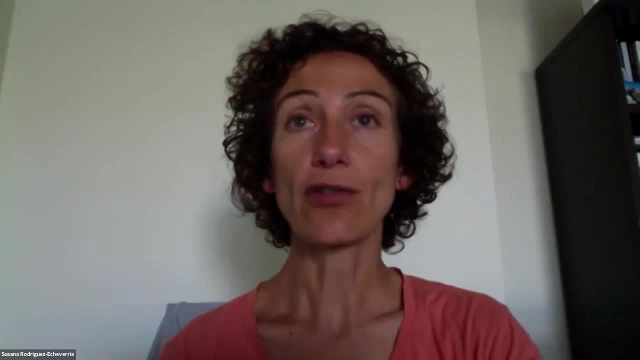 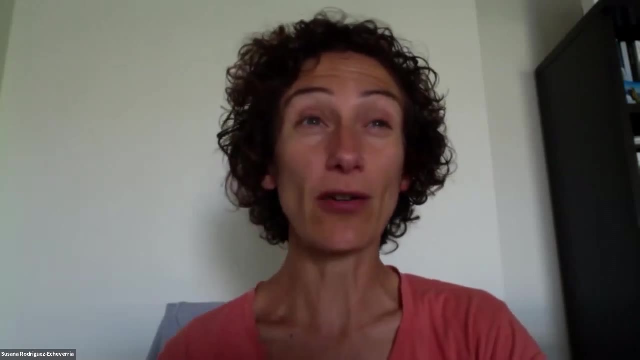 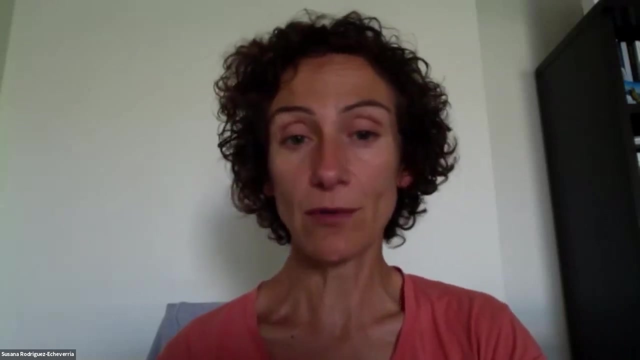 analyze them, like from using microscopes for or just for symbiotic bacteria, just to count the nodules. But they are all destructive measurements. So it can be something that can be done at certain points of time to check how it is going, But I wouldn't think that it's going to be the best way. 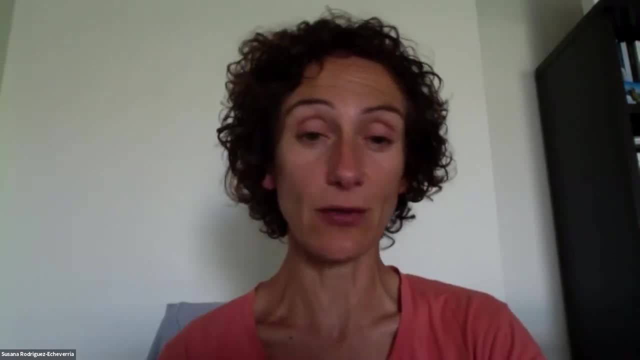 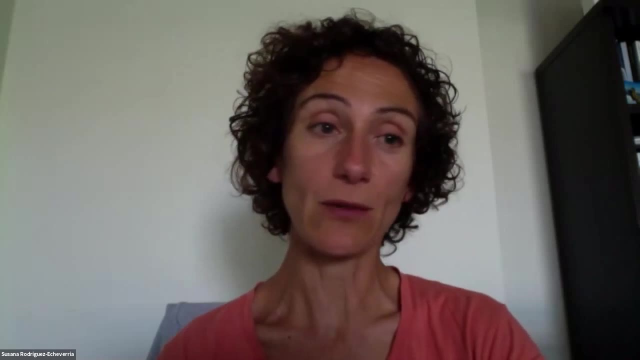 to do it. I think it's better to analyze how the plants are doing. You can detect any nutrient deficiency or any growth impairment or something like that. I think that plant monitoring is easier and will let you know what is happening. Yeah, I agree with that. I think it's better to do the root endophytes and then mutual enzymes. And also that brings me back to one of the questions before about how inoculants would establish and disperse. I think usually you do want to do the inoculation at the beginning, So you have the plants to establish And then that usually has a very good fast result on the plants. But yeah, It is true that there are not many monitoring schemes after that, after many months or years have passed to see what happens. So maybe the inoculants are only there for the first initial stages and help plants, And then the system takes over and they disappear, And then we have to. 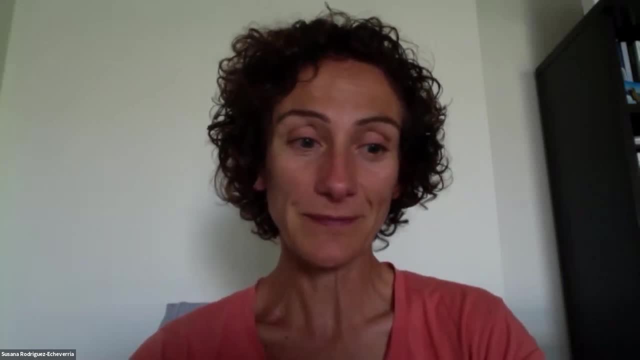 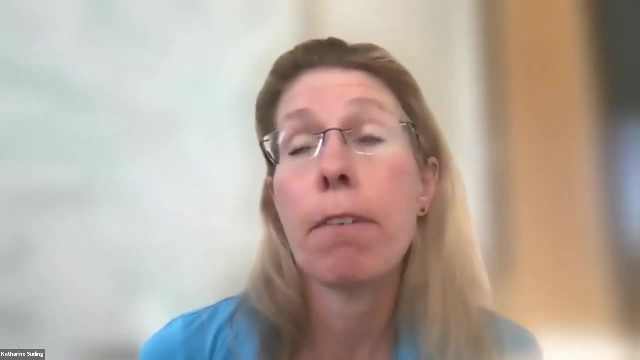 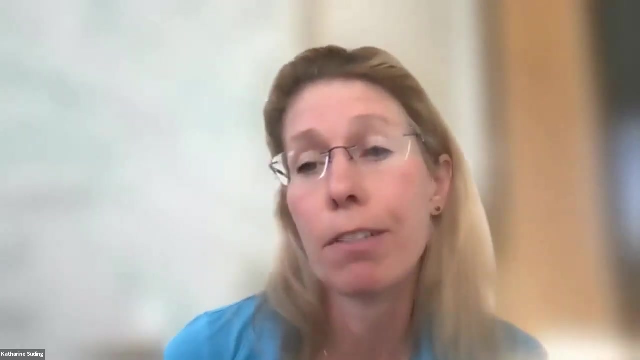 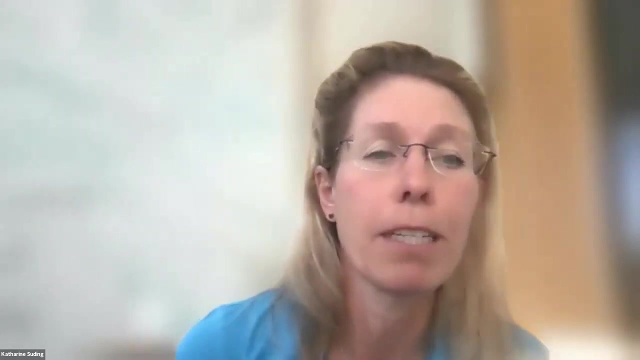 measure something different, something more functional. I think a lot also about if you're in a degraded system. there are plant-microbe relationships that exist right, And so you have to Almost knock out some less beneficial relationships to establish the more beneficial, And that's pretty difficult. 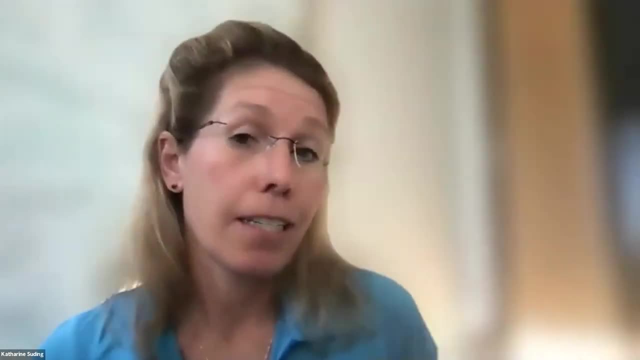 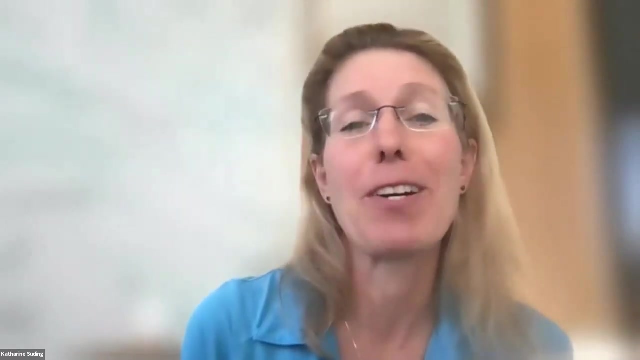 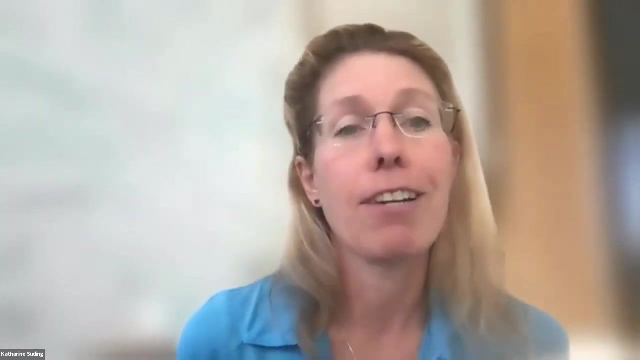 to do, And it's not quite clear who has control, right, whether it's the microbes or the plants. I mean, we'll that. Hmm, it's probably not one or the other, right? so it's a, it's a very much uh, um, just a tight interaction. 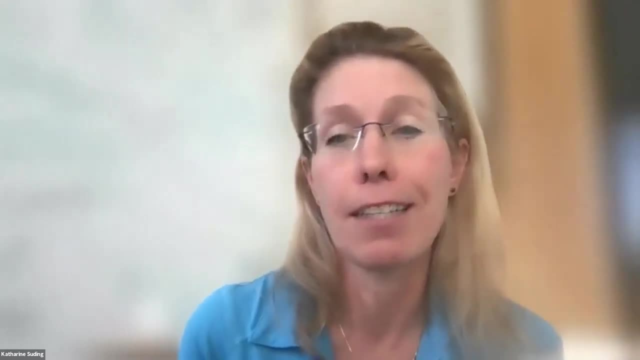 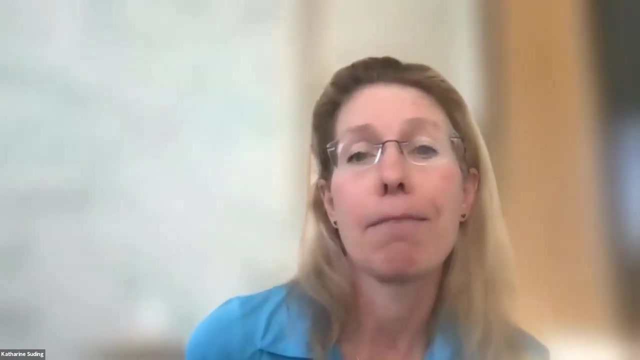 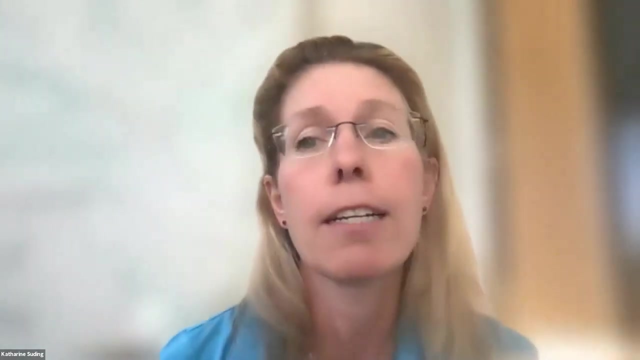 there to even to even so, just introducing the important players might not mean re-establishing the important players, and so that's, i think that's um also kind of a key question. um, there is there's there's questions about whether, um what, what do you think about biochar? 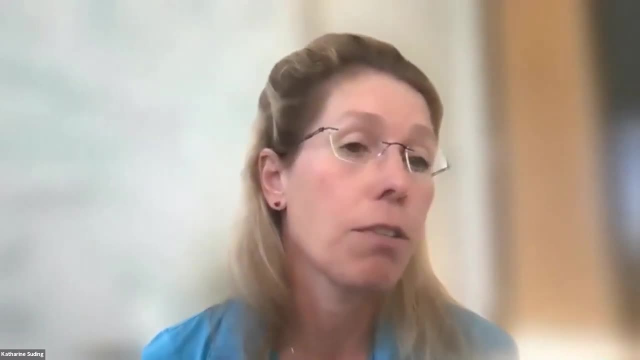 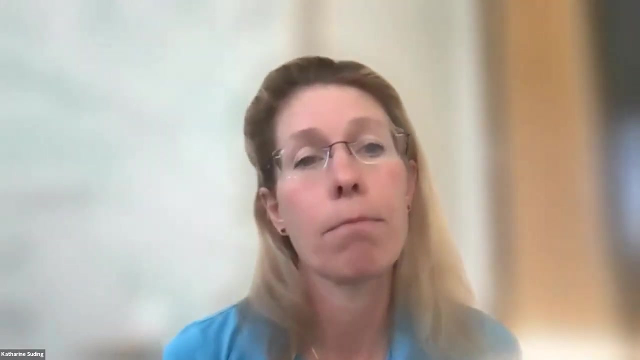 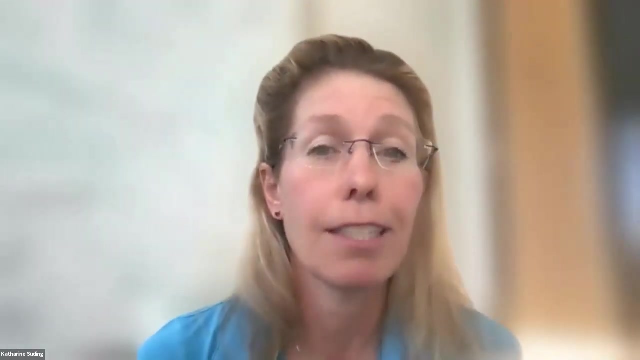 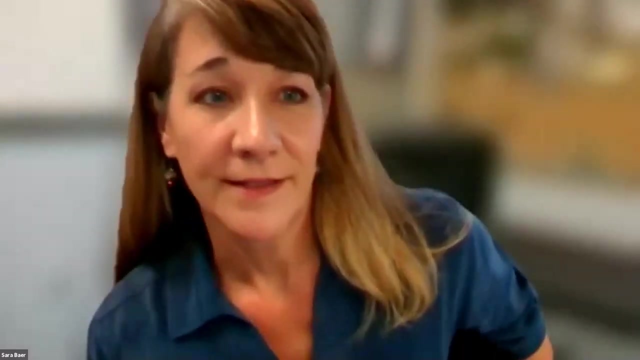 compost amendments and then also compost extracts um to introduce, um or to try to try to address um some like um soil, um soil processes, um. anyone has any thoughts about any of those three techniques? well, i think there's some. there's evidence that the adding the biochar, that black carbon, 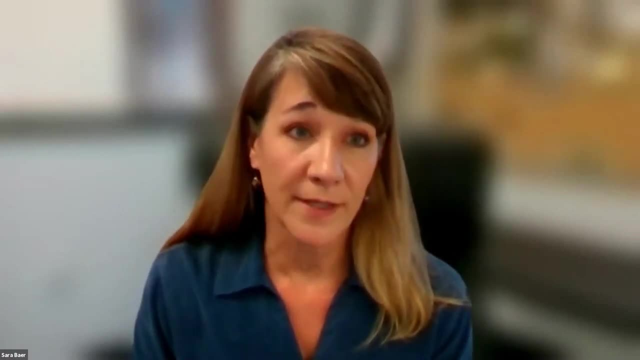 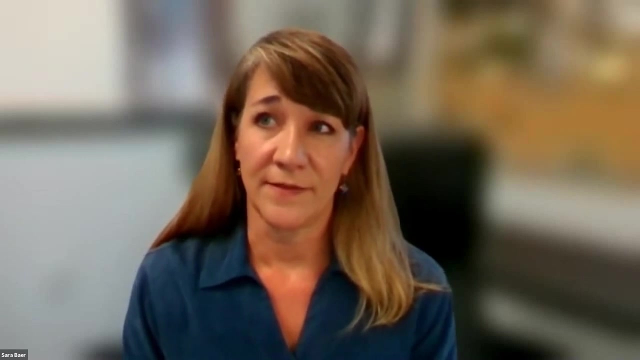 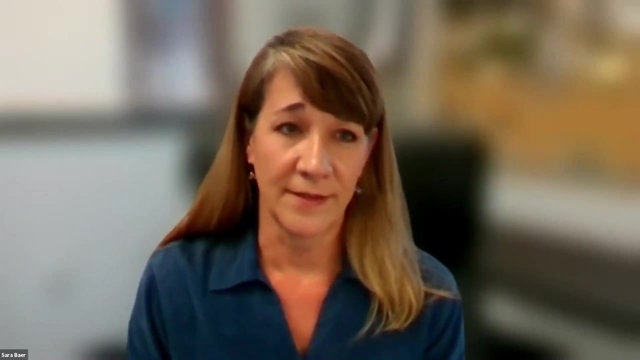 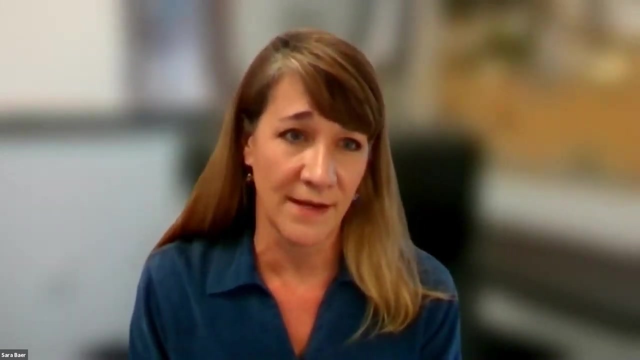 um can. it can help with carbon accrual in that um. it it's a very difficult to to decompose, but then organic matter can interact, you know, with the, with the, with that substrate and sort of um be adsorbed to it. it's a, it's another, it's like a. 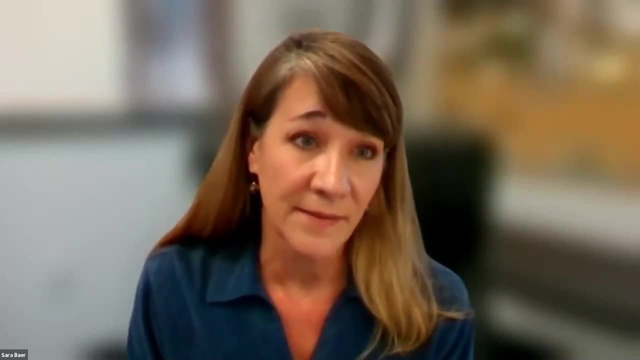 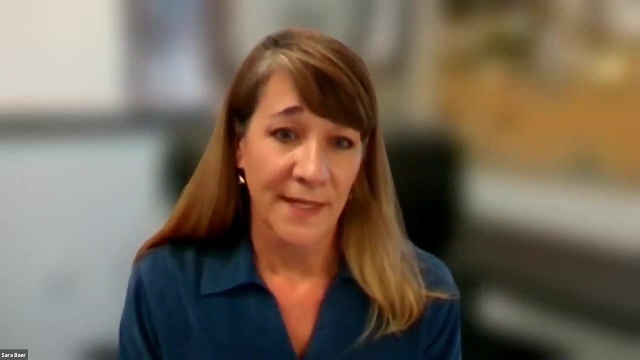 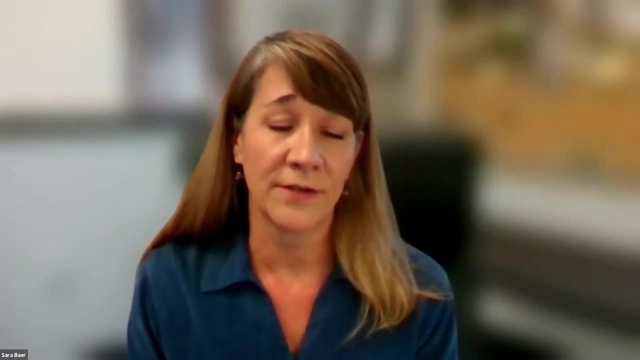 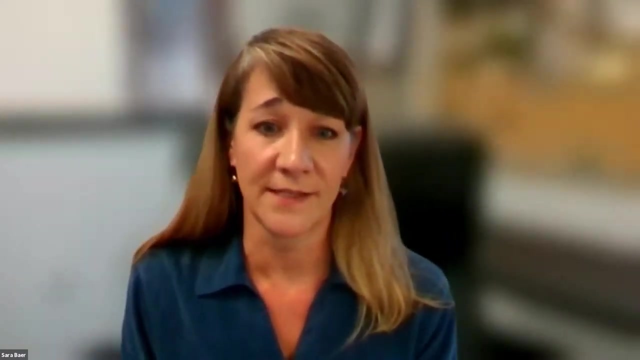 physical, chemical uh mechanism of carbon and it's a it's a very difficult to to decompose, but then organic matter can interact with carbon sequestration so that so that's an option and as far as i mean adding amendments, uh, we've added carbon and sugar to some agricultural soils at an onset of a restoration and a larger heterogeneity. experiment and we found that that can rapidly reduce nitrogen availability. so if high nutrients are are problematic, then we can add carbon sequestration to some agricultural soils. and we can add carbon sequestration to some agricultural soils. those organic matter amendments, uh, can be added and they basically feed the microbes. the microbial biomass grows, and that microbial biomass immobilizes uh, the nitrogen, so it can be a means to help mitigate, um, maybe, some excess uh nitrogen in a system. if you want to restore, you know, plants that do better in low nitrogen environments or reduce weeds, yes, absolutely. Jero. So I would say that you coulduse compost in two different ways, or perhaps complementary ways. one would be to increase the carbon and the nutrients in the soil, or perhaps also to, let's say, to improve the soil structure. but another way, we could just add some less plantation. here as to where do we need toâce compost? or we could use organic small grains, uh, let's say perオol sheet. it's been very successful in hatte, prospects, everything. just your fact that we, we will decide, jor Gaerei, I think is selected a little- what we could do with Coca Cola. we had a point 지난. 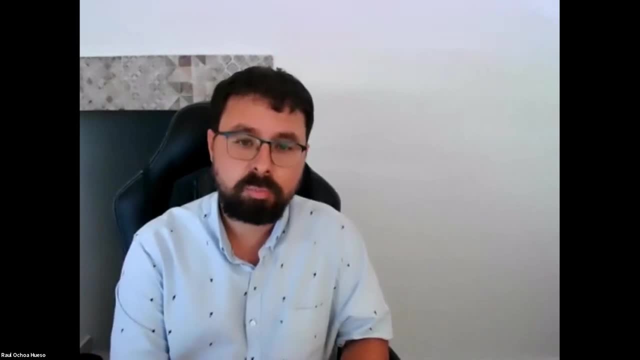 some time, including a very interesting problem and in addition to his current, but it was just functionally- to use compost would be just as a vehicle for microbes. so those are two different. perhaps, like i was saying, uh, alternatives, uh. so maybe i mean it's like when you take probiotics: sometimes you 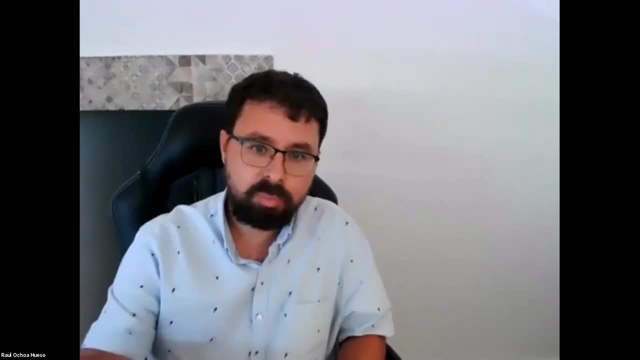 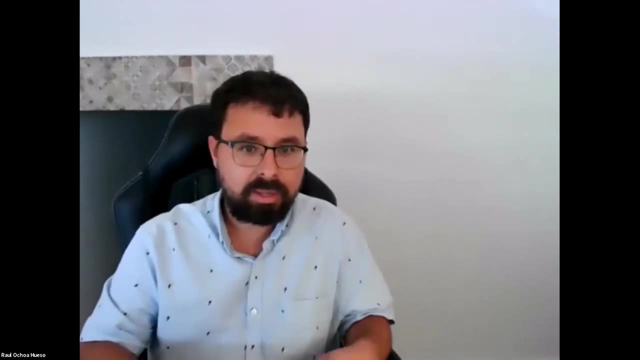 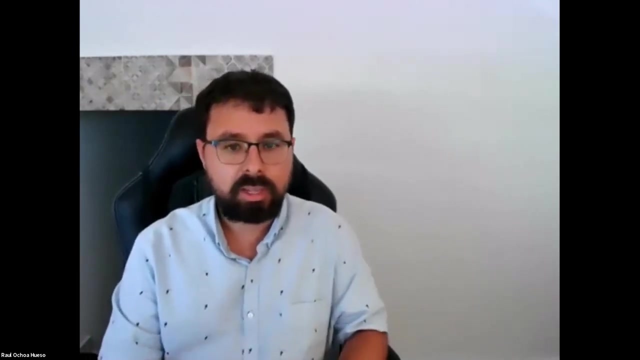 take them with the prebiotics right that help those microbes that you are ingesting to establish somehow, but you are not being fed by the carbon sources that you are eating. and in this case it would be the same. perhaps we don't want to directly enrich the soil with carbon, we just want. 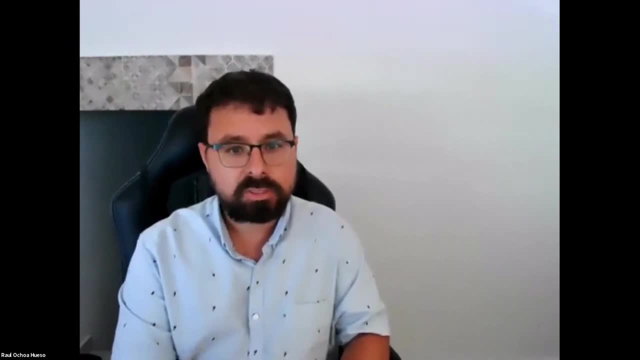 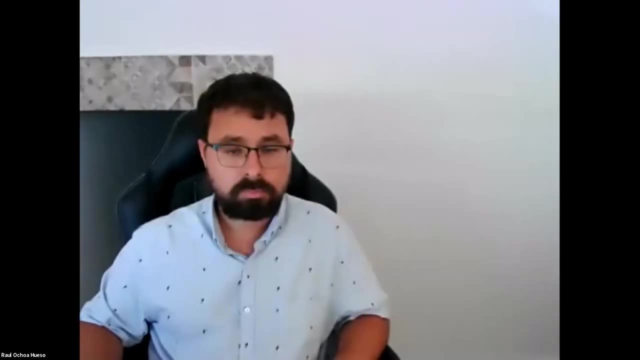 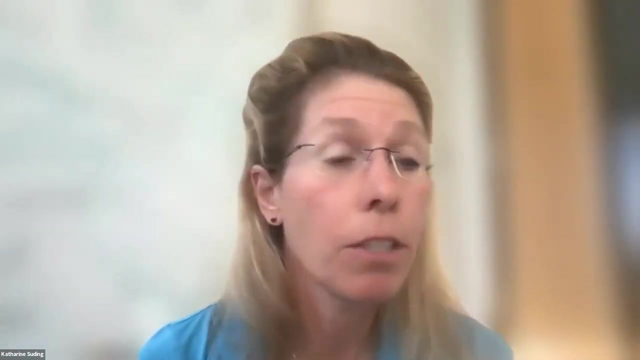 to give those microbes an opportunity to establish and get them going. excellent, yes, i, we, i have experience, we, we do um. compost amendment experiments, um and um. it looks like there is some very different effects by adding the compost extract versus the carbon and the vegetable. and um and so um. i believe that the combination of from kind of um, i believe that the combination of from kind of the same um, i believe that the combination of amendments And also the compost amendments have some kind of whole system effects on soil moisture and also delivering a different form of N than maybe what weedy plants might take up. And so it. might actually be a form of nitrogen that kind of is retained in the system a little bit more than just a nitrogen fertilization. that oftentimes might not be the best thing to do in systems, but you do need something to jumpstart plant recovery. So there is a lot of subtleties between. 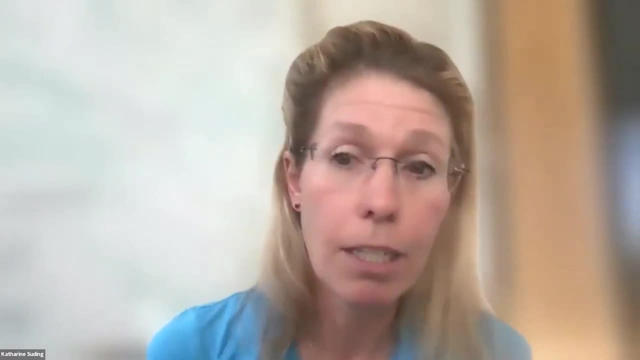 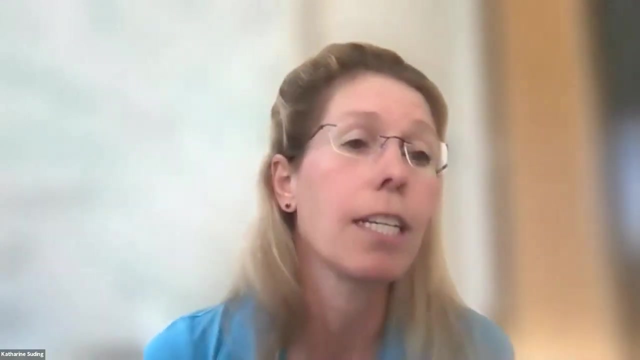 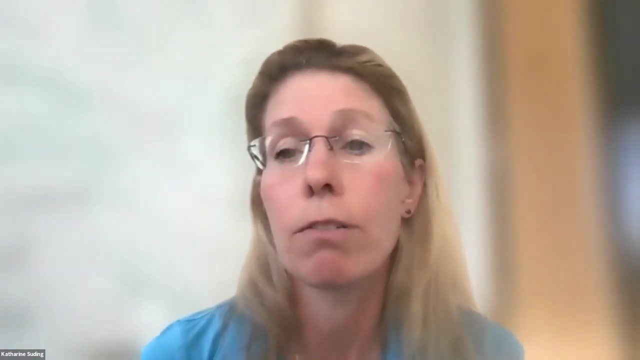 what compost does, but certainly something to look into, I think, especially when people are with a system that has have grazers right in the system and trying to make those kind of more, more complex loops or reestablish those. So Jim has a question that 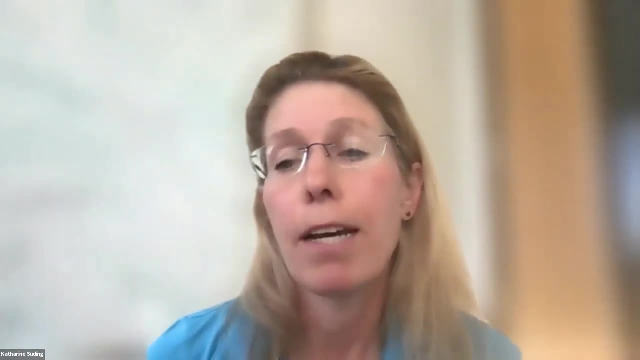 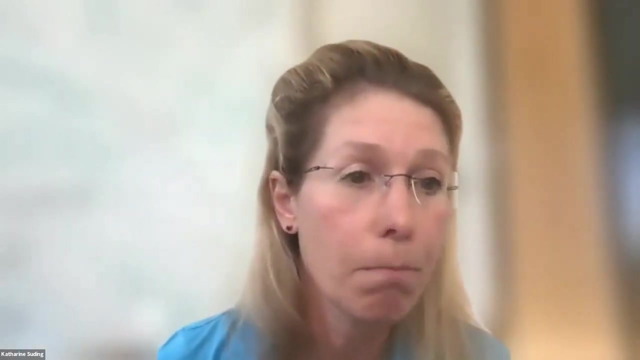 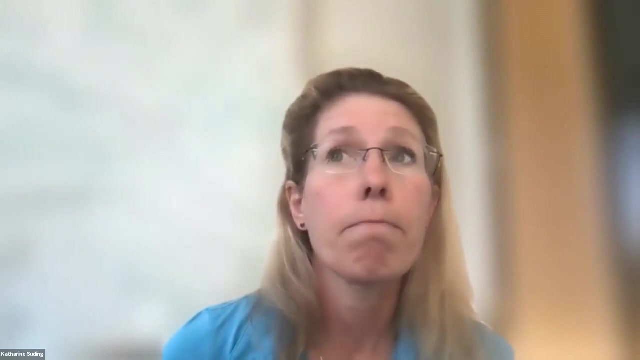 I think is kind of the elephant in the room about. so if we're emphasizing that these, these, this, the soil system is so complex, so diverse and so important because of its complexity, is there any any way that we can start thinking about actually complexity as the goal in 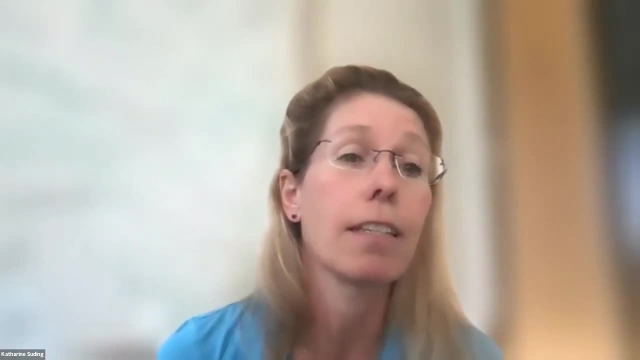 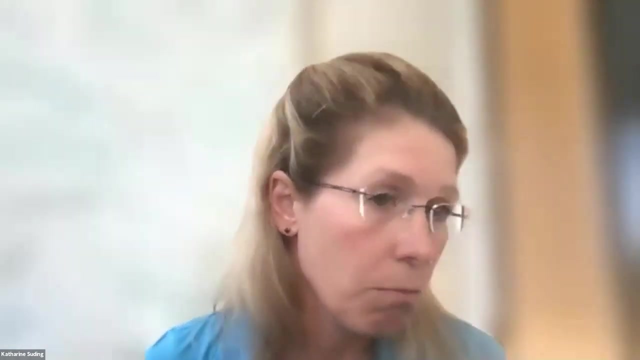 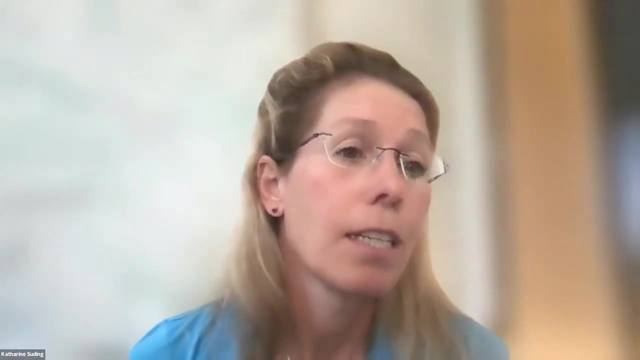 restoration and trying to think about that as the emergent property that we want to want to achieve in terms of, as Raul said, like a self-sustaining right system. So any thoughts about that, whether, instead of focusing on perhaps a one process, 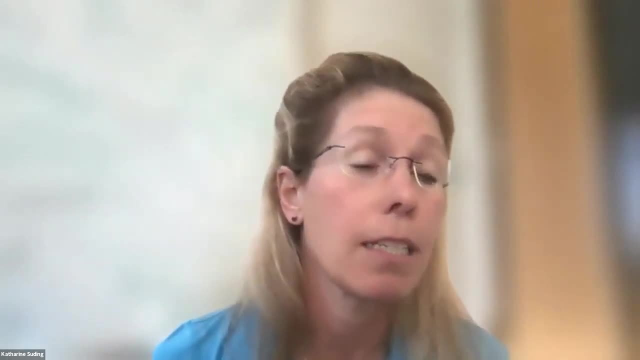 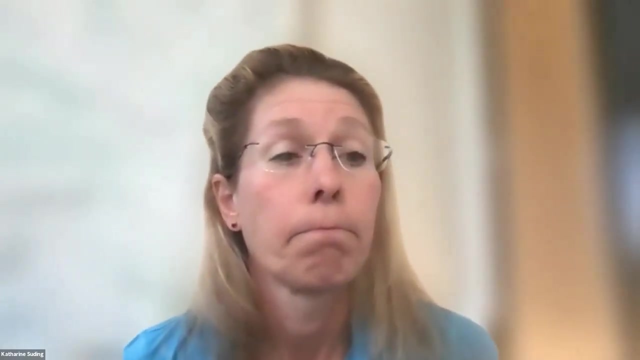 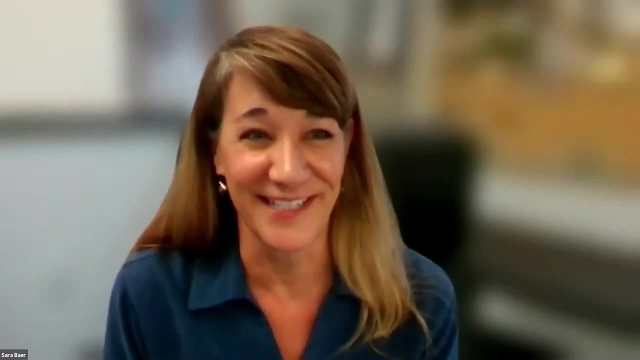 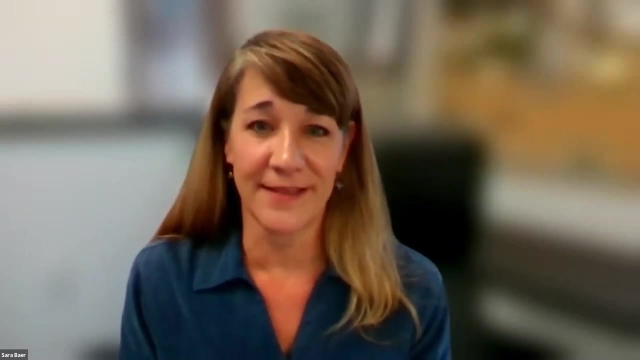 kind of turning towards complexity in terms of policy or monitoring or just our practice. Well, I've spent more than 20 years studying soil heterogeneity and restoration- its role in restoration, So I I think in in theory, complexity is something that should be promoted, because 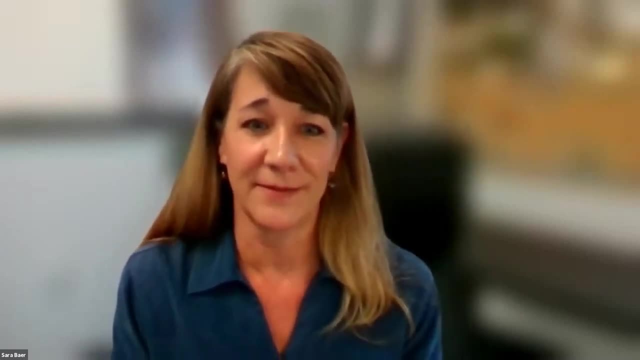 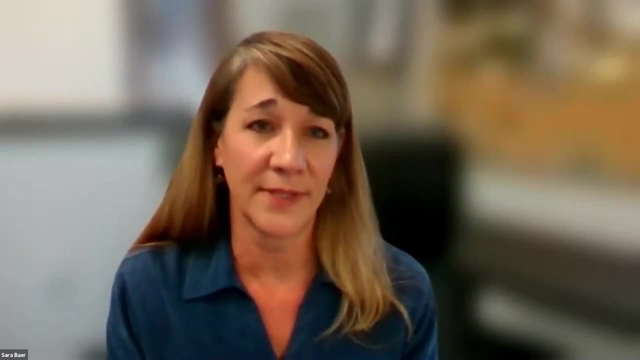 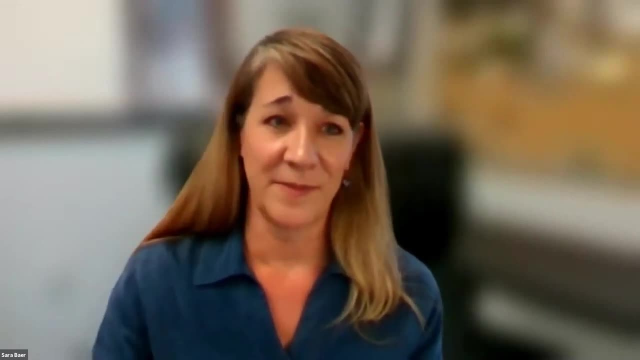 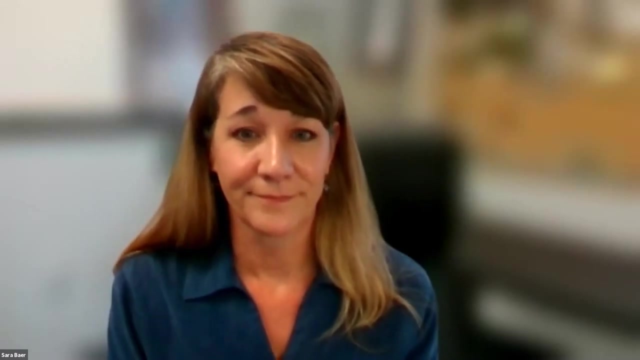 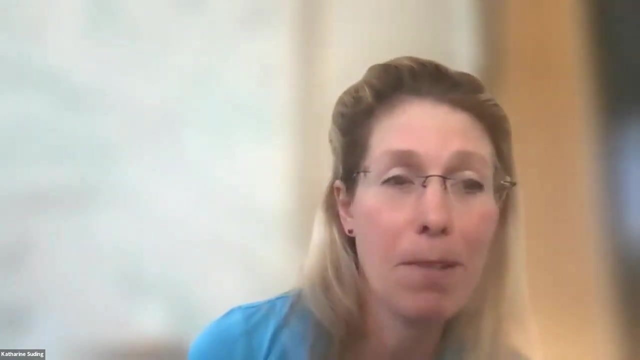 that's. that's a great point. I'm glad it was made. There is, I think that from everyone's other comments I think it's absolutely probably shared by all panelists How we actually get there might be a good 10-year goal right. 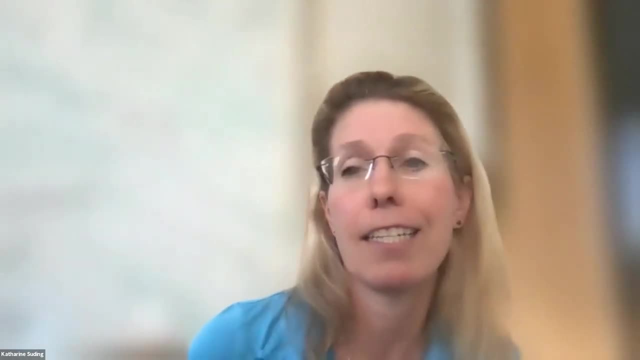 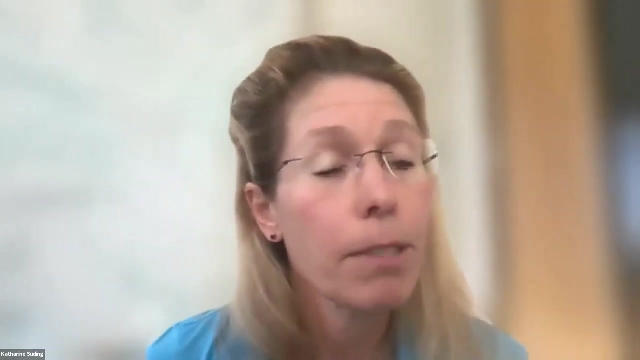 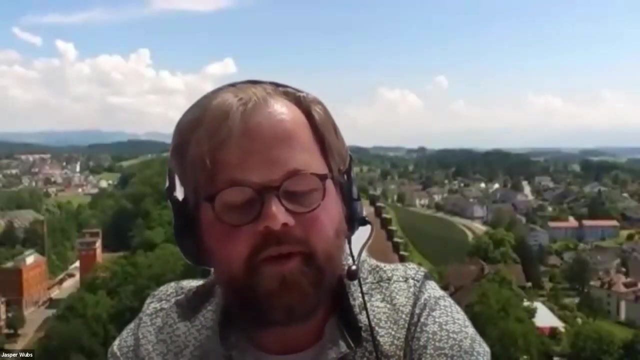 And so thinking about more of the system and really trying to take into account heterogeneity and complexity across different organisms. Jasper, Yeah, I think I agree with it in broad terms, but just to bring up another point, I mean a lot of research is focused on increasing diversity, increasing diversity in some microbes. 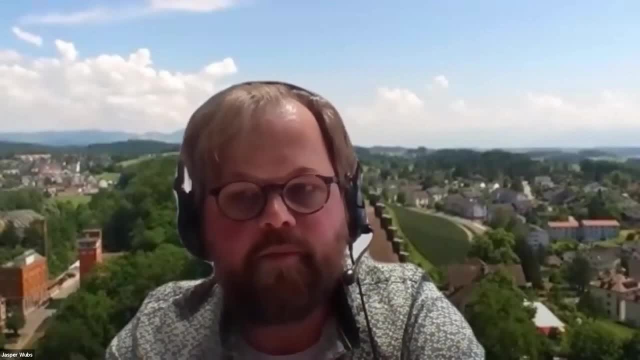 for instance, But I think we're also realizing that it's much more about composition rather than species diversity per se, And so I think, in general terms, it may be good to focus on complexity and to increase it, but you may be able to be much more effective if you know what components of biodiversity 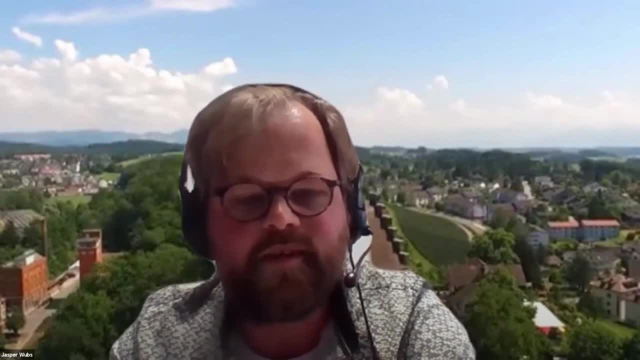 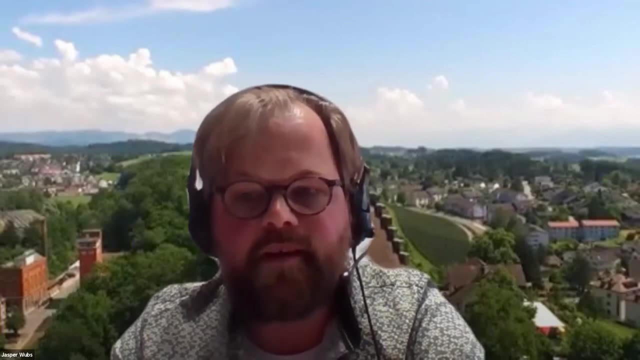 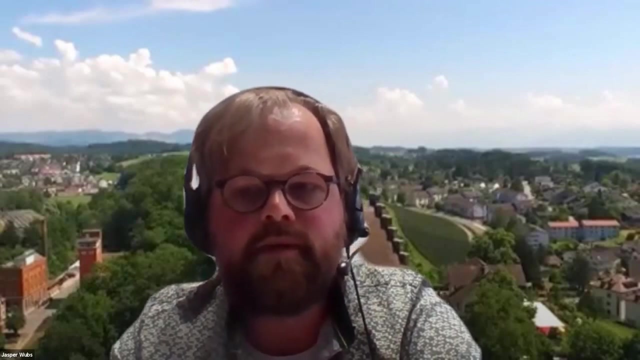 what you know? what AMF are you needing in that system? what faunal decomposures are effective there? rather than simply saying, okay, we just need more of everything. So I think we, you know, if we zoom in on that, I think we can do a better job. 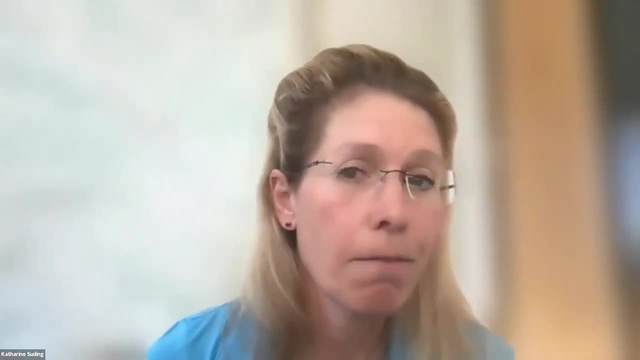 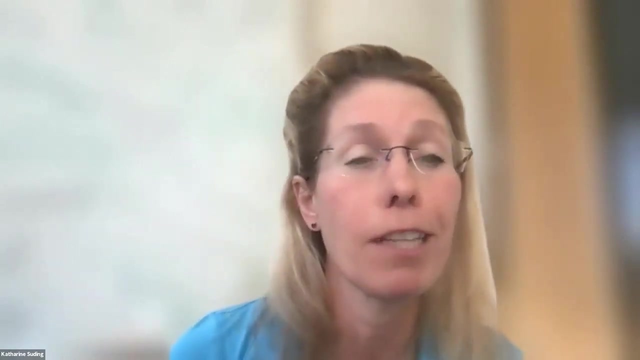 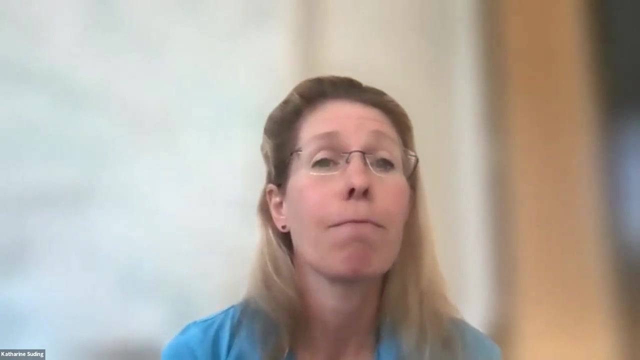 Excellent, yes, Getting a little a couple questions that are pushing us to think, maybe across systems a little bit. I'd like to address that a little bit. So do you think that these dynamics- let's talk about some of the systems that we haven't- 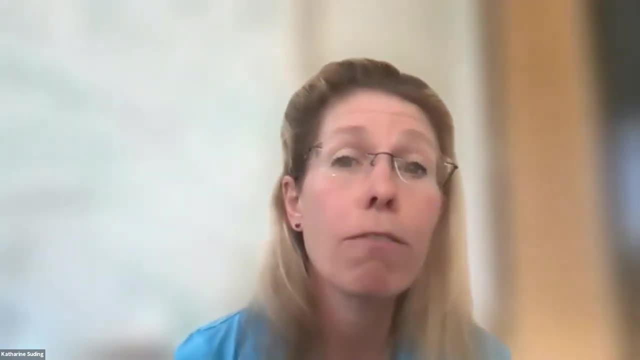 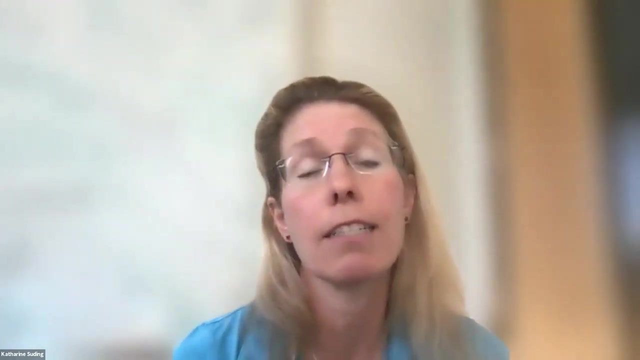 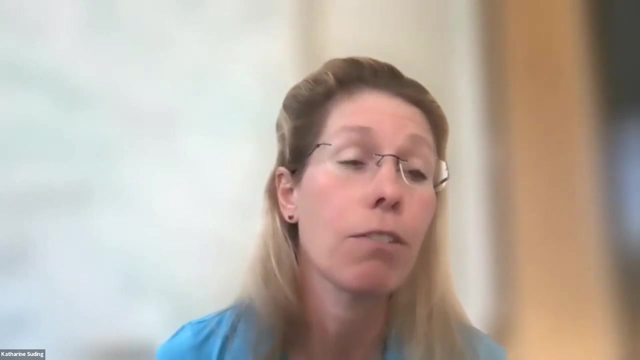 talked about before, So maybe a little bit more tropical forests or deserts or wetlands, like how much can we kind of think about these general processes across the board? Or are there some systems where soil biodiversity is critical for restoration and maybe some that maybe it's not as much of a key, key consideration, or you know anything kind. 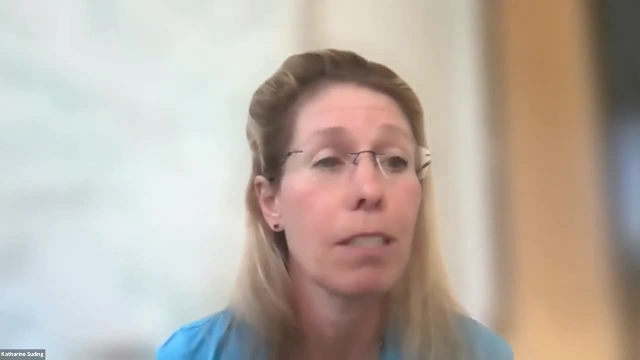 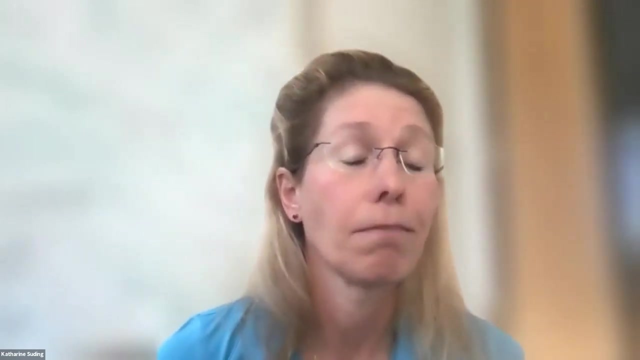 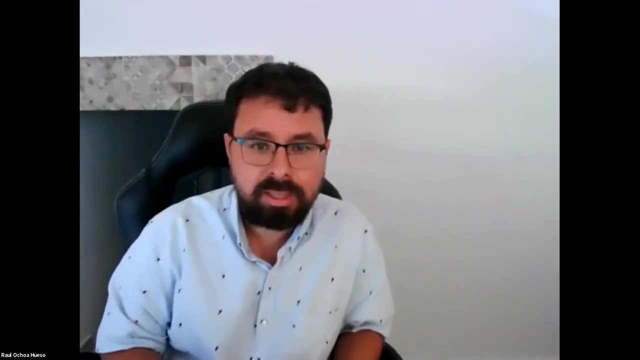 of at a, you know, at that kind of broad scale across some systems. Any thoughts? Raul, Yeah, I would say that as long as the immunity of the plants depend on soil microbes, that's always going to be a critical point. No, No. So maybe in wetlands we don't have the earthworms or other big animals- I mean soil animals- but still the plants are always going to need the microbes for their health, So they're always going to be critical. 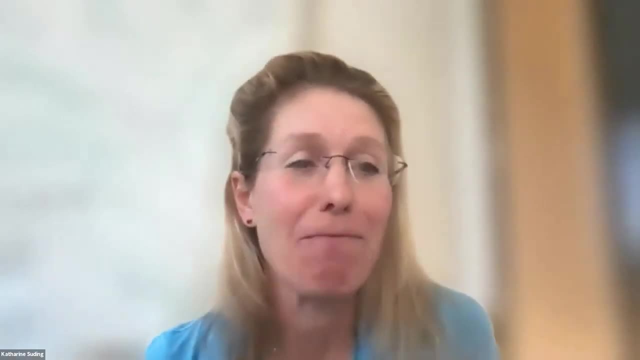 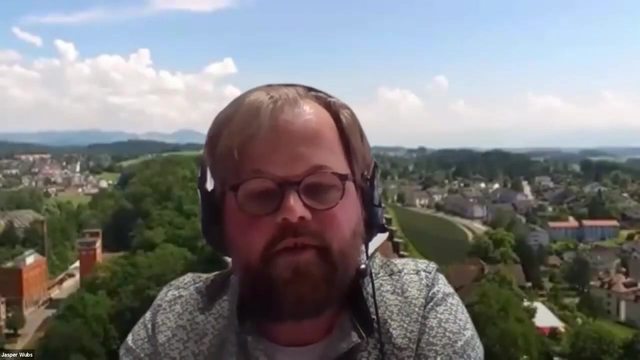 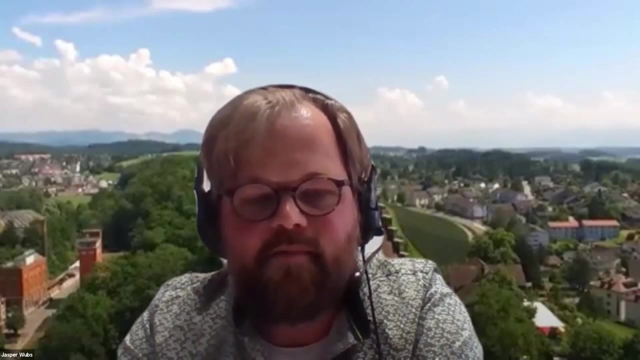 It's always important. I've always found it important. Yeah, I agree. I mean, at some level it is important. You need the microbes to cycle the nutrients. I guess if you keep, you know if they are not there that will not happen. 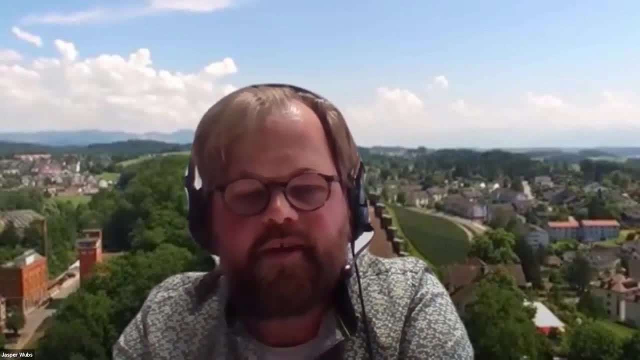 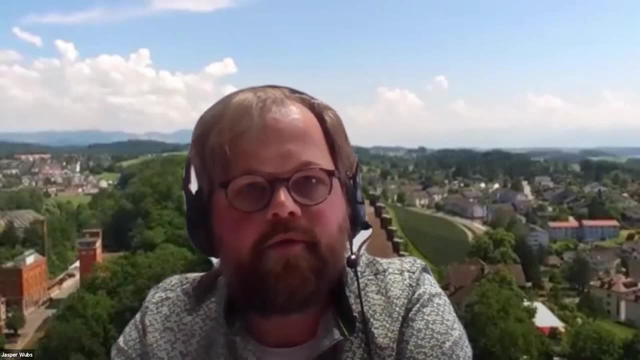 But again, I think you know it's specific components of biodiversity that you need for more detailed things, And it's interesting to think about this: how in the different tropical to peatland systems in the tundra would differ in this. 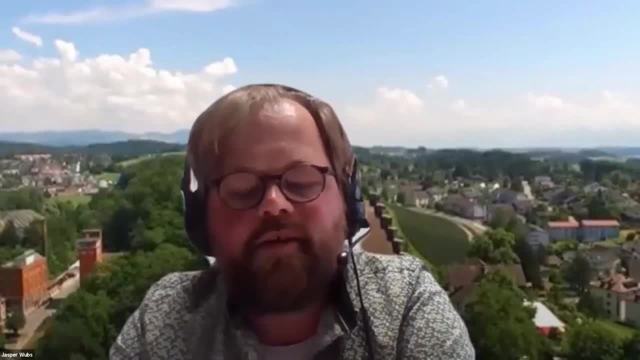 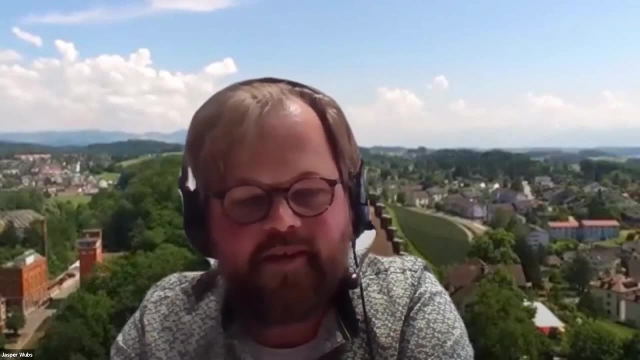 I don't really know if you, if, for instance, inoculation would generally be more important to do in tropical forests or in peatlands or in temperate grasslands. I mean, obviously there's a huge research gap in those tropical areas. 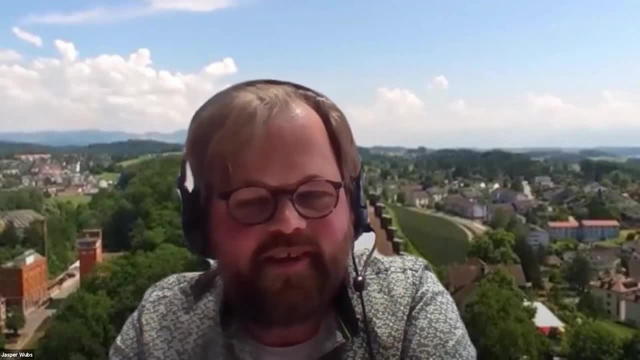 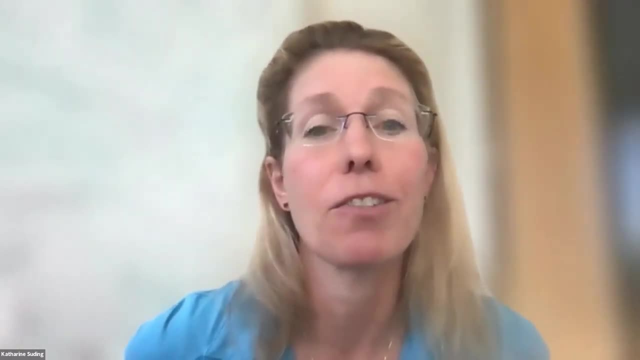 So I guess it's a shout out to doing more research there. I think it would be very helpful to have some of those kind of thoughts about just those general system dynamics and where and why in these different systems. So, Susanna, do you have any thoughts about that? 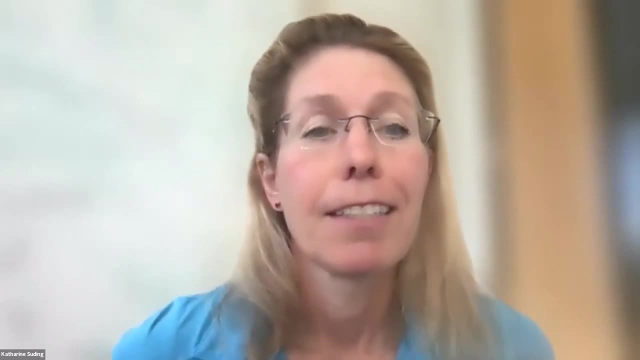 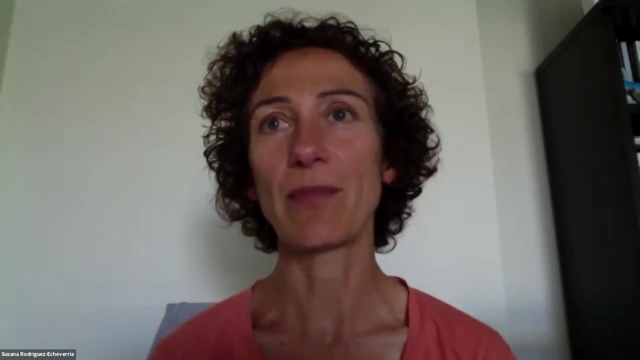 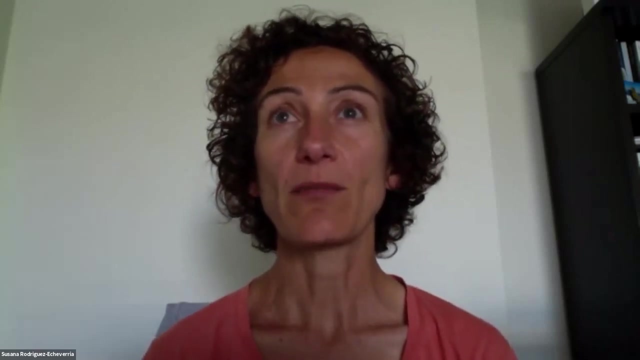 No, Well, of course I agree that it is important in all systems, but it is true that there is a big knowledge gap in many of these different ecosystems. There are some things done in tropical areas, more related to agricultural soils, for example. 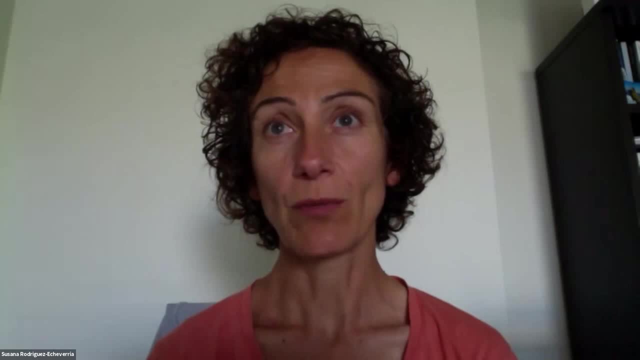 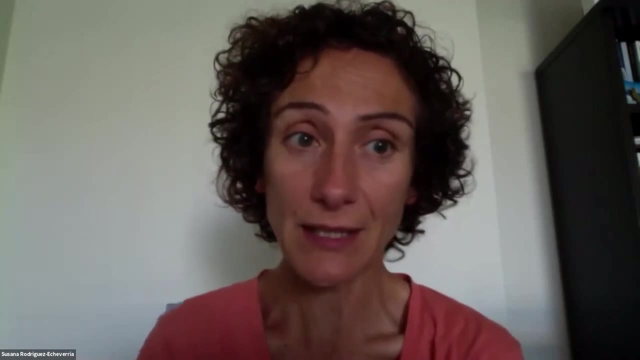 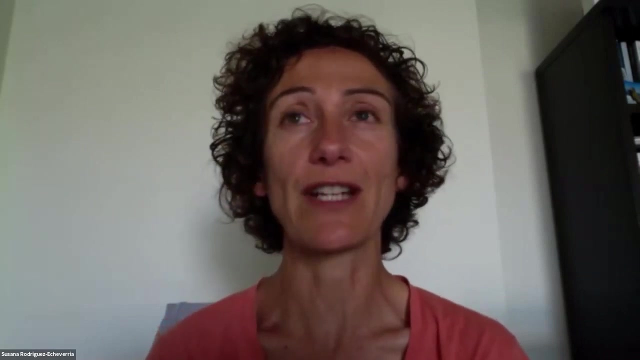 intercropping or to improve the composition of soil communities in terms of suppressing soil, And in many of these systems they are very complex, very rich in terms of soil microbes And I really wonder how they will behave with inoculations and soil inoculations. 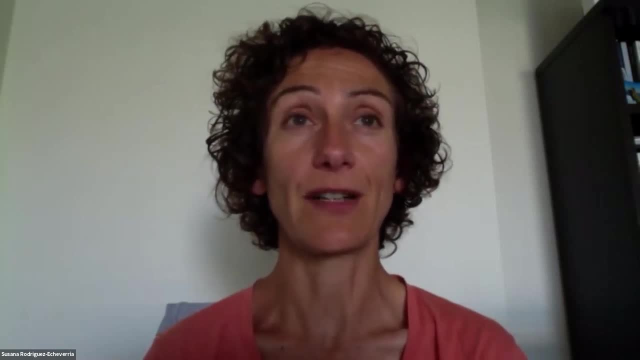 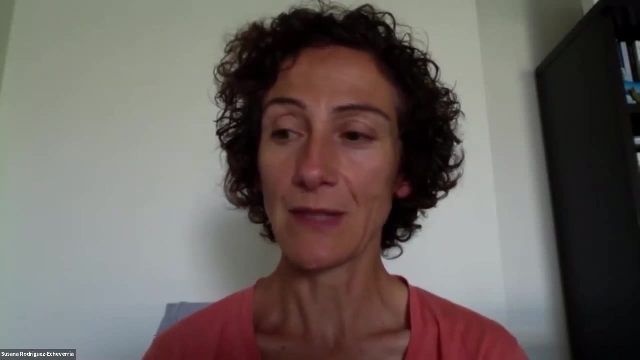 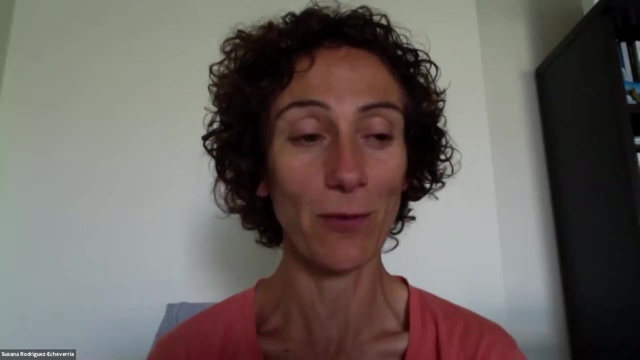 I think it would be very interesting to see how this would be applied in the future. I think it would be very interesting to see how this would be applied in the future. Thank you, Thank you. Thank you, Lidalh. Okay, thank you. 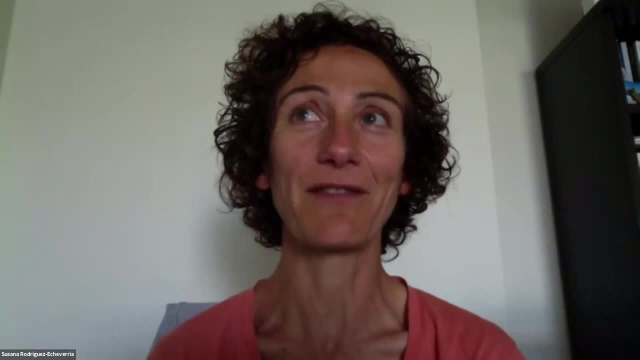 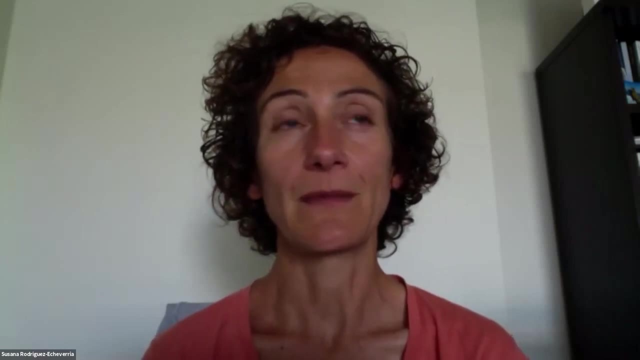 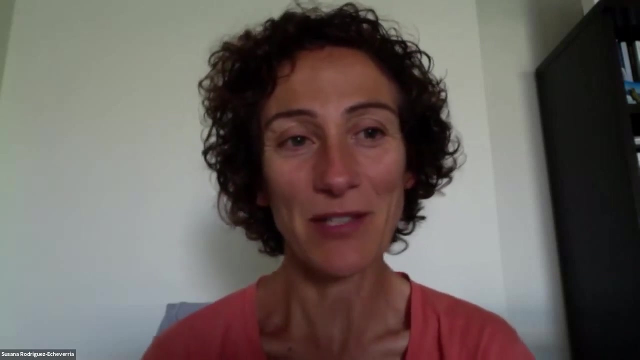 But we do not say just about the soil. We say, well, OK, if you made Serbia into a substrate, you can start having good soil production, if that will be mobile or is a very high- funky system that you cannot put anything different in there. 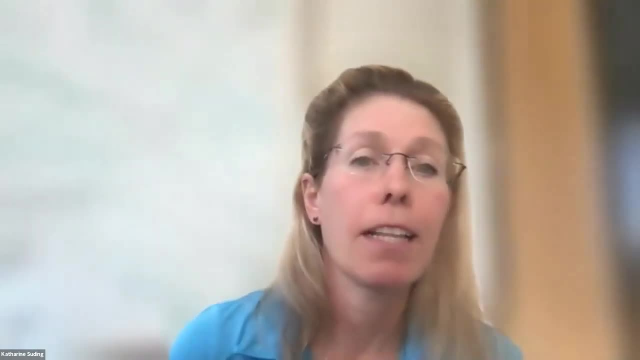 But yeah, I mean, you always have to take into account the soil, Otherwise plants are not going to be happy. Yes, it depends on the particularities of the system and knowing what is important there. Great, So we have about five minutes left. 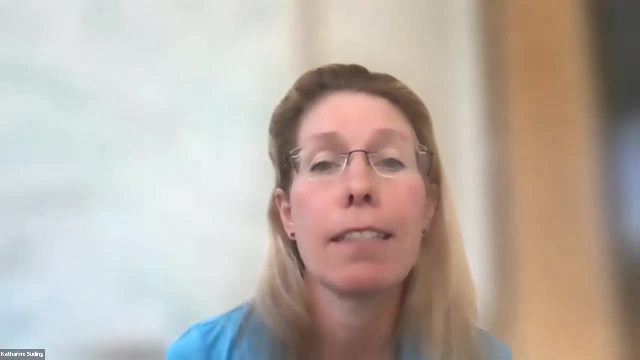 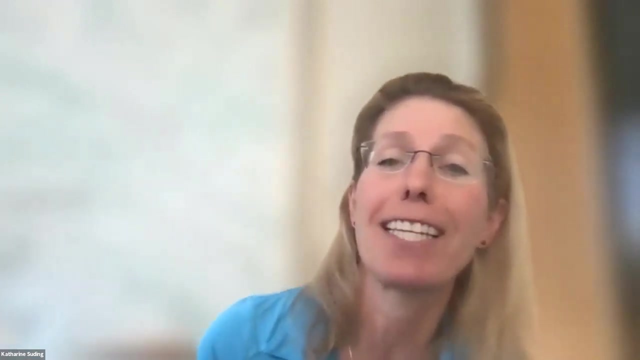 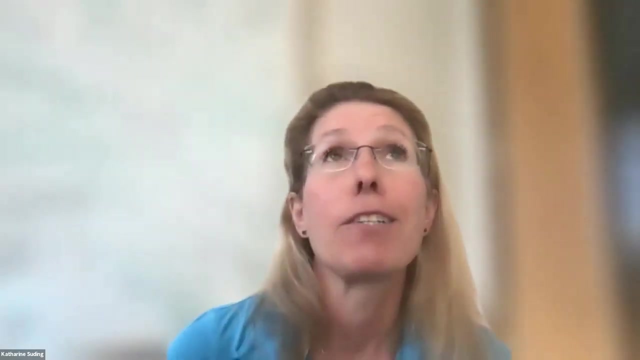 I just want to wrap it up a little bit, And you know we've talked about some really amazing things today, super exciting kind of new approaches and new ways of thinking and also some kind of frustrations or research gaps where we really want to move forward. So I'd like to end. 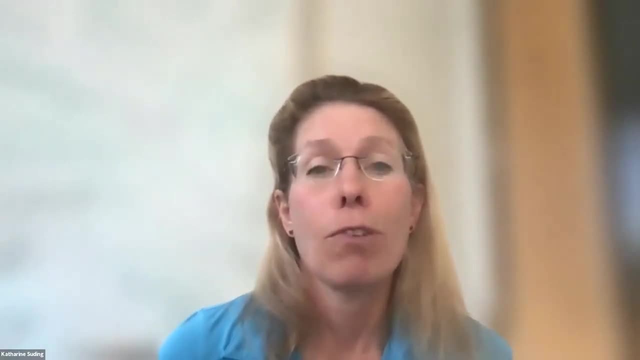 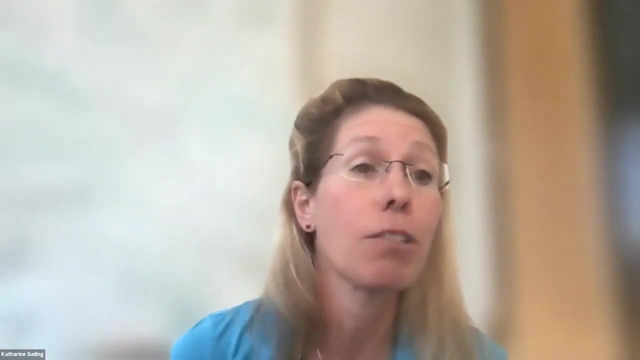 by asking you know what keeps you going and what really inspires you to be able to do this work, but also to transfer it to you know kind of change the mindset, whether it's land managers or policymakers or society as a whole. you know, in terms of transferring, you know these. 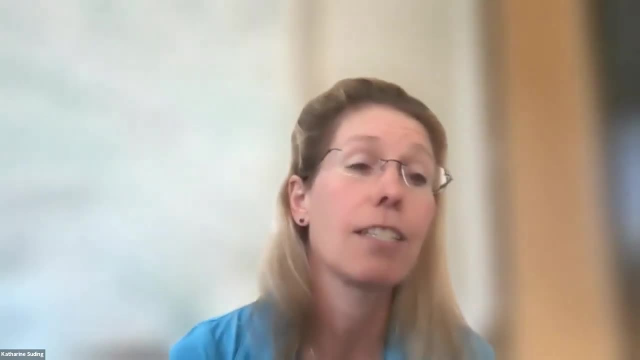 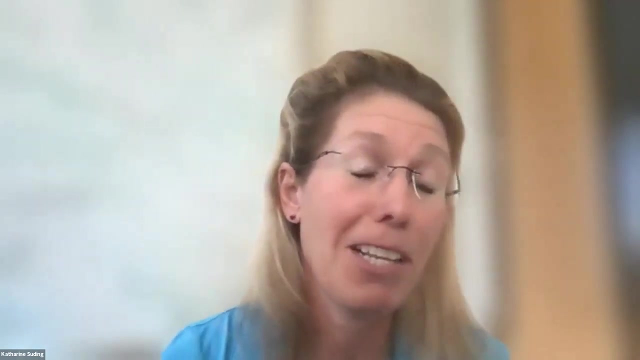 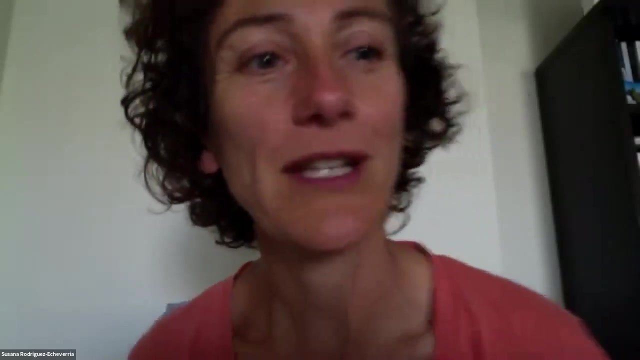 this kind of very exciting system but also really challenging issues to the greater good. I'd just like to hear kind of those end thoughts From all of you. Well, I can start if you want. As you say, doing research on soil can be very frustrating. 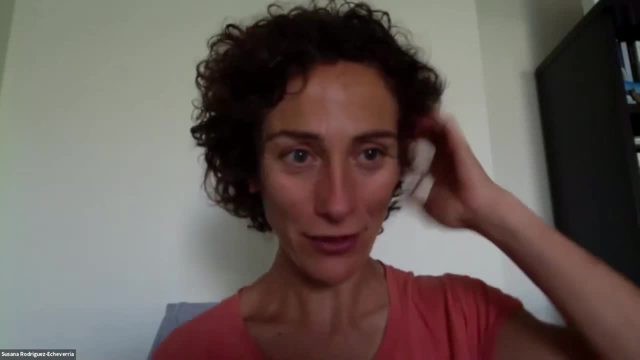 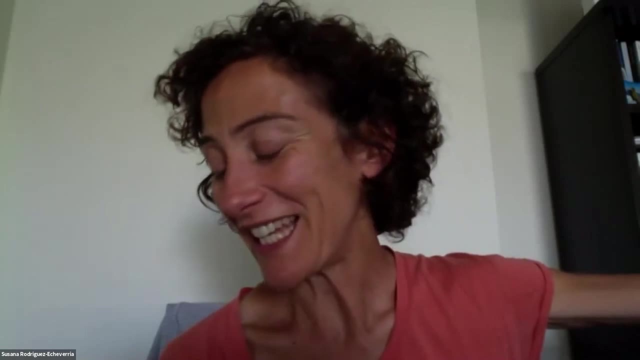 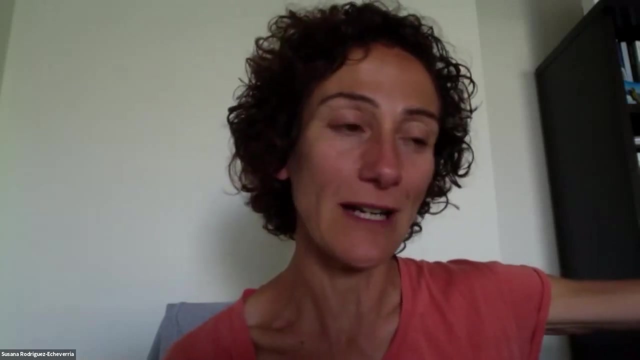 And sometimes I have thought many times to change subjects and study something that you can see more easily. But then, anytime that I do an experiment and see how important soil is, how different soils can change the whole result of the experiment, of this or the study, and then I 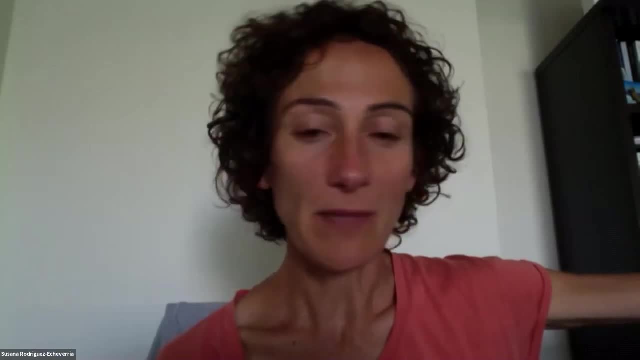 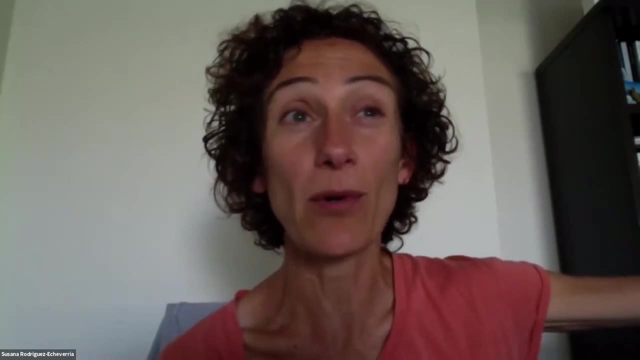 realized that is very relevant to pass the message, and so still, in many occasions, soil is used like a substrate, like a black box. that cannot be the future, because you cannot understand what is happening without understanding what is in the soil and what the soil is doing to the 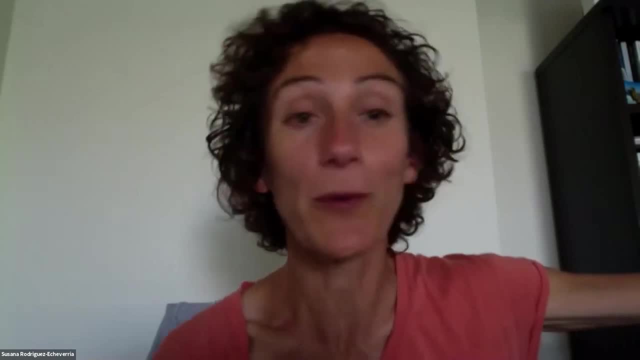 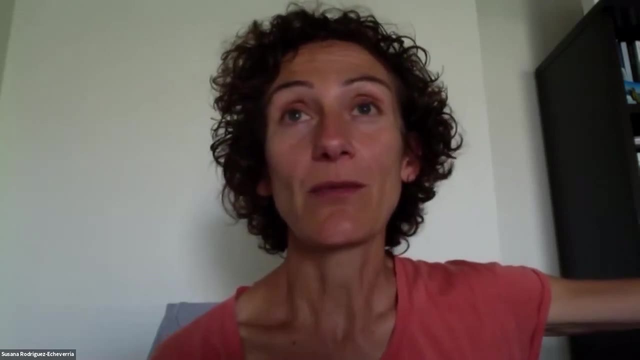 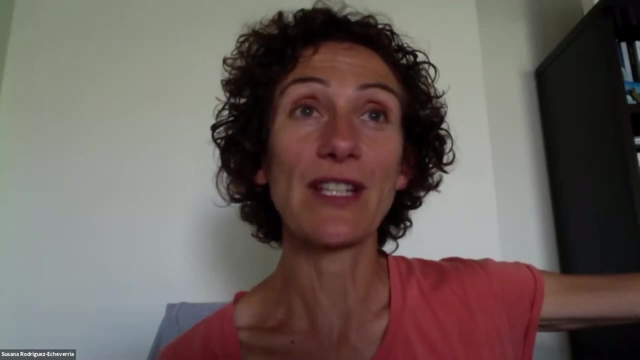 rest of the of the above ground organisms. I don't have much experience with managers or policy so I'm not sure how that can be addressed, but I'm very happy to see that are that there are big initiatives also at the European level to address this and to 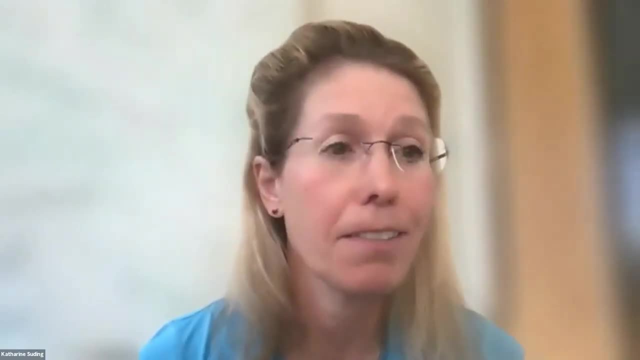 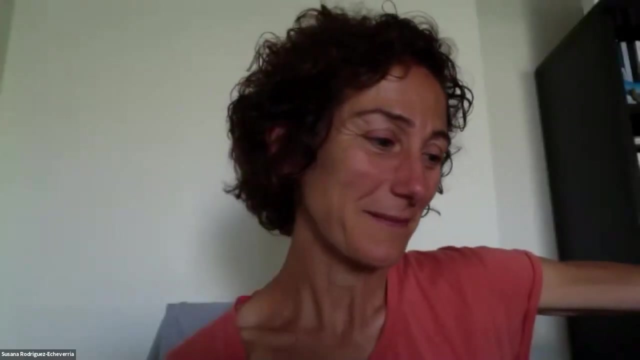 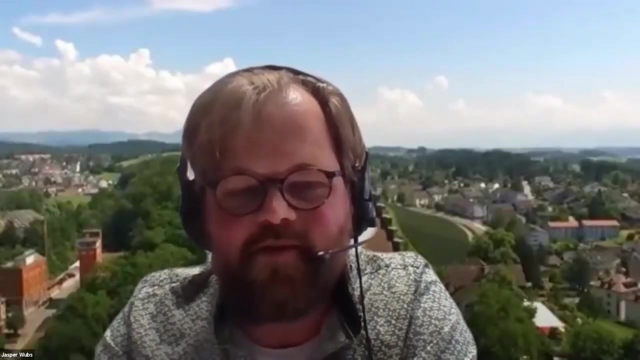 to get things in the right direction. Yes, there are. there are definitely some really exciting initiatives, Jasper. Yeah, I think I will echo Susanna's words. I mean, for me the inspiration is is mainly two things. one is is the complexity of the challenge. so soil biodiversity is complex. 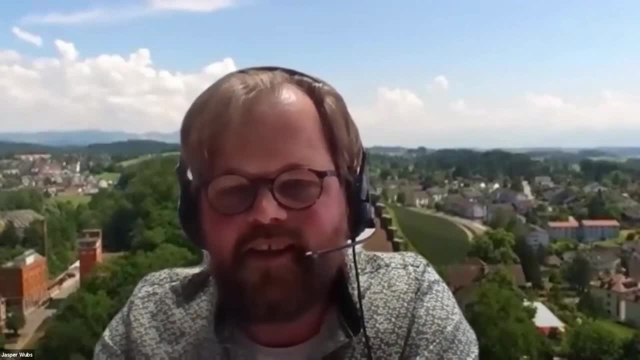 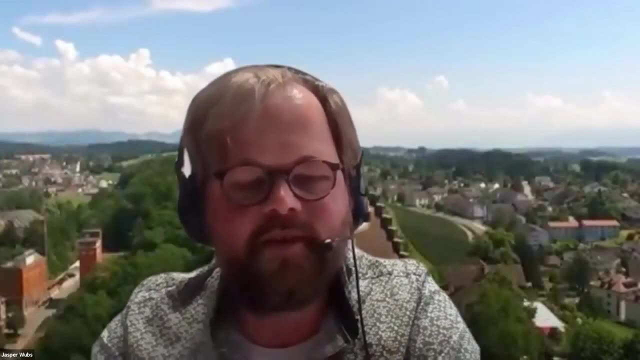 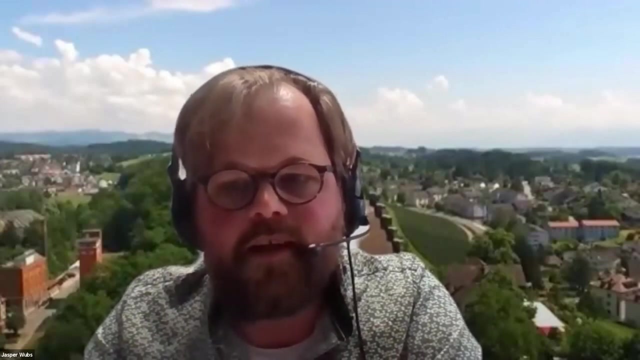 the interactions are complex. that also makes it a major intellectual challenge, which, which I think motivates me, you know, to try and untangle that and see what's the what influences what and why. and the other is the, the- the increasing attention that soil biodiversity is getting and the- the importance that we we have been increasingly able to show. 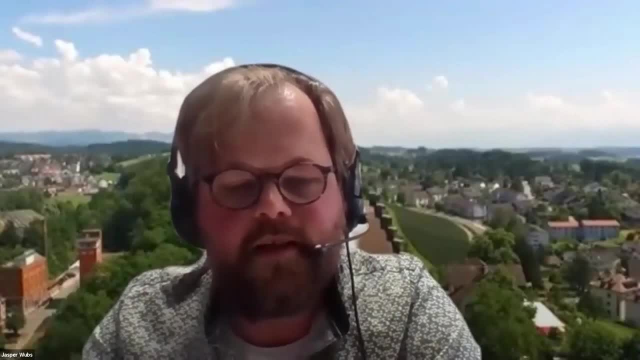 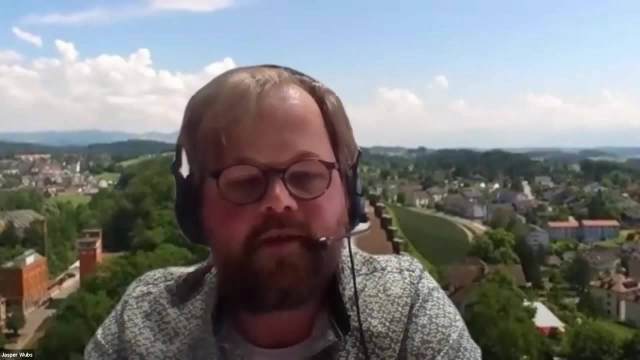 it has for soil functioning and and also restoration, and that that's now. you know that they're, that the public is very interested in this. the policy makers are very interested in this. I think that's very motivating. so there's a lot to do, but there's also a lot of people. 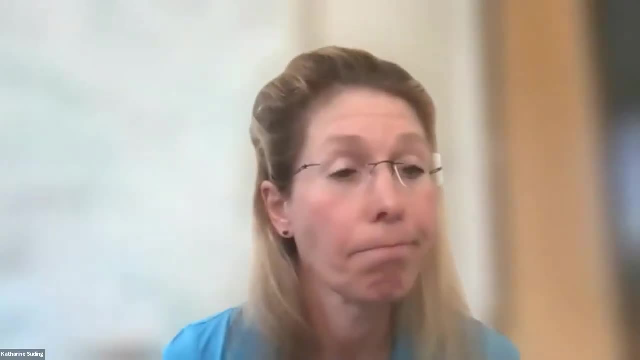 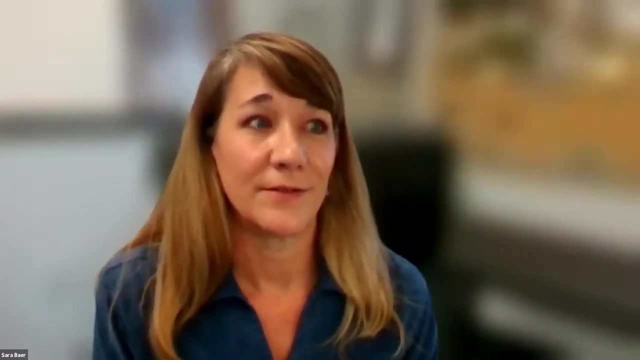 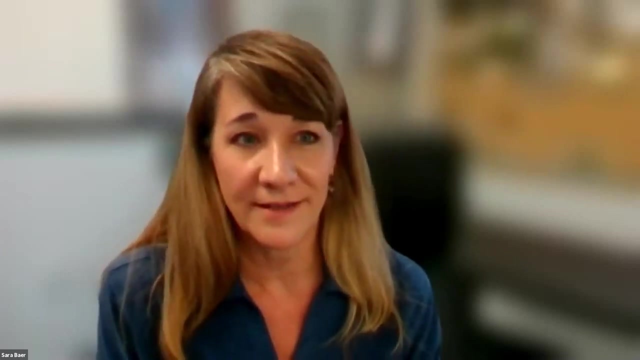 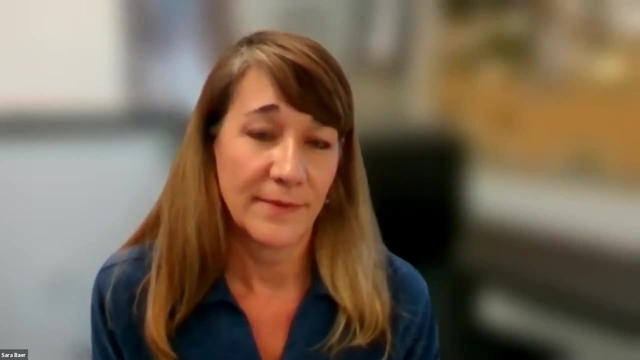 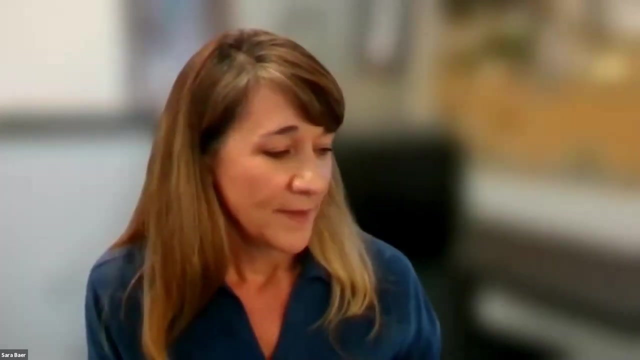 wanting us to do it, Sarah. So so I think there are two major um motivating reasons for for my research and what I do, and and one and and how it began um was that I wanted to help inform practice so that restoration practices are are more effective and informed. um the second thing that keeps me going. 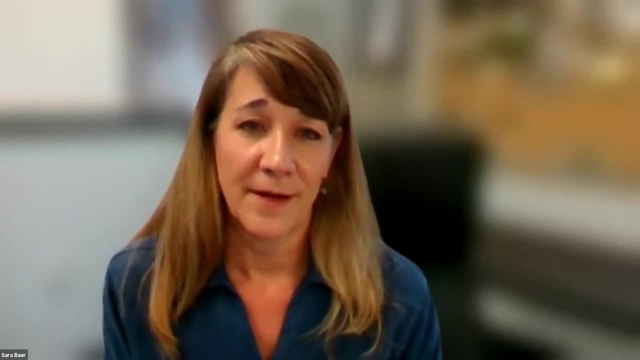 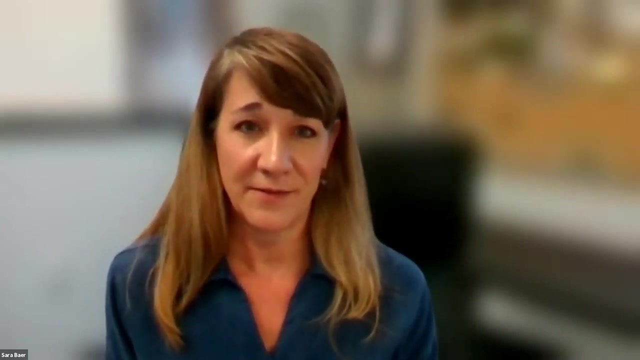 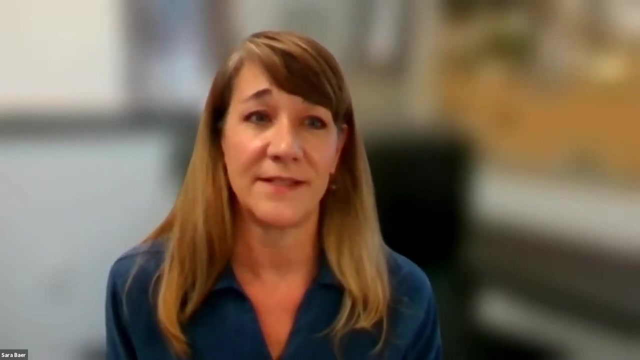 are? are the surprises? um, I mean, I I really enjoy working in soil where, again, you can't see what's happening, but you collect according to a design within a system and you are seeing these patterns over time and the data that you can't see. you can't walk out onto the land and see. 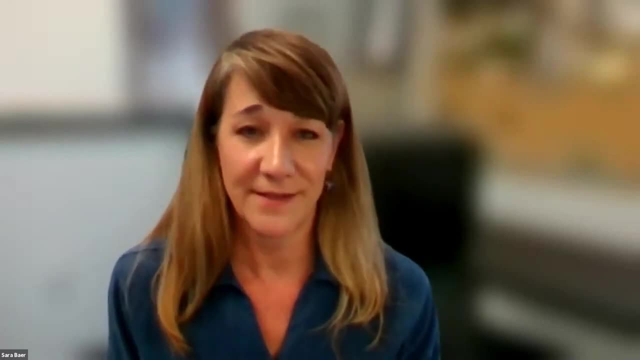 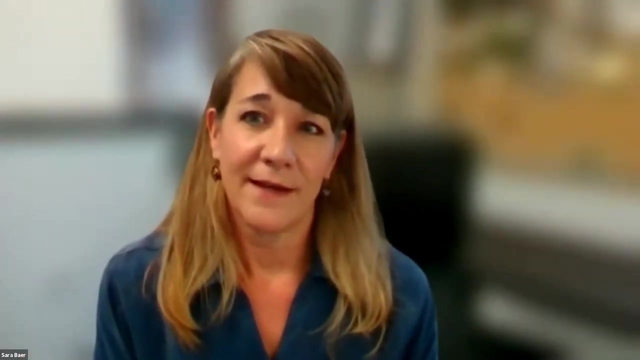 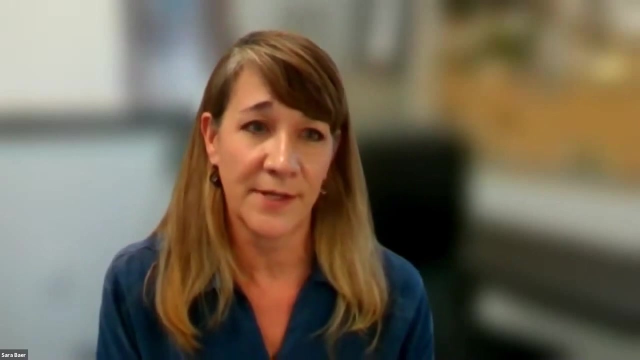 the phospholipid fatty acid biomarkers. you can't, you know you can't. well, you can kind of see the structure if you get in there. um, and then, and then the surprises from ecosystem comparisons. right, when we compared the sandy and clay soil, I didn't expect nothing to be happening in those. 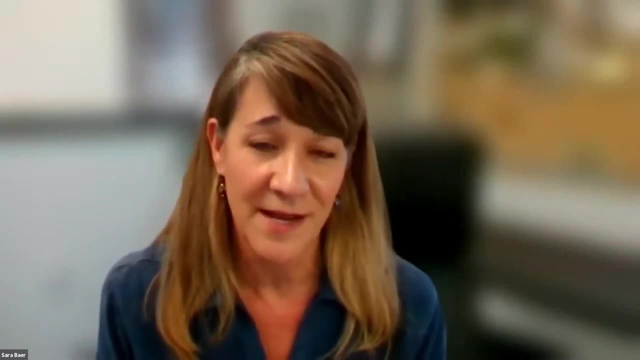 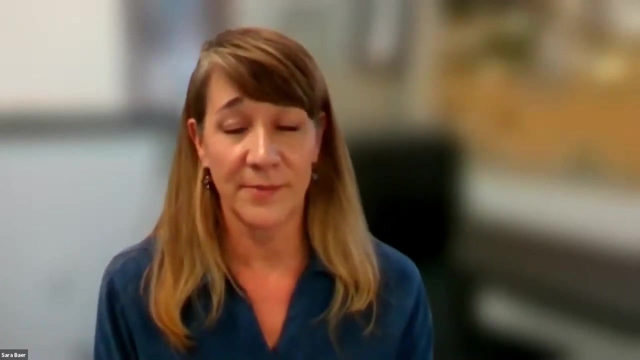 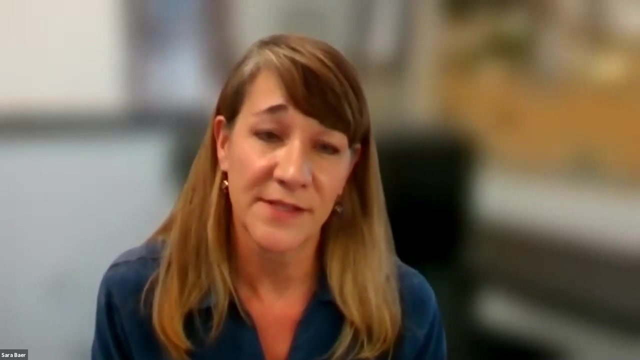 sandy soils. they had just as much above ground net primary production. the plants were there, the roots were there, right, and so that was a huge surprise. and then there is, there is an important me message for land use and policy, and that is: some systems maybe deserve a little more. 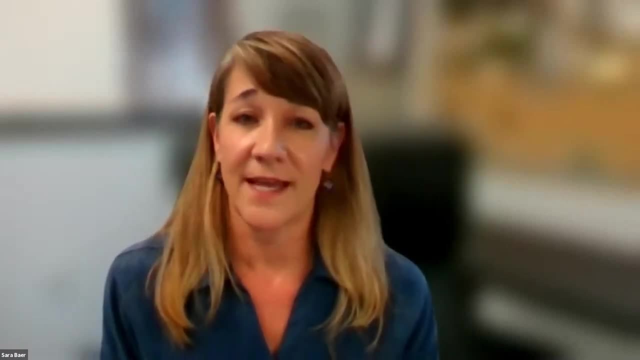 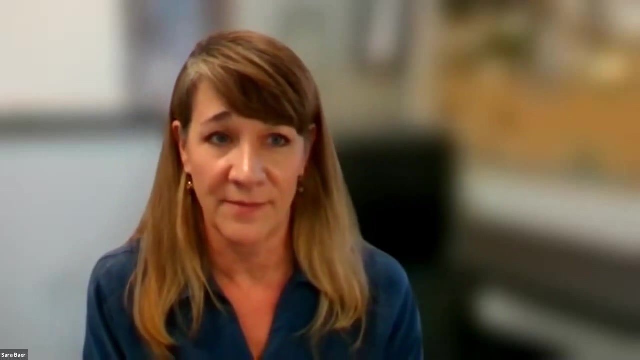 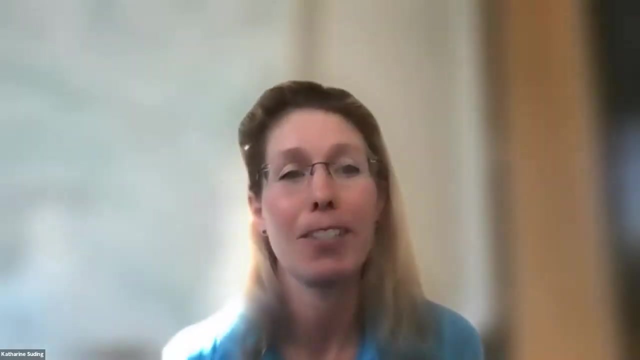 protection than others, if, if they are, if they can't recover, um, you know, using restoration practices, even with and within the time frame of of programs and incentives to to help. that's awesome. yes, I totally agree. um, the other thing is it just seems like stakeholders and 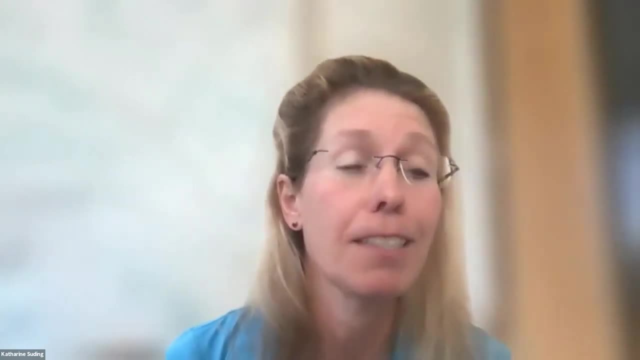 people that work the land really appreciate the soils too, right, and so they um. so it's, it is a common currency that you really- people really um- know. if they're um, they have a long-term relationship to particular parcel of land. how important the soils are, Raul, okay, yeah, I align. 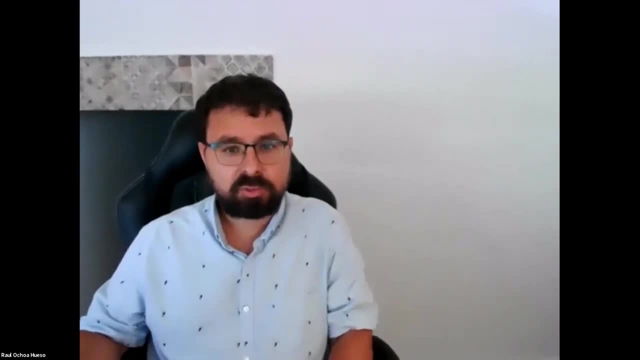 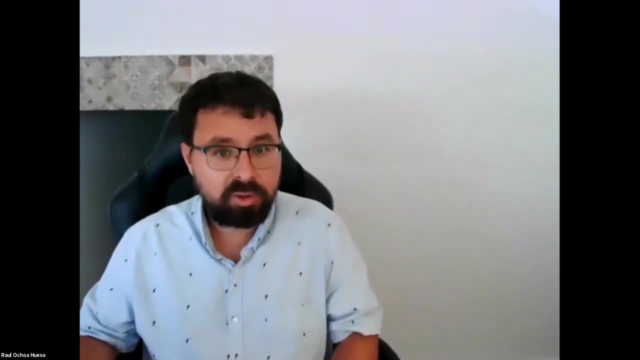 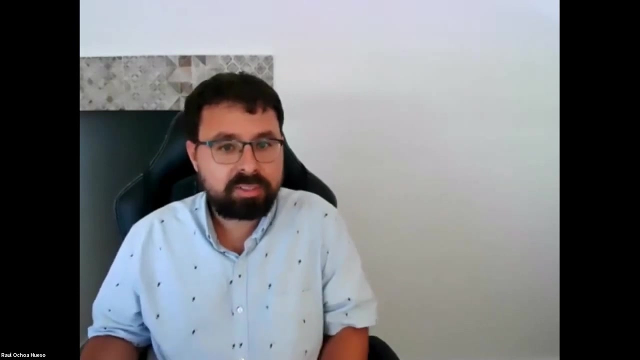 very much with Sara. I also have two main reasons. the first one would be to promote the well-being and the health of complex living systems like us and ecosystems, and the other one is simply to understand the world around me, and soils happen to play a critical role in it. so it's somehow circumstantial, but here I am. it couldn't be.